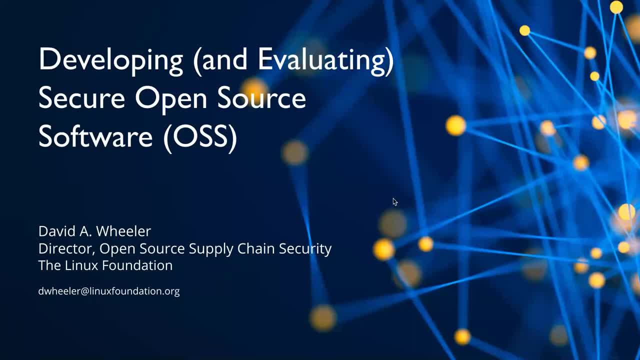 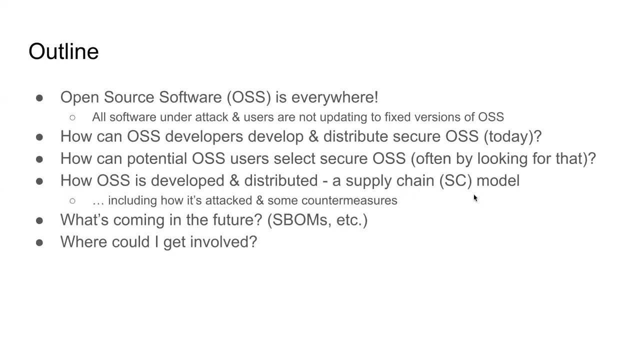 joining me today. so thank you very much for joining. i hope that you'll get a lot out of this presentation today, because i'm going to be talking about developing and also evaluating secure open source software. so very quickly, here's my outline. i'm just going to jump right into it. so quick. 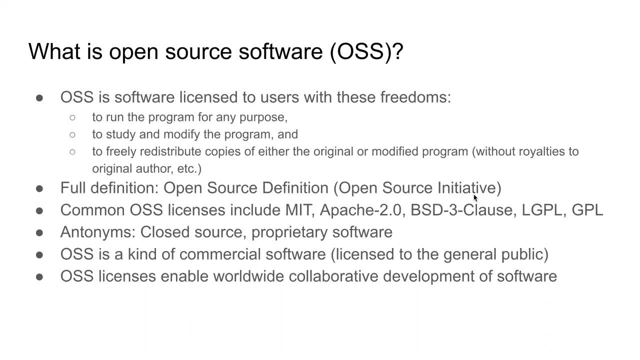 quick background because i found that some people don't know about some of these things. uh, first of all, i'm talking about open source software. what is open source software? well, that software license to users with certain freedoms, run it for any purpose, modify, study, freely distribute either the original or a modified version. there's a full definition in the open 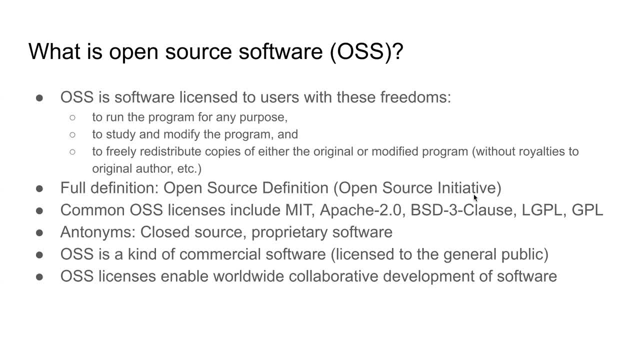 source definition and there's a lot of common licenses, like the mit, apache 20, lgpl, gpl. if you're talking about software and it's not open source software, typically it's called closed source or proprietary software. um, although it's not as focused, it's not the focus of this talk- it's important to understand. 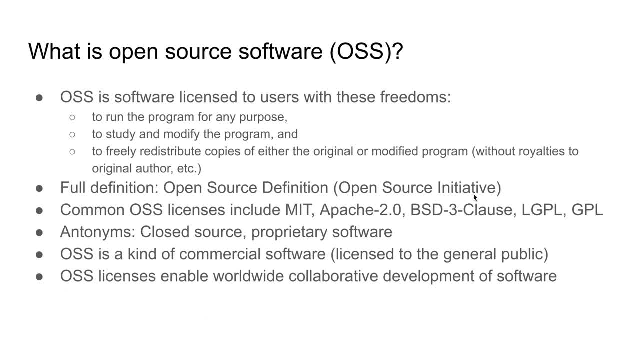 that open source software, at least under us law, is a kind of commercial software. it's licensed to the general public and automatically that makes it commercial software and that's actually pretty important if you ever have to interact with some organizations like the us government. open source software licenses, uh enable worldwide collaborative development of software and that 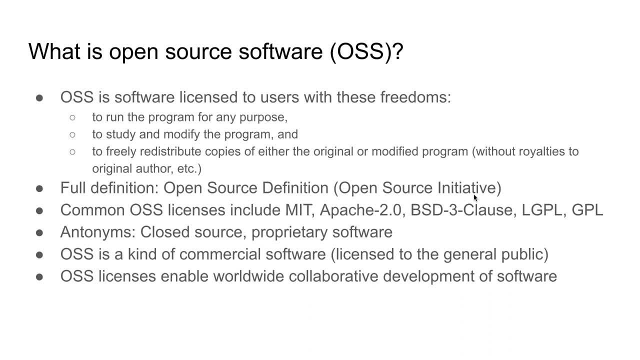 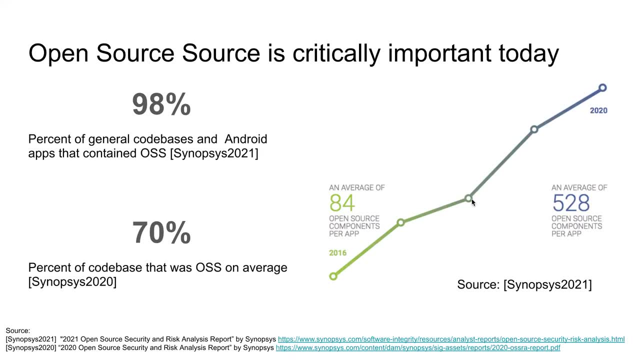 can have many positive benefits, including, uh positive benefits for people with disabilities or for security. open source software is critically important today. here's some figures. you know: almost all 98 of code bases uh contain open source software. uh, when synopsis looked into programs, they found that even if the software as a whole was proprietary, when you average things out, 70 of code bases were 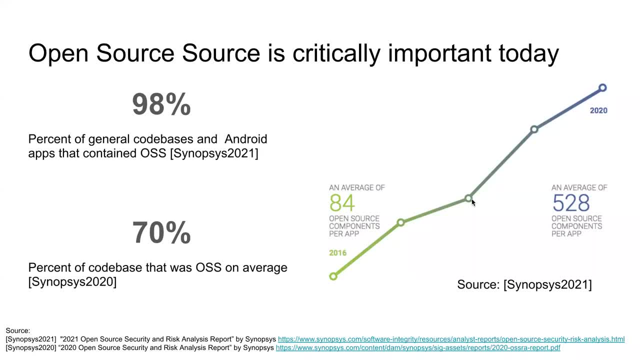 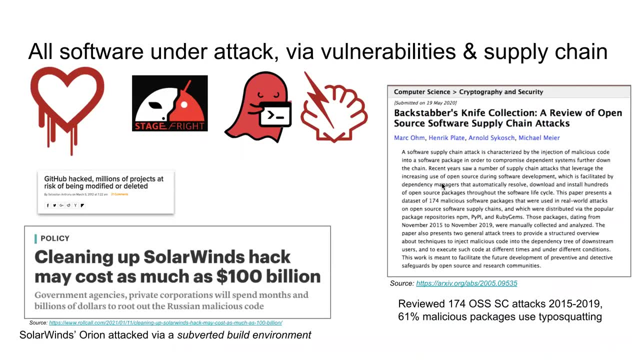 internally open source and there's more and more and more open source components within applications, and that growth continues now. so i've talked about open source offer. now let me talk about security. the reality today is that all software is under attack- open source, closed source, doesn't matter. 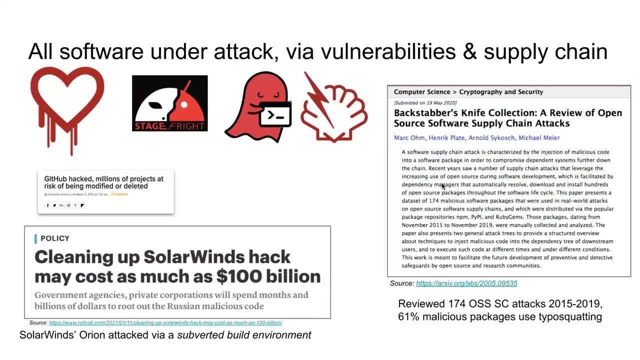 they're all under attack, and here's just some of the many, many examples, uh, that i hope. i hope i don't have to strongly prove this, uh, in this context, but just you know, it's not just open source, it's not just closed source, it's all software. it's under attack, both directly. 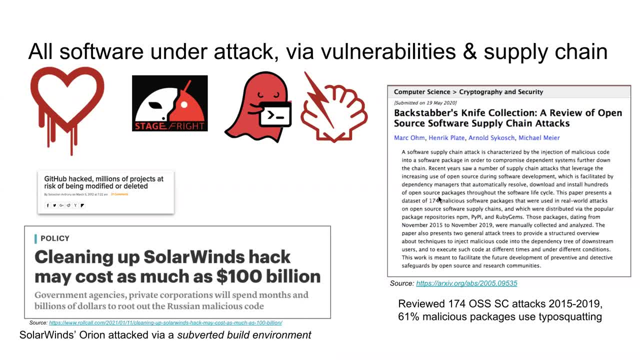 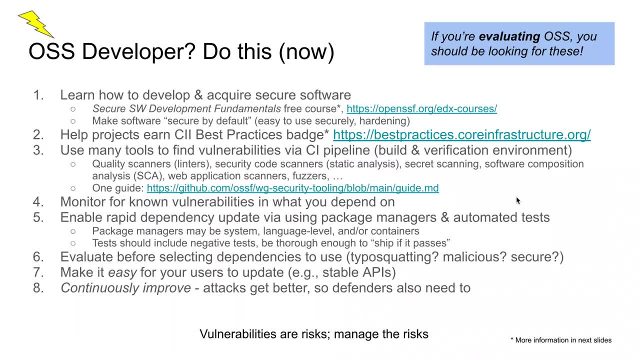 attackers trying to exploit these vulnerabilities, and the via supply chain attacks, where attackers try to subvert the process of getting the software to its eventual users. If you only can look at one slide today, here's your slide. Now I'm kind of hoping you'll see some other material. 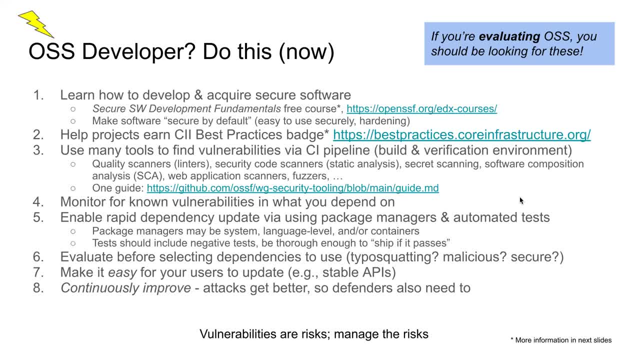 I'm gonna talk about. but if you are developing open source software, I'm hoping that you understand you need to make it secure as one of those important categories. Well, how do I do that? Well, here's kind of a top list of things. 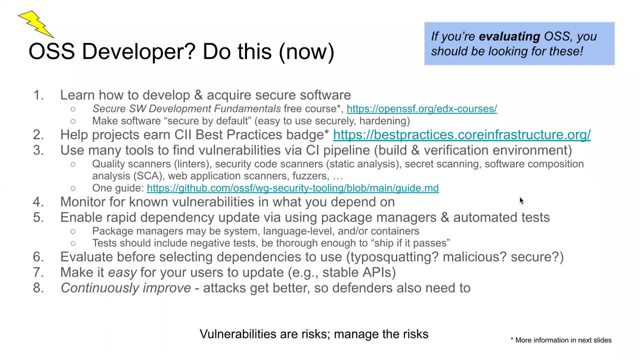 that you need to be doing. Number one and, in many ways, the most important: learn how to do it. The sad state of affairs today is that most colleges, most universities that teach how to develop software, don't teach how to develop secure software. 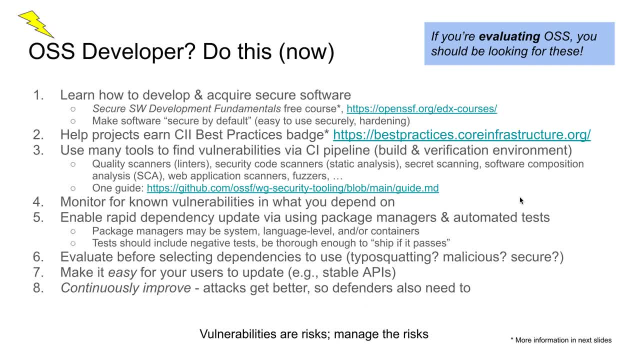 I think that's terrible, I think that's awful, but it is a reality. So if you don't already know how to do it, take a course learn. If you don't have that already easily available, please consider taking this. Secure Software Development Fundamentals. 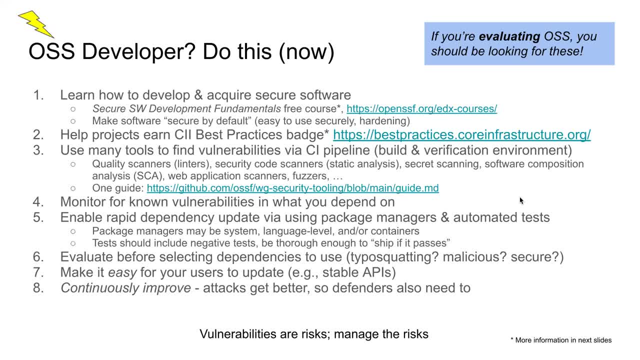 It's a free course. There's a URL right there. I'll show it again later. It's on edX. It costs you exactly $0, costs you nothing, and it will help you understand how to develop. I'll go over some basics of that. 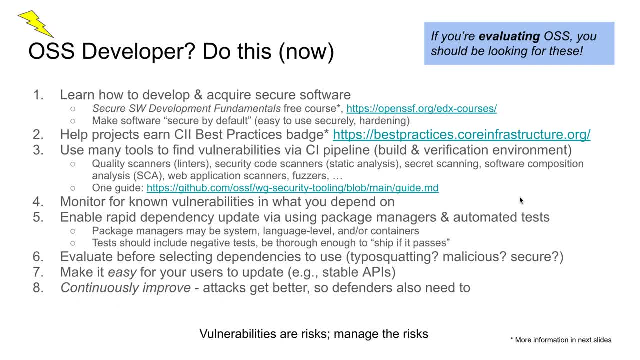 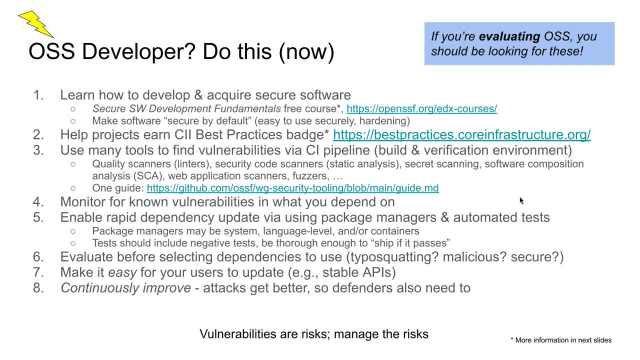 And, of course, it's more than learning. you gotta apply what you learn right. So make the secure that you develop secure by default. Make it easy to use securely. harden it against attacks. Make it so that when the user receives it, 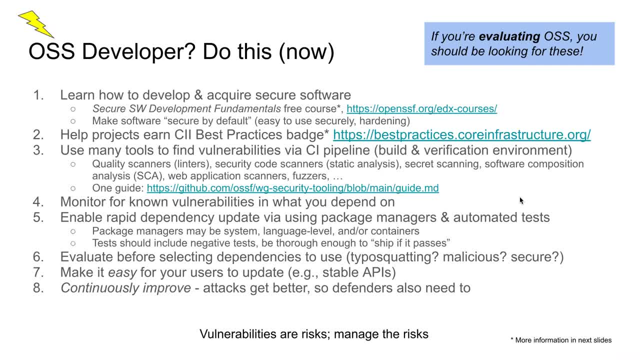 it's ready to go and to run securely. Number two: if you're developing open source software, work to earn a best CII best practices badge. There's another URL. I'll talk more about these in a moment, but basically it's a list of criteria. 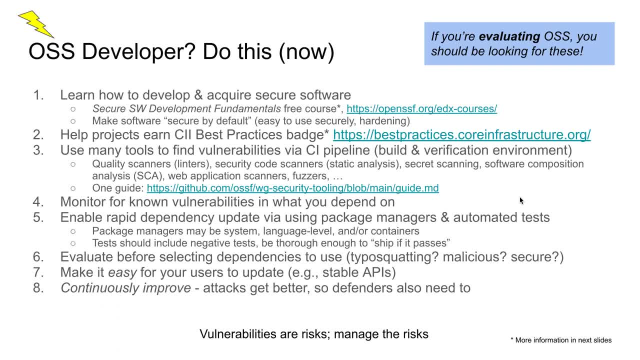 that, if you do, are going to increase the likelihood of producing secure software. Number three: use a lot of tools to find vulnerabilities in your continuous integration pipeline. There's a lot of different kinds of tools available. I've listed some common ones here. 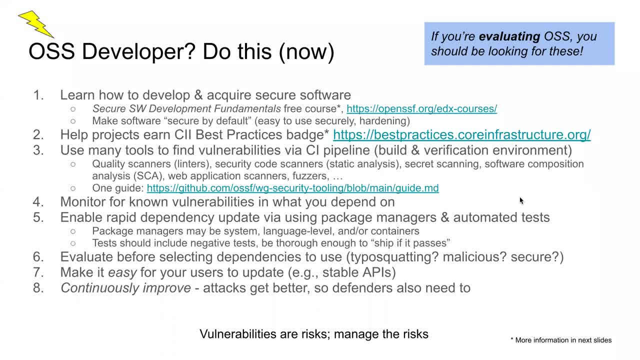 You know quality scanners, AKA linters. there's security code scanners. there's secret standing. there's software component analysis. there's web application scanners. there are fuzzers. You wanna use multiple different kinds of tools. You wanna use multiple tools. 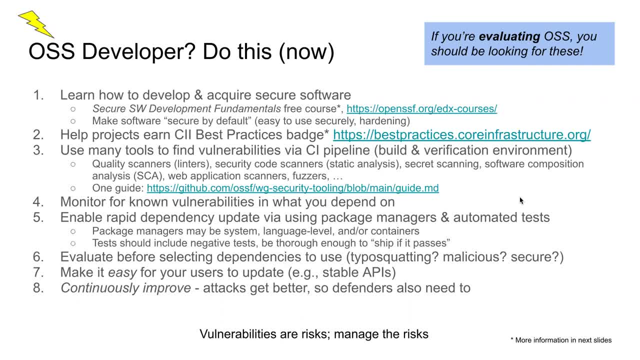 Tools just by themselves aren't enough to make software secure. You still have to know how to make secure software in particular, but they can be an important part of that of making secure software. Next, monitor for known vulnerabilities and what you depend on. 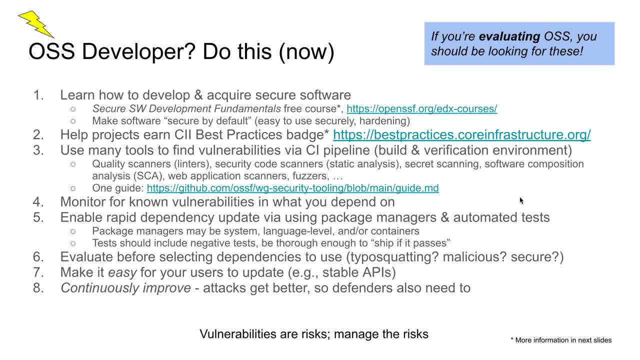 Nowadays most software brings in a lot of other software. If those dependencies have vulnerabilities, then that may become a vulnerability in the system that you've created using them. So you need to monitor them and update when they're vulnerable. which means number five: you need to enable rapid update of your dependencies. 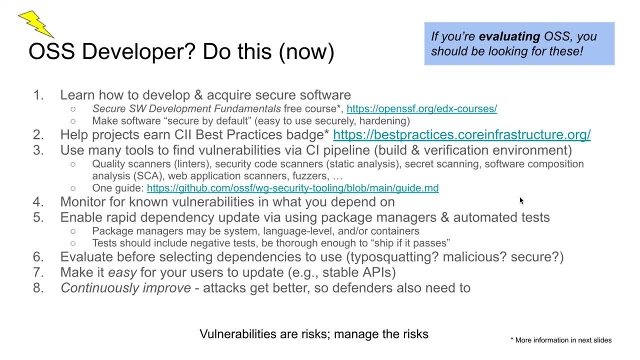 You know, once you find out that there is a known vulnerability, you need to be able to quickly update, quickly ship. How do you do that? Well, package managers and automated tests are keys to that, because package managers automate the process of managing your dependencies. 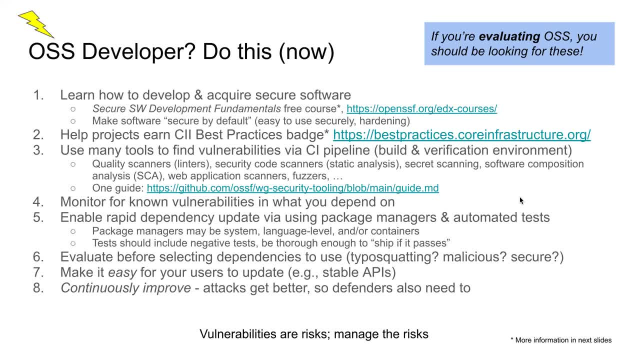 And there's different kinds, but you need to use them And your tests, your automated tests, should include native tests, tests to make sure that things that shouldn't work stay not working, and be thorough enough to ship if it passes. Some people ask you: well, how much do I need to test? 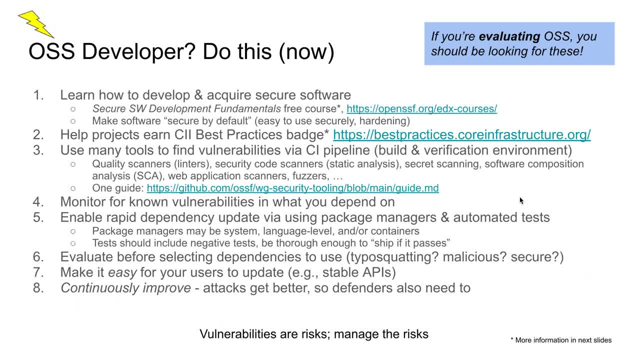 And the answer is: you make enough of an automated test suite so that if it passes your test suite it's ready to ship. If it's not there yet, then your automated test suite is not good enough yet. Number six: Evaluate before selecting dependencies. 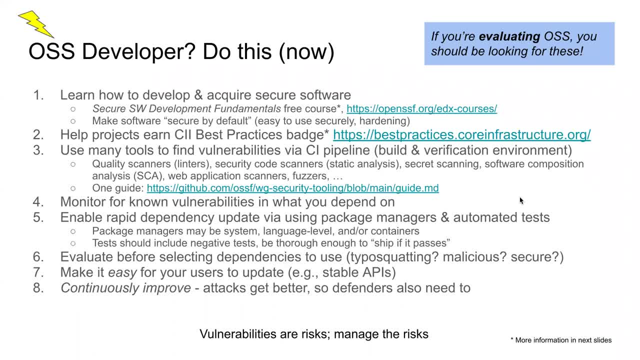 I guess in some sense that's out of order. but you basically, before you bring it to dependency, make sure you know, evaluate it, make sure you're bringing in the one you think you're bringing in. Make it easy for your users to update- things like providing stable API so that they can quickly update when there's a problem. 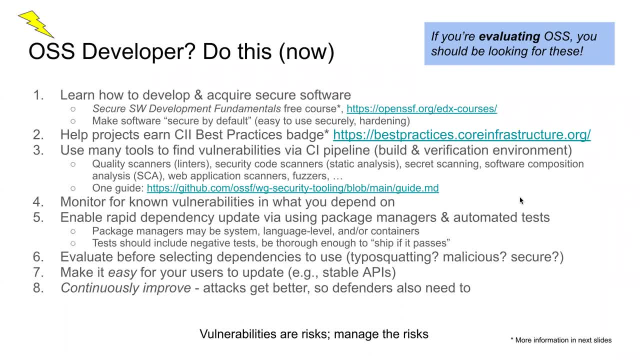 And finally, number eight: continuously update. Attacks get better, so defenders also need to get better. Now I don't want you to get the idea that Um Perfection is the one and only goal here. Vulnerabilities are risks. 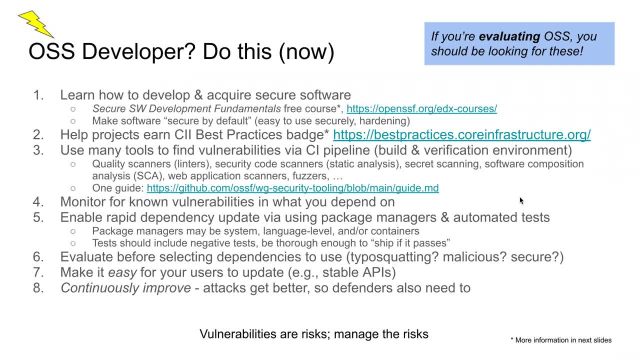 It's hard to eliminate all risks, but you can manage risks, You can mitigate them, You reduce the likelihood, You can reduce their impacts. Um, but you have to actually think about doing that. David, there is one question in the Q&A, if you want to. 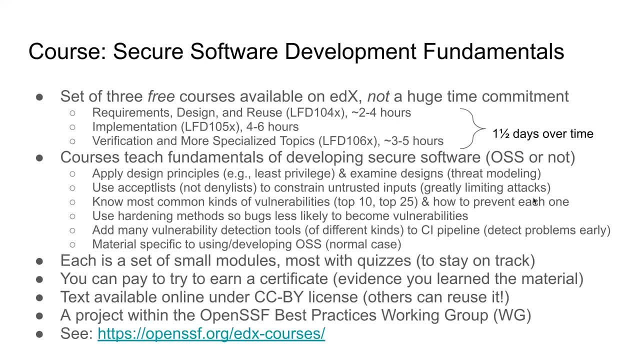 Um, yeah, we, um, I'm happy to take questions as we go. We probably need to, uh, we, it might be wise to have not too many, because we're After I'm done with my presentation. I'm hoping to have an open uh uh, you know uh, an open uh set of questions. but, yeah, let's uh, please do. 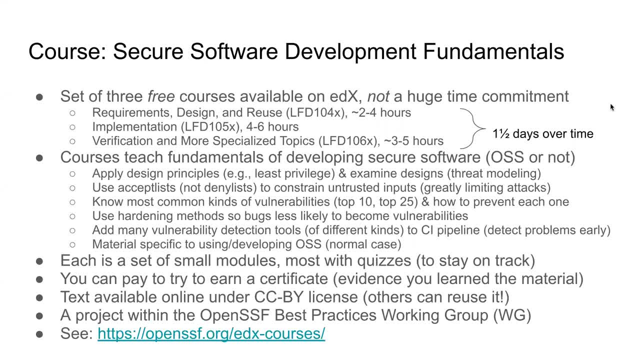 I want to answer questions. Uh, oh, I need to click on things. Let's see Where do I click. Uh, Q&A, All right. Uh, if I'm trying to select them open to add an application, how would the badges help me? 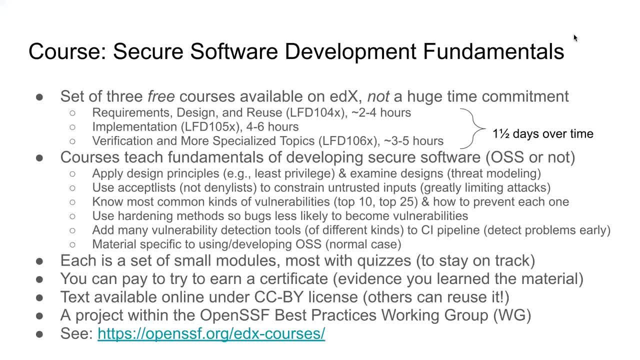 Um, let's see here. Uh, basically, the badges will give you an idea of whether or not those projects are working to develop secure software And you know where they stand. So, um, trying to achieve the best practices for your own project helps your project get secure. 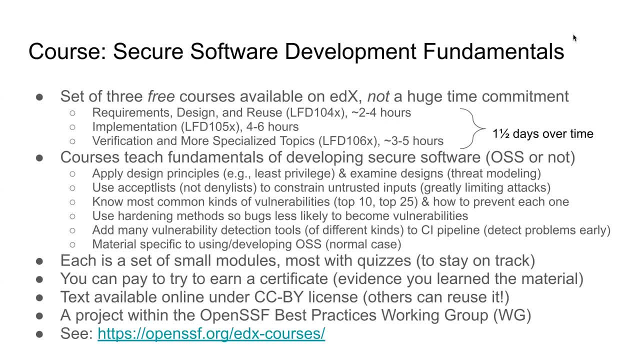 Looking for projects that have achieved those badges, or at least are well on the way to achieving them. uh, gives you confidence that the projects you're bringing in that you're, as your dependencies, are in fact more likely to be secure. All right. 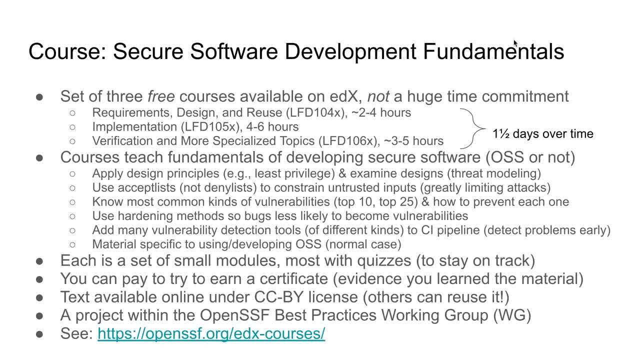 So let me talk a little bit about some of the things that I um. I gave him my summary slide. I talked about this course, about developing, Uh, about secure software development fundamentals. It's a set of three free courses. It's not a huge time commitment. 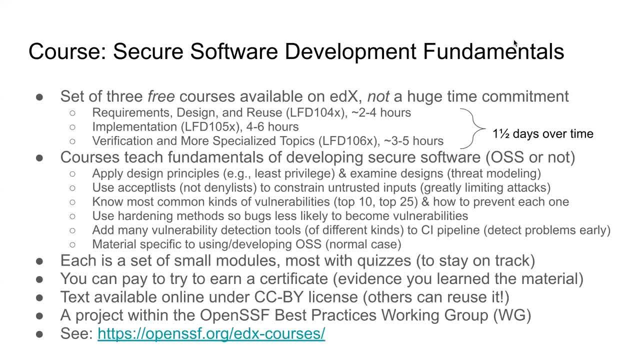 You've got approximate hours here. I mean, if you took an hour a day, you'd be done in less than two weeks. Um, and it covers these topics. Um, you know how to design. what are the design principles for security? 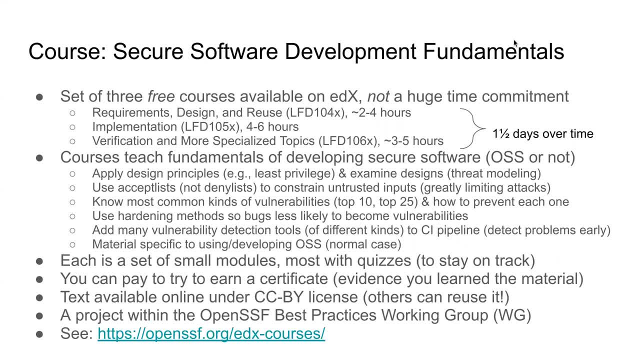 Things like least privilege and least privilege, how to apply those, uh, how to examine designs, how to use, use accept lists and not delight list to constrain untrust, Yeah. So if you're taking inputs from somebody you can't trust, you should be very, very strict on what you accept, define very strict patterns on these are the only input values allowed and just reject everything else. 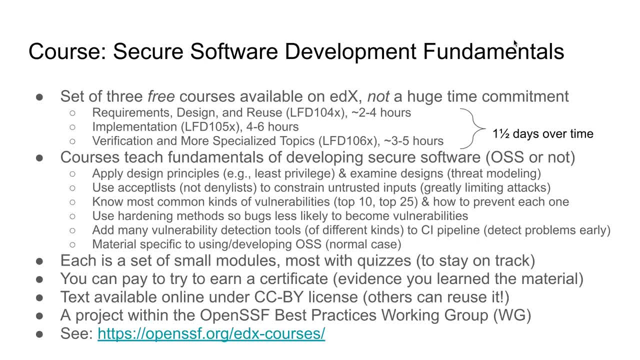 This is incredibly effective. effective on limiting a lot of attacks. know the most common kinds of vulnerabilities. You know there's various top 10 and top 25 lists- and then how to prevent each one. uh, use hardening by methods so that, yes, you're probably going to have some bugs in your code. 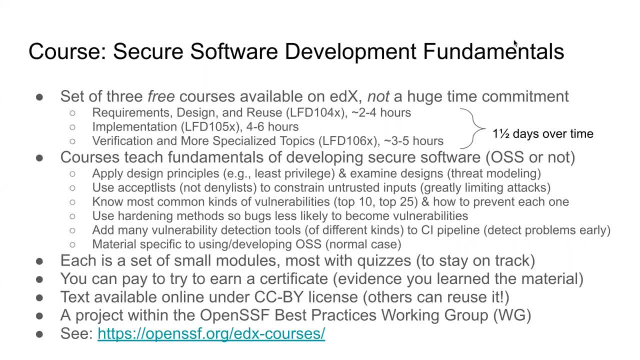 But not all bugs are equal. You can take a lot of steps to reduce the likelihood that a bug is a vulnerability. Uh, I already mentioned adding a lot of vulnerability detection tools to your CI pipeline. It talks in more detail what the different kinds of common tools are, the pluses there's, their strengths or weaknesses, how to apply them. 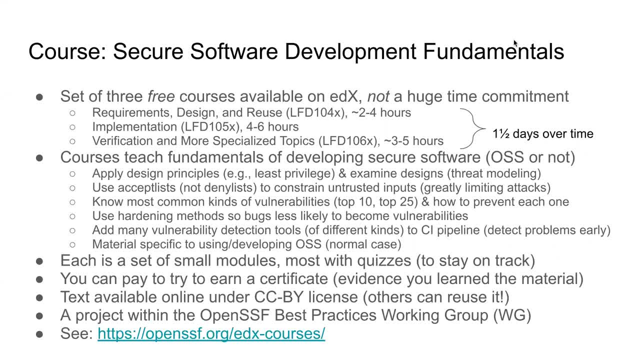 Um, and, of course, uh, in this course, unlike many, has materials, uh, specific to using a developing open source software. Uh, we've got some. some of you needs to put mute on, All right. Um, one nice thing about this little this course is not only is it free, but it has a large number of small modules, and almost all of them have a little quiz at the end. 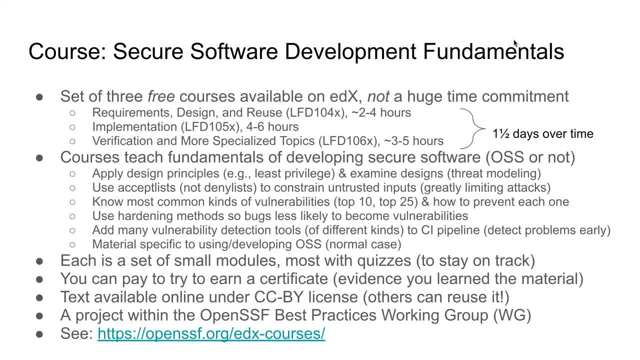 Uh, this is a very simple technique, but I found that it's really, really helpful to stay on track instead of just, you know, blindly reading- Oh wait, I got a little quiz. I got to answer my quiz And that really helps. you can pay to try to earn a certificate. 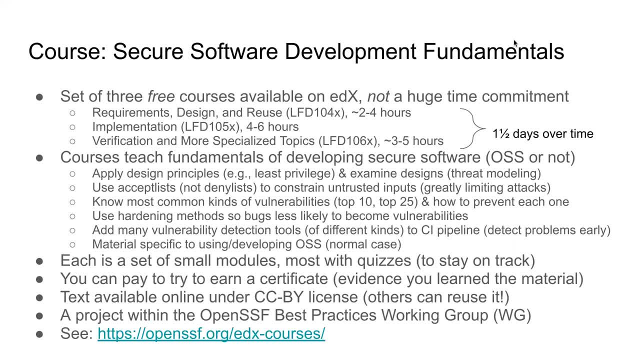 You don't have to, but, uh, some people want to be able to prove that they learn the material. Yeah, Yeah, And so we offer that as well. Um, by the way, this is a project within the open source security, uh foundations, best practices working group. 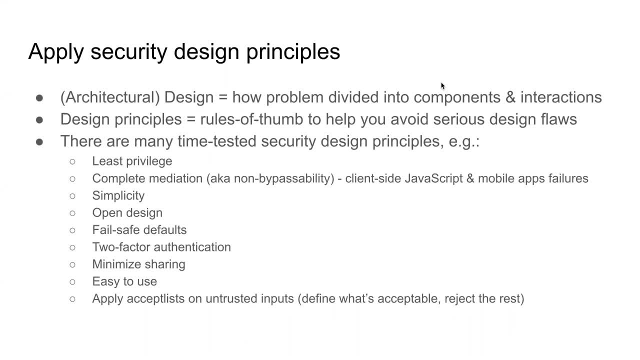 All right, Let me talk a little bit about some of those key points that are covered in much more detail in that course or other courses about developing secure software. So, uh, I've heard some people say that, Hey, my software doesn't have a design. 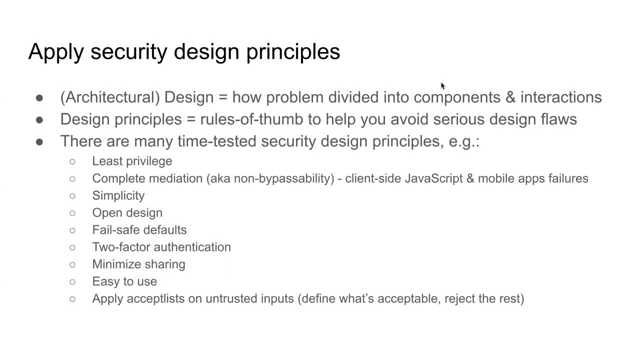 Well, your software might not have a documented design, but if it runs, it has a design, because the design is simple: How you divide your problem into components and how they interact. that's all. all it's meant by design. working software always has a design. 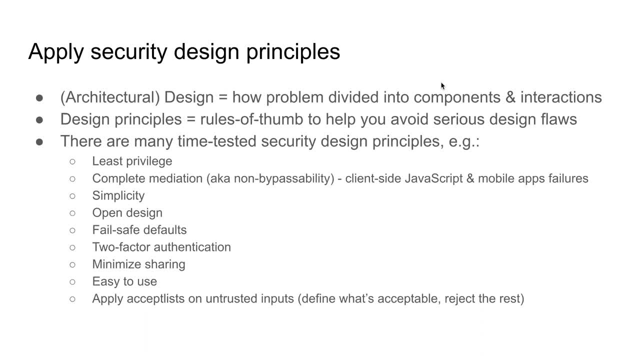 Um, but some designs are way better than others in terms of being secure. So there are some things called design principles, which are basically rules of thumb to help you avoid common serious design flaws, And there's a number of time-tested design principles, things like least privilege- give your software the least privilege it can. 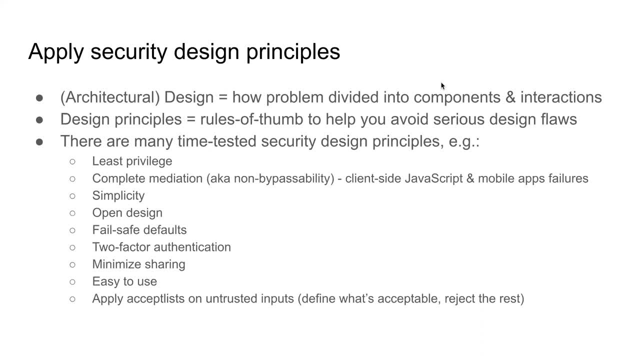 So I just wanted to go back to the, the, the whole concept of the cloud, andもう, you know, and, and, the, the, the, the, the in a lot of what we call the cloud solution, which cowboys call it the cloud solution. 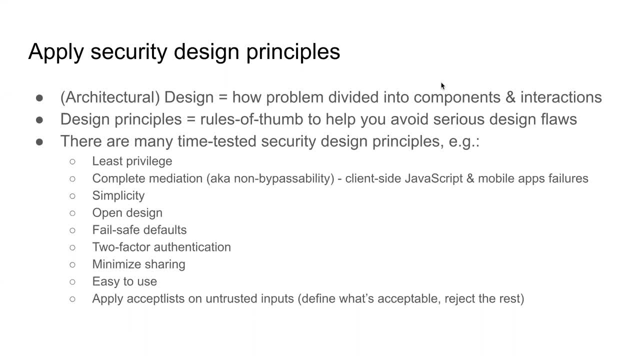 Uh, it's the cloud system, which is very, um, very similar to what we call in the cloud system of of cloud solution, And it's not a real cloud solution. Uh, in, in a lot of cases it it's more of a cloud solution. And so it's. it's a, it's a kind of a cloud solution. So I'm going to talk a little bit about that in a second. Go for it, Uh, okay, Well, let's, let's take a look. 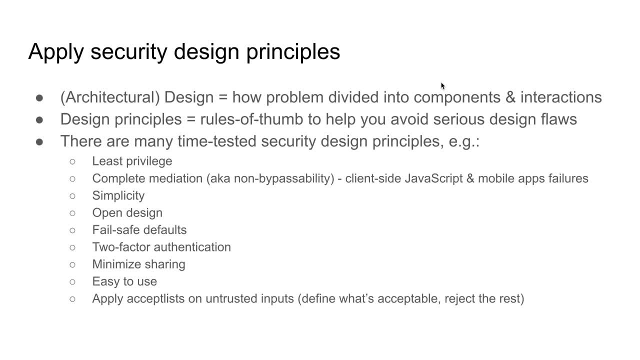 Okay, So the, the, the, the, the. we have a lot of ideas for them. Okay, to be running on a computer you can't trust. This happens over and over again And, by the way, the problem with things like failing to know about or apply least privilege or non-bypassability. 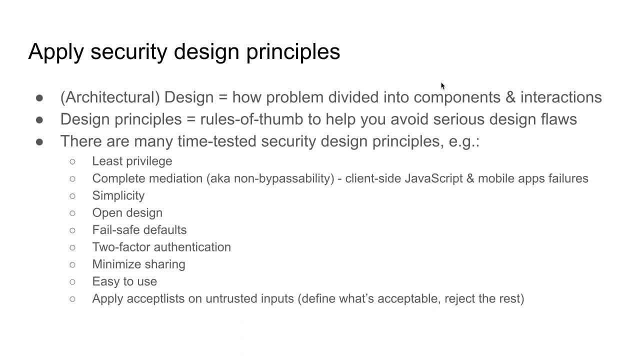 is that it's often a lot of work to change your code later to fix the problem, Whereas if you knew about them ahead of time and applied them, it's no big deal. I've often heard that security can be expensive. Well, it's not usually very expensive if you think about it ahead of time. 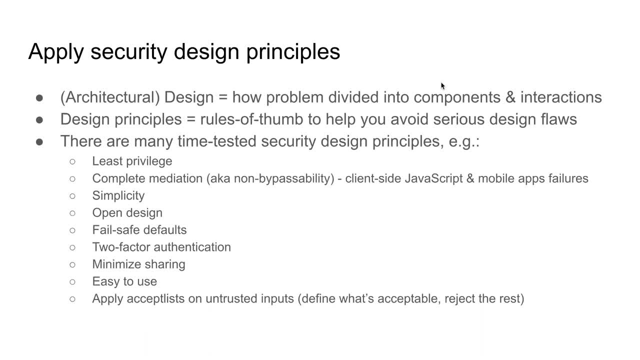 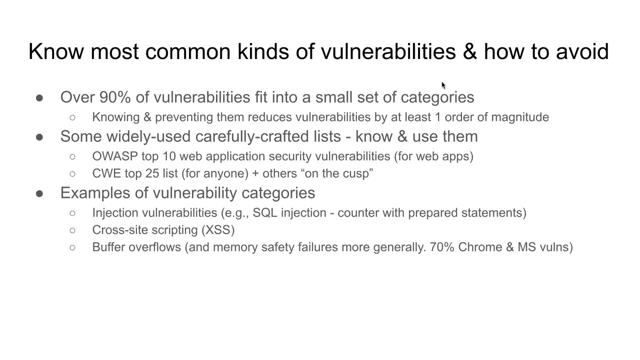 But if you have to rejigger all your code, trying to retrofit security is typically what's expensive- not security, But retrofitting security. oh yeah, that can be very expensive. I mentioned earlier you need to know the most common kinds of vulnerabilities and how to avoid. 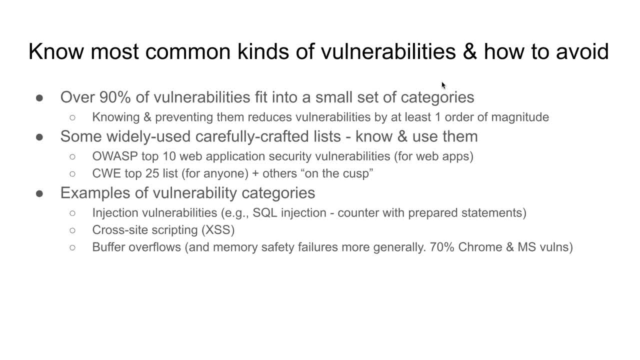 them. Depending on how you measure, over 90% or maybe even 99% of vulnerabilities fit into a relatively small set of categories. So if you know about those categories and know how to prevent each one and do that, you can reduce your vulnerabilities by at least an order of magnitude. 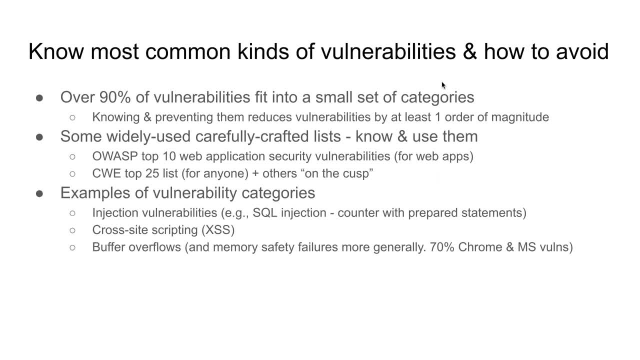 There are some widely used, carefully crafted lists of common vulnerabilities. You should know them. You should use them If you're using web applications. a lot of folks use the OWASP top 10 for web applications. If you're doing anything else, a commonly used list is the CWE top 25 list. 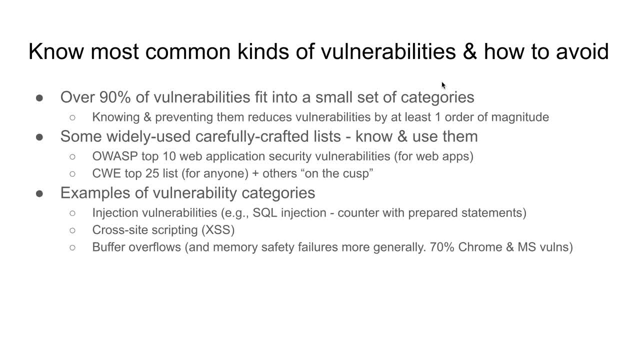 Top 25 is actually a little bit misleading, because they do list 25, but they also list on the cusp, which are a couple actually that aren't the top 25, but maybe you should think about those too. The good thing is, once you know about these common kinds of vulnerabilities and 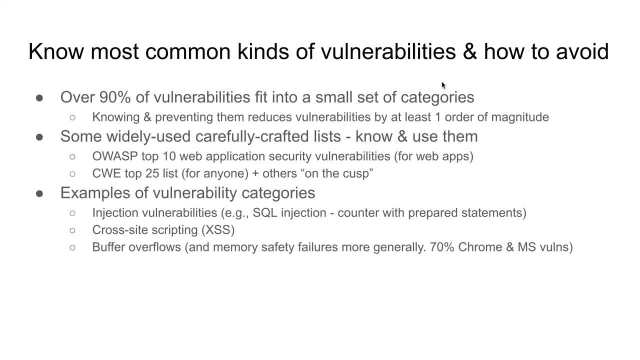 how to avoid them. you squash an incredible number of vulnerabilities in your software, So here's some examples: Things like injection vulnerabilities. There's a common problem that can be a disaster, in particular for web applications, called SQL injection, And these are incredibly easy to counter If, instead of 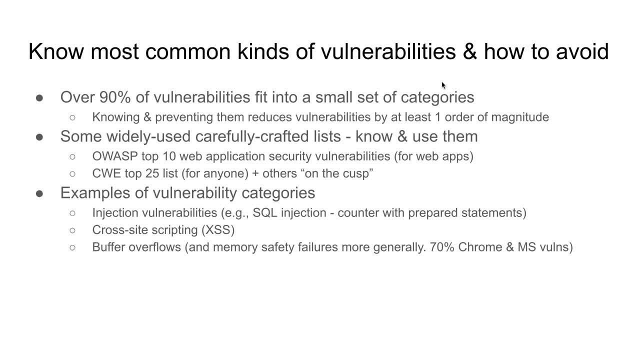 concatenating strings. you use something called prepared statements. then the code is easier to see, It's sometimes faster, It's easier to understand and it'll counter SQL injection attacks. Another common problem is cross-site scripting. Another problem is buffer overflows. 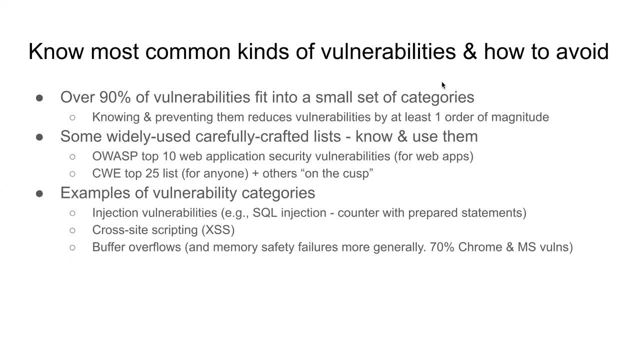 which is actually a subset of a larger category called memory safety failures. These are still endemic. 70% of the Chrome vulnerabilities and of Microsoft's Chrome vulnerabilities are memory safety failures and have been for many, many years. So once you know about these, you can. 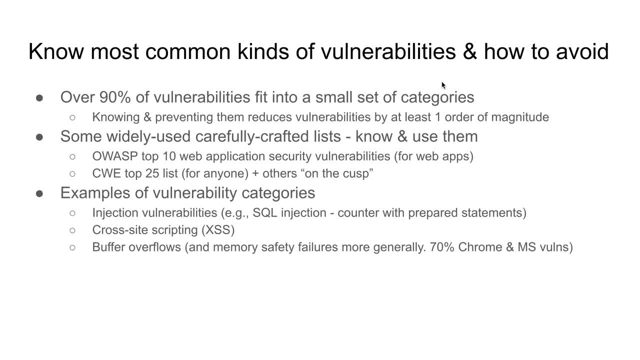 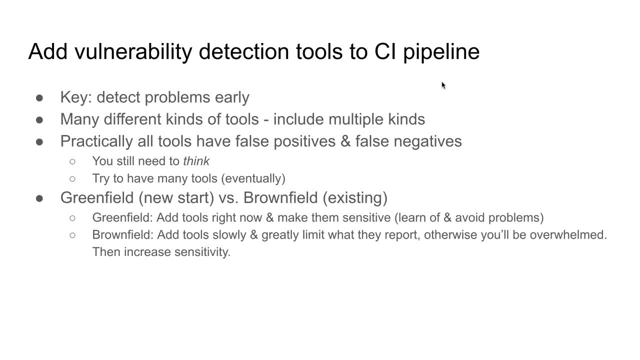 start countering them and eliminating them as a problem for your software, as vulnerabilities. Now, I mentioned earlier, you need to do more than just know in your head. You need to apply, but you know what. It's hard to be perfect, So it's important to also add vulnerability detection. 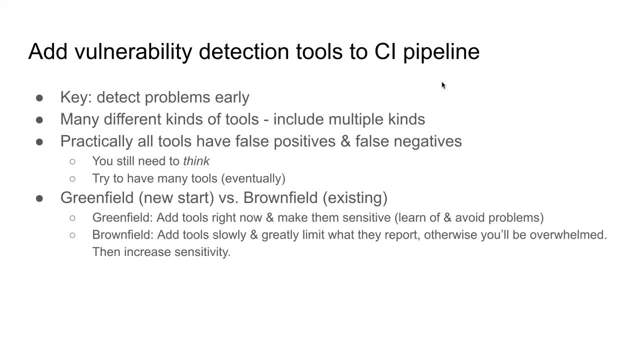 tools to your CI pipeline. The key here is to detect problems early. okay, Now there's many, many different kinds of tools. You should include multiple kinds and, in many cases, include multiples even of the same kind. You can think of tools as a kind of automated reviewer: Different reviewers, human reviewers. 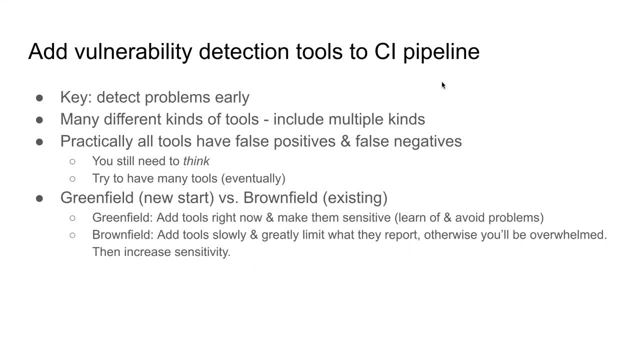 will notice different problems. Different tools notice different problems, And so you really want to bring a suite to them to bear. Practically all tools have both false positives and false negatives. They're almost always going to have at least one, and typically both. False positive means that it's going to report something that isn't really. 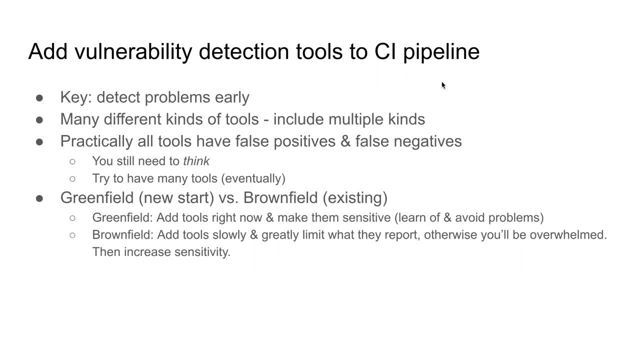 a vulnerability. False negative means it's not going to report something and it was a vulnerability. What does this mean? You still need to think The false positives means just because a tool reports something, it doesn't mean that's an actual problem. You need to figure out what to. 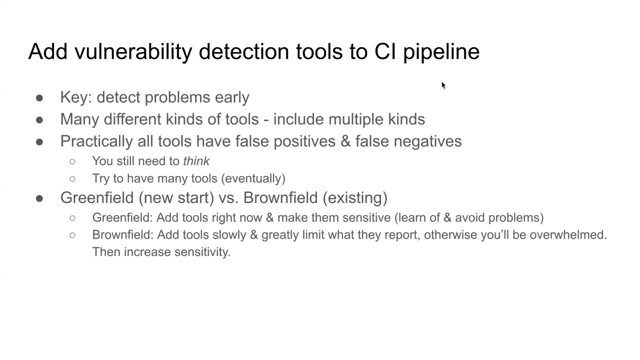 do about it? Maybe you don't need to change your code. Maybe you just need to tell the tool that, no, that's not really a vulnerability. Or maybe you need to change how you do this- develop your software so that that false positive is no longer. 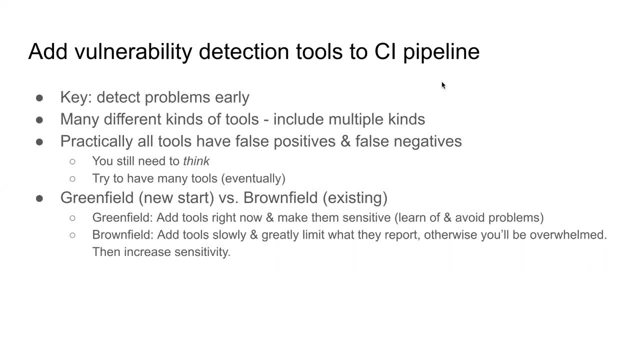 triggered. False negatives are a problem, of course, because the tools aren't going to find everything, which means you still need to know how to develop secure software. You still need to apply those design principles Again. try to have many tools. 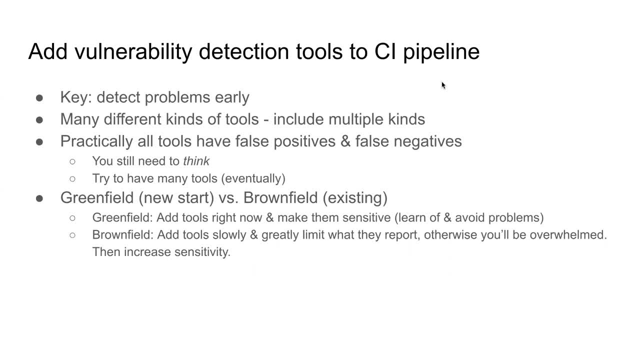 Now there is a really different kind of strategy you'll need to apply, depending on whether or not you're doing a Greenfield project or a Brownfield project By Greenfield. I mean, it's a new start. There's no code Brownfield. oh man, here it is, Congratulations, It's a million lines of code. 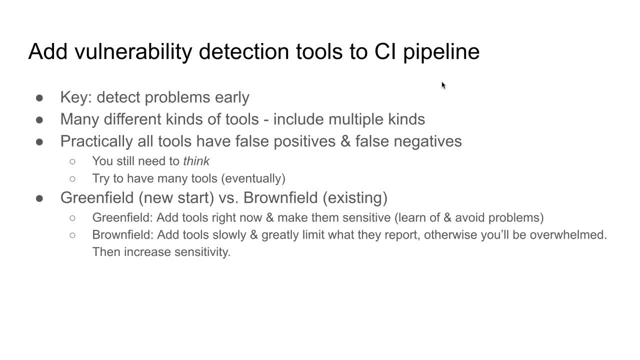 It may have been around for years. If it's Greenfield, a new start. typically you want to add the tools right now, probably as many as you can Get them into your CI pipeline, Make them really sensitive. Why? Because the instant you start writing code at all, it'll immediately warn. 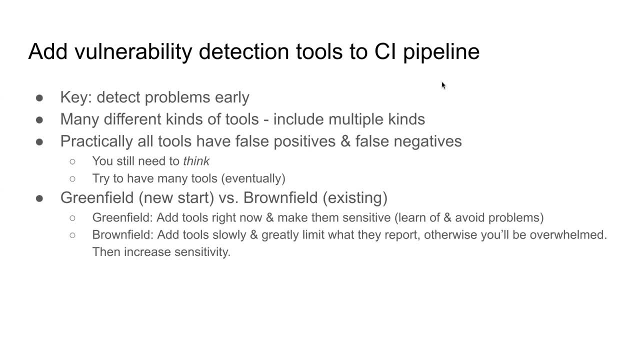 you about problems and constructions. You're going to have a lot of problems. You're going to have a lot of constructs that are dangerous And you can- oh, I guess I see that- Do this instead, And then all the rest of the code will apply. those lessons Brownfield's very, very different. 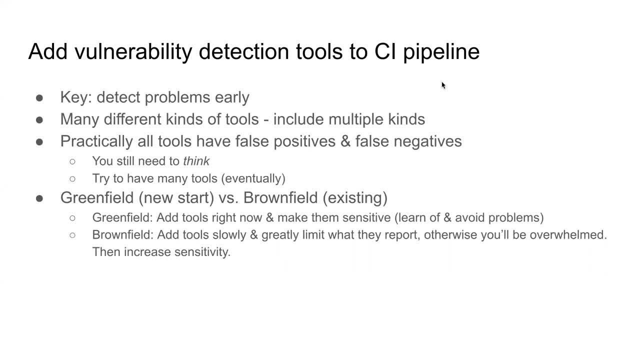 If it's an existing project, you typically need to add tools very slowly and start by greatly reducing their sensitivity, Really limit what they report and then slowly increase their sensitivity over time. The problem here is that if you're doing a Greenfield project, you're going to 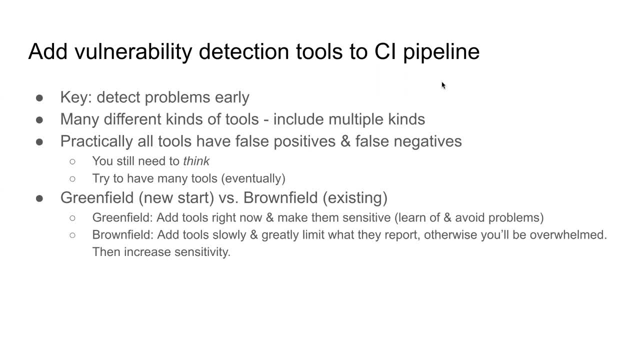 just add a whole bunch of tools and make them sensitive, You'll be completely overwhelmed with reports. Oh look, there's a billion reports. I can't possibly handle that, Right. Okay, Start with very few tools, Start with the most important limit and then add things over time. 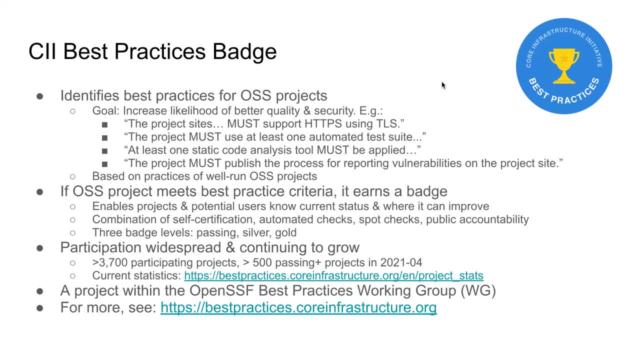 There was a question earlier about the CI best practices badge. Let me talk a little bit more about that. The CI best practices badge is essentially a list of criteria of best practices for open source projects, And the goal of those criteria is to better improve quality and security. So here's an example of some of these criteria. 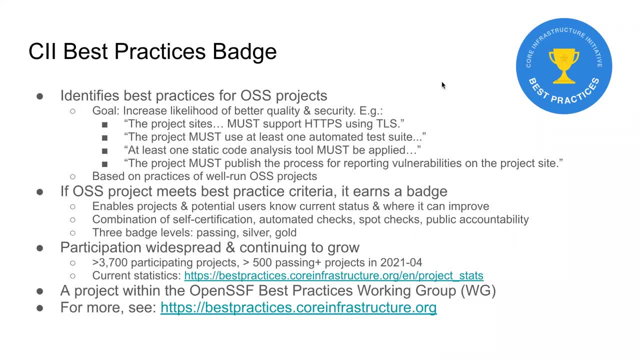 You know, the project sites must support HTTPS, They must use at least one automated test suite, At least one static code analysis tool must be applied, That's a tool that analyzes the code without running it, And the project must publish the process for reporting vulnerabilities, Because 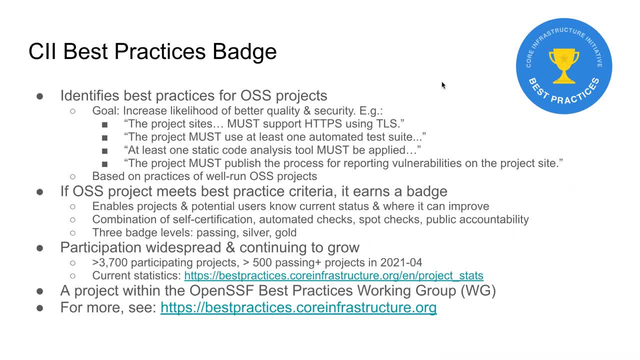 you know, even after you do everything, there may still be a vulnerability. Make it as easy as possible. People report it back to you, And these are based on the practices of well-run open source software projects. If an open source software project meets those criteria, it earns a badge. 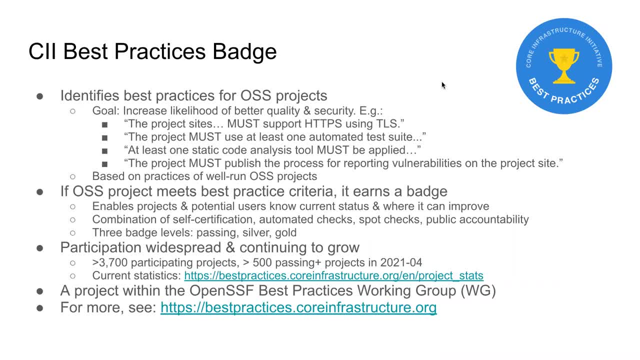 And this enables projects and potential users to know its status. So there's that question earlier about you know if I'm a potential user. what do these do for me? Well, they help you figure out. oh wait, a minute. this project is working hard to apply a lot of good. 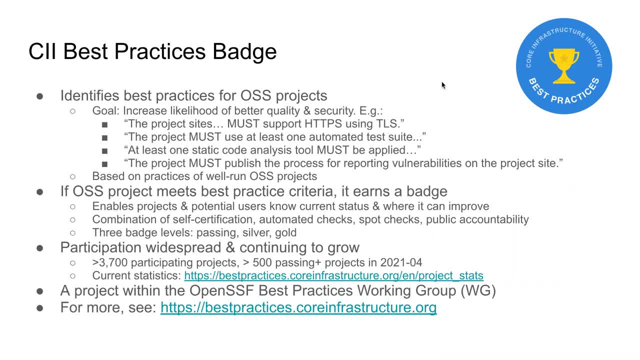 good practices. There are actually three badge levels: passing, silver and gold. But I'll note that even getting a passing badge is a significant achievement. Participation's widespread I have on the slide deck is 3,700.. It's actually over 3,900.. We're getting really close to 4,000. 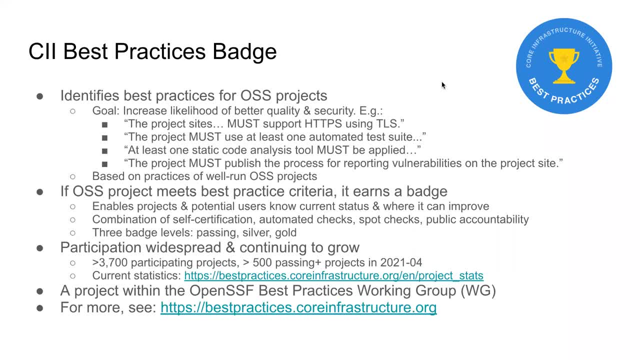 participating projects. There's over 500 passing projects And you can see the current statistics right there in that URL, And this is also a project that's being done. So you know if you're a project within the OpenSSF Best Practices Working Group. Now, if you are a user of open source, 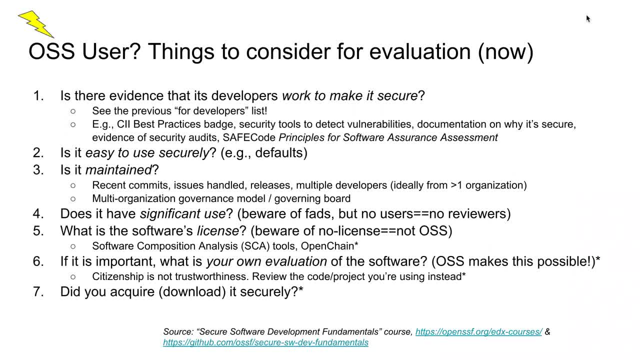 software. okay, including, by the way, a developer software that's using other open software as a dependency. And, by the way, that includes most software developers. So what do you do? Well, number one: is there evidence that developers work to make it secure? And oh, by the way. 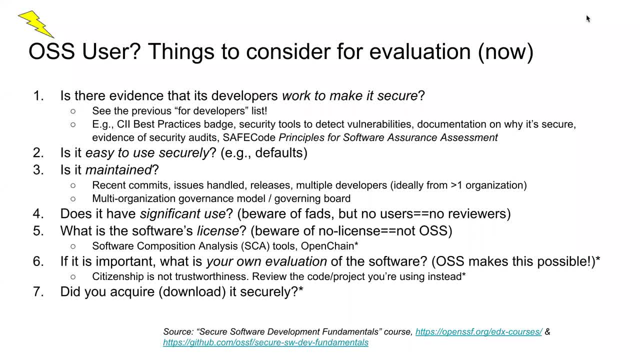 all those things I just told you before about how should developers develop secure software. Now, your job is to make sure that your software is secure. So if you're a developer, look to see if they're doing that. Okay, Are they doing things like applying the CI Best Practices? 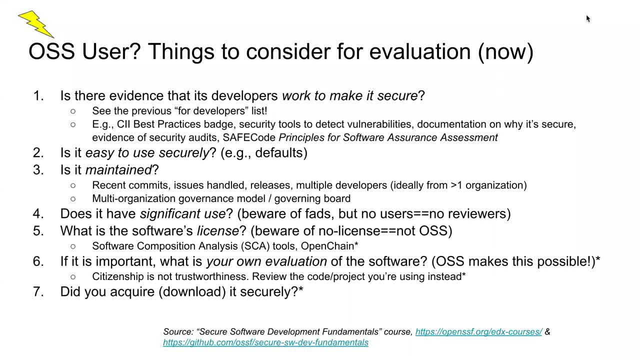 badge Number two: is it easy to use securely? Three, is it maintained? You want to look for things like recent commits, multiple developers. Does it have significant use? Now, I have to be careful here. There is a real problem in the software development world with what I call. 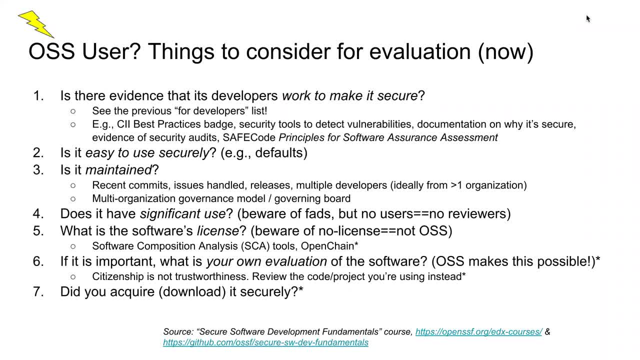 fad engineering, You know. oh, big company X uses it, Therefore that must be the right software for me. No, Actually, they probably have been using it for a long time. They've been using it for a long time. 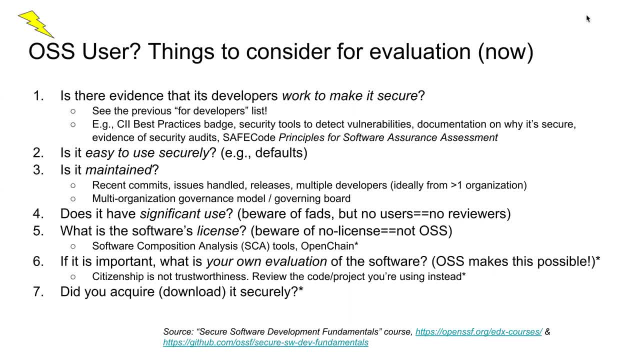 Very, very different problems than you do. So you know, just because somebody else uses it does not mean it's an appropriate software for fewer circumstances. However, there is something to it. If there are no users, there's probably going to be, no reviewers, It's probably not going to be. 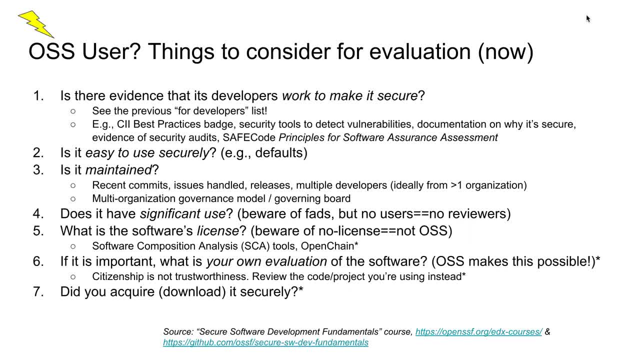 maintained well in the future. So you know it should have some use. What's the software license? We still have people today who have the misguided thought that if there's no license on the software, it's open source or it's usable by anybody. The law around the world has not changed because 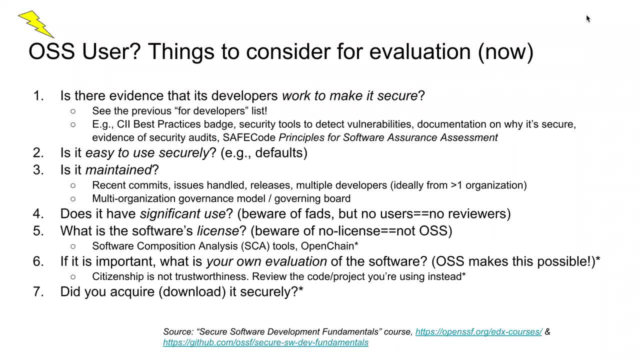 some people think that, okay, The law is the law, And if you want to be allowed to use the software, it has to be licensed. This isn't some ideal. This is what laws around the world say, So there are various tools that can help you identify the components within them. to figure. 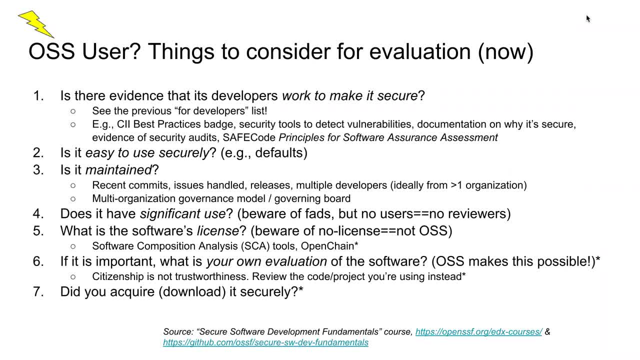 out things like the license and also if there's known vulnerabilities in them. If it's important, what is your own evaluation? Okay, And the great thing about open source software is that it makes it possible. I like to note to folks that citizenship isn't. 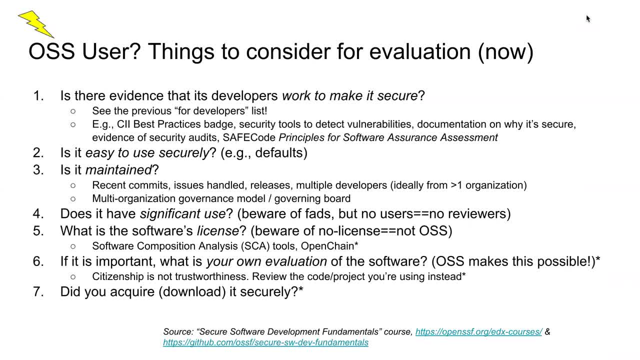 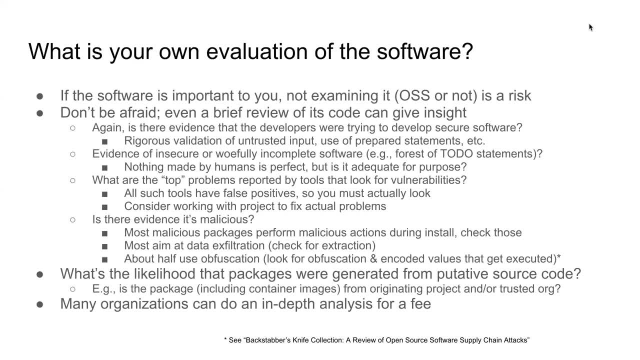 trustworthiness. If you want to trust something, look at the code And did you acquire it securely? And the biggest problem there is: did you acquire the right thing? Now I mentioned evaluation. If the software is important to you, not examining it is a risk If you just take some bits. 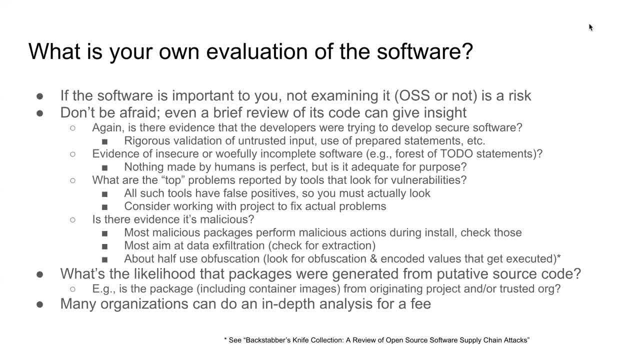 whether it's open source or proprietary. that's a risk, Okay. So I think it's often a good idea to review the software, because even a brief review of the code can give us some insight. You know again, is there evidence that developers are trying to develop secure software? 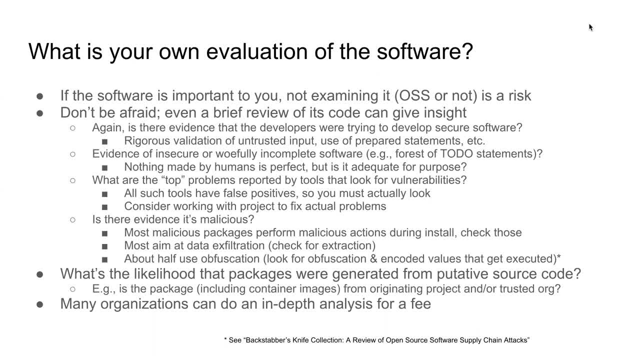 You can often find some evidence of insecure, woefully incomplete software. You know run some tools against it. You can look for evidence of maliciousness And, of course, you know, trying to figure out the likelihood that the packages were developed. 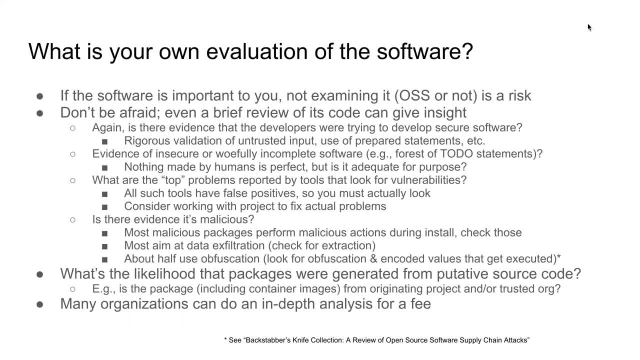 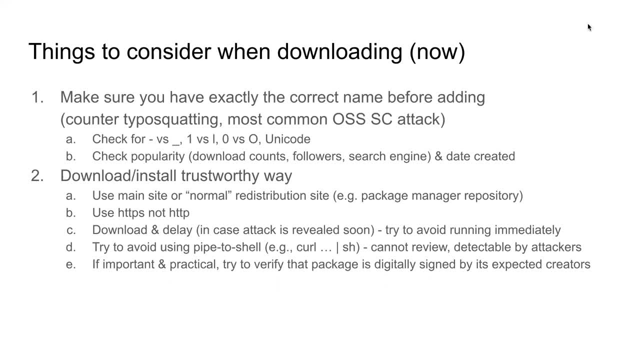 were generated from the source code it claims, And there are folks who can do that for you for a fee, if you don't want to do it. Now, when you're downloading some software, there are some things to think about And there are some complicated things Before you go. 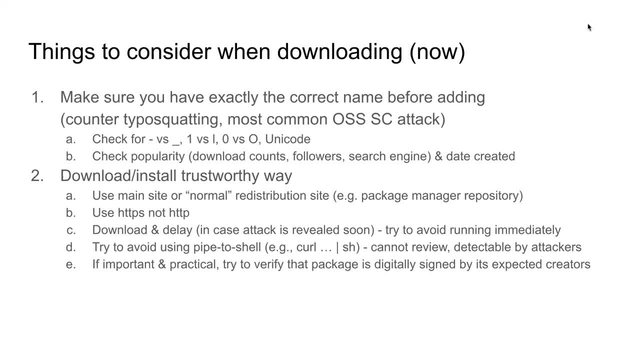 complicated. there's some simple things you can do that can lower risks with almost no cost. First of all, double check the name. Make sure you have exactly the correct name before you add a package. as you're doing it, You can go to your research, sort it out, send it to an email or download it for use. 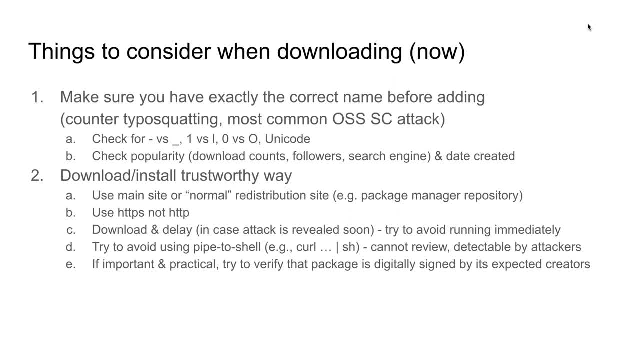 Today, the most common kind of malicious attack on open source software is typosquatting, creating projects that have similar names, but not exactly the correct names. Why? Because attackers can take the easy road, and this is easy: Instead of trying to subvert the software, just make another project. 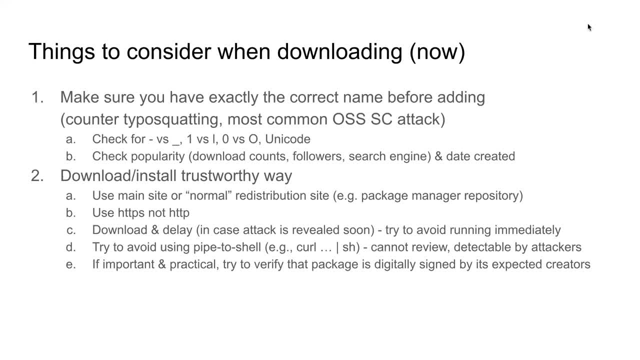 Check for dashes versus underscores ones versus L's Unicode characters and also check its popularity. And that's a whole different thing. Why? Because the attackers can take the easy road, and this is easy: Instead of trying to subvert the software, just make another project, Check for dashes versus underscores ones versus L's Unicode characters, and also check its popularity. 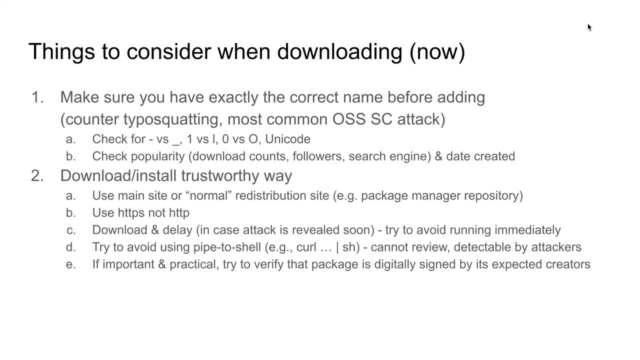 things like you know when was it released, what's the download counts and so on, If you are about to use a package you know has been around for 10 years and it's widely used, and oh look, here's this package. It was created last month. It's got three downloads. 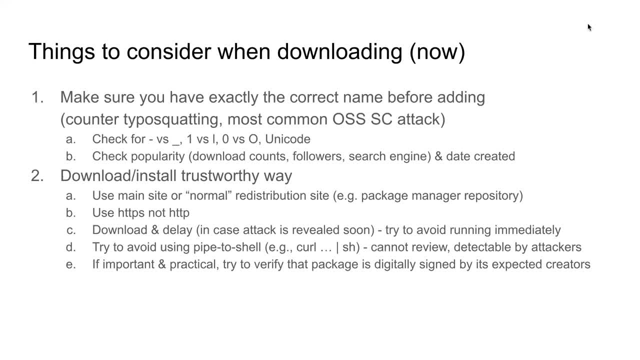 That's not it, right? You don't need to be a genius to realize that's not what you were looking for. So you know, some simple checks can actually avoid a lot of problems. And, of course, download, install in a trustworthy way. you know, whatever its usual redistribution approach. 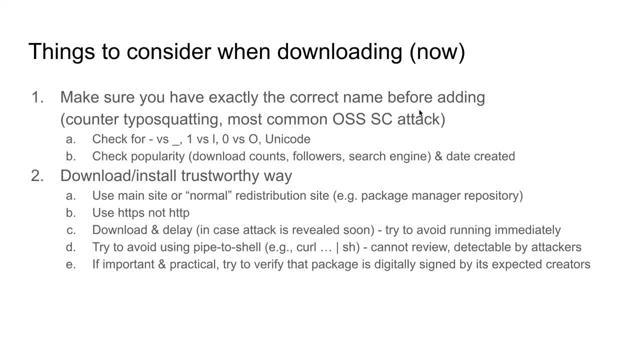 Try to use HTTPS instead of HTTP. One technique that is actually really helpful is download and delay Download, but don't install it quite yet, particularly if you're doing application-level packages, because sometimes if a system, if a site, if a download site gets attacked, it's noticed, it gets fixed, But if you waited a little, 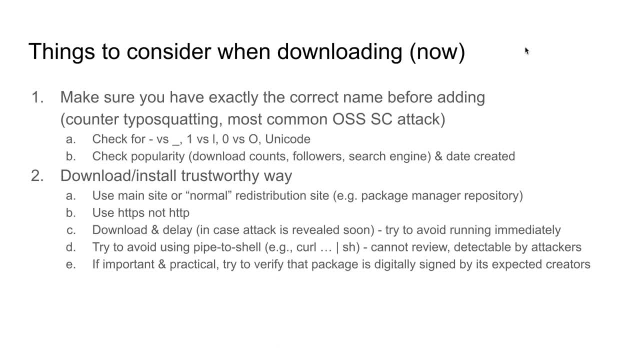 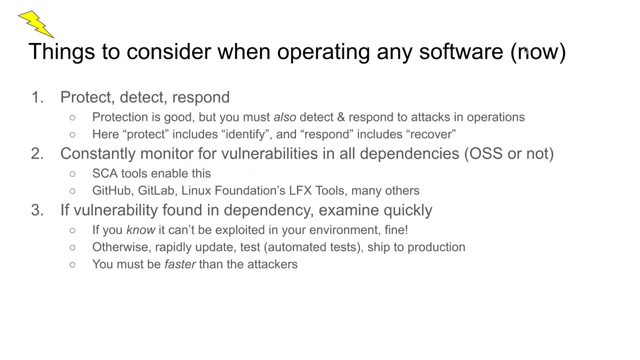 bit then you didn't end up installing the maliciously subverted one. Try to verify it's digitally signed. but the challenge there is that there are challenges today with digital signature and verification. I'll talk more about some efforts to try to deal with that later Now, of course, 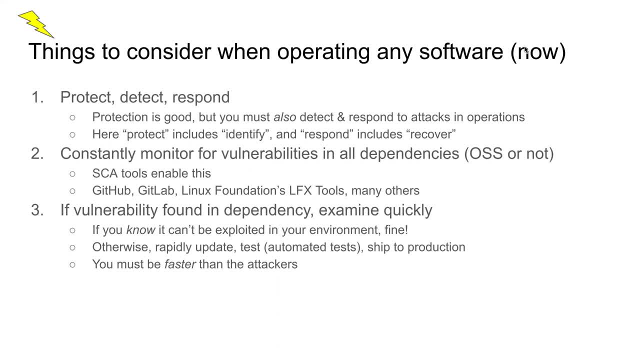 when you're operating the software. you know: protect, detect, respond. you need to protect protections- Great, But you know things happen, so you also need to detect and respond to attacks, constantly monitor And, if a vulnerability is found in a dependency, examine it quickly. 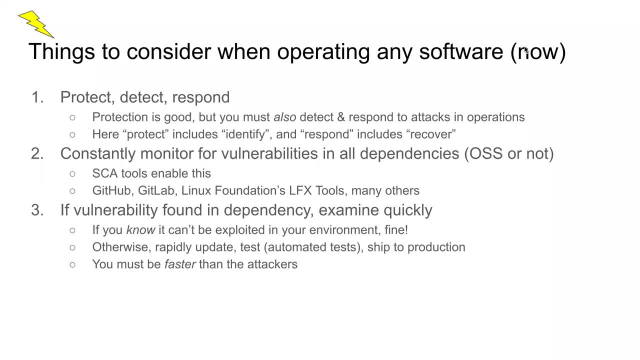 If you know it can't be exploited in your environment, fine, But otherwise you want to rapidly update test ship, as I mentioned earlier, And the key here is you've got to be faster than your attackers. If you're waiting a month, that's probably pointless because the attackers aren't. 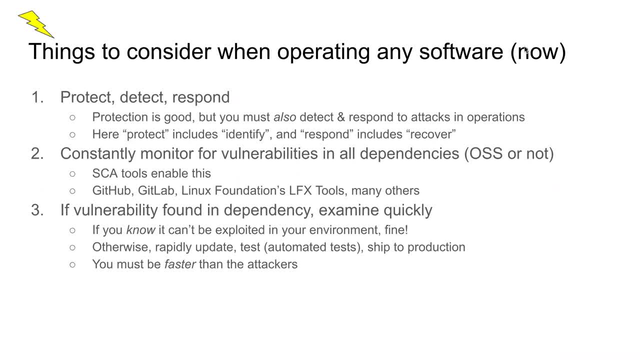 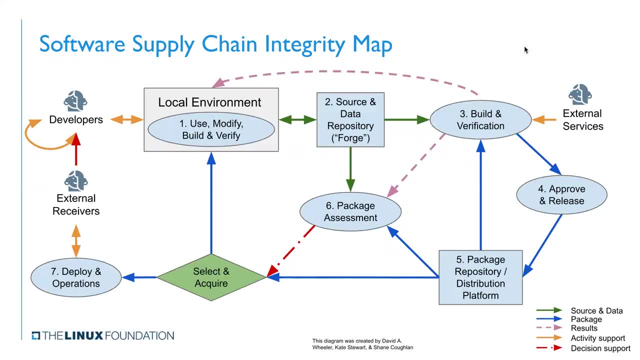 waiting a month, As soon as the vulnerability is found, you're going to be able to detect and respond to attacks, But ideally you want to do it now, So when vulnerabilities become known, the clock is ticking. I don't have a lot of time talk about it, but I should just note that, although attackers certainly 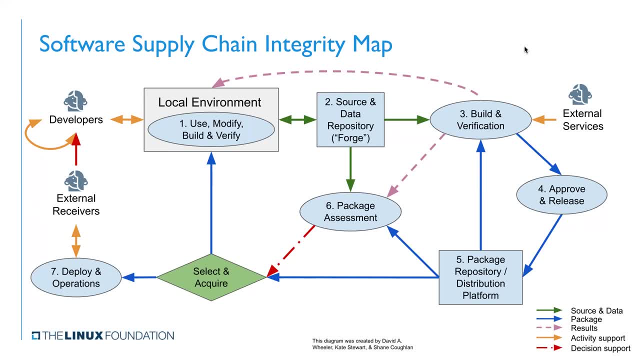 attack vulnerabilities in the software itself. attackers also attack the process where software emerges from developers heads all the way out to eventually being used. So there is a process that's used to develop software. Typically, developers create a local environment. It gets merged into some data source and data repository, build, verify, approve, released as some sort of distribution platform and then either selected directly by users or selected and brought into larger systems which build and build and build. 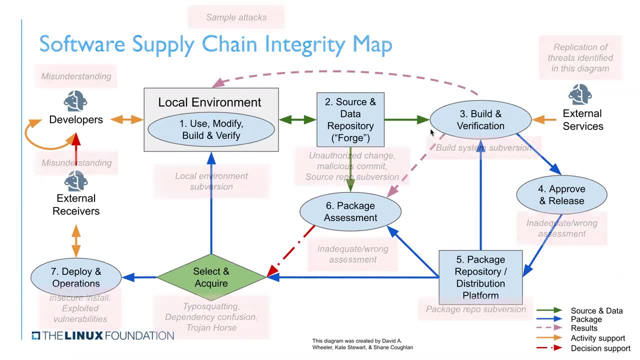 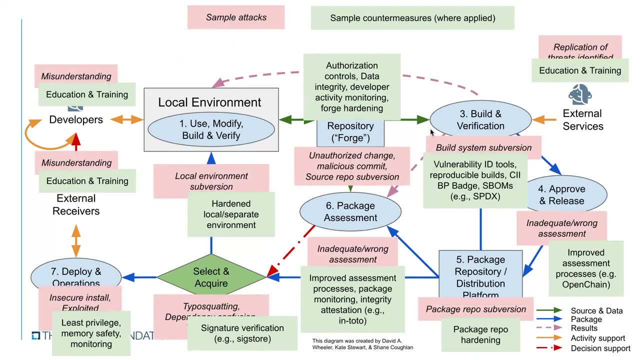 And of course, attackers can attack all those steps. But the good news is that there are many ways to counter those. once you realize, oh wait, attackers will try to attack me, but I don't just have to accept that I can actively work to counter them. 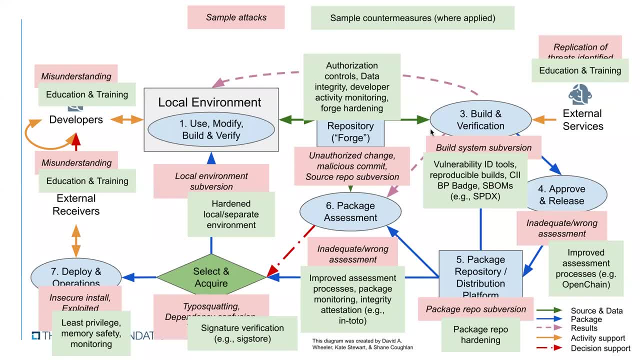 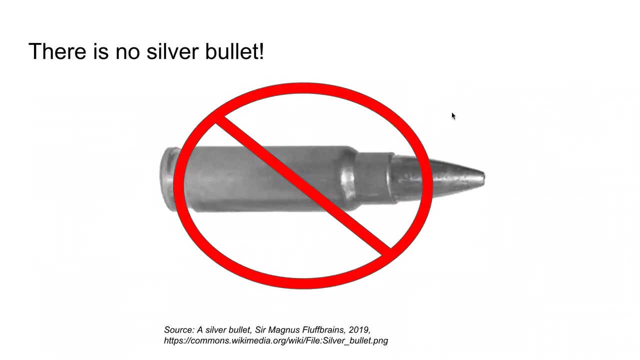 Things like using two-factor authentication for my repository, so that arbitrary people can't just guess a password and break in and take over control over my software. There is no silver bullet, Okay Now. so you really need to think about a number of different things. 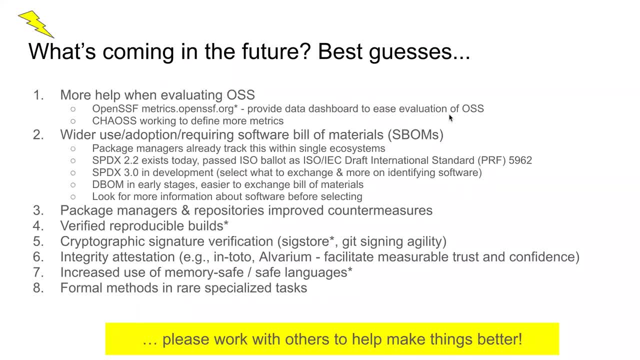 Now, what's coming in the future? My crystal ball is a little fuzzy, but here are my best guesses. I think we're going to see more help in evaluating open source software. I'll note that OpenSSF is working on providing a data dashboard. 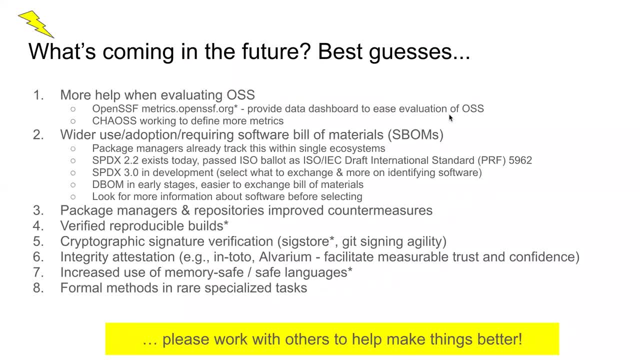 MetricsOpenSSForg, CAS is working to define more metrics. There's a lot of folks working on trying to make it easier to evaluate open source software, so that at least you know: hey, there's three different open source software packages. which one should I use? 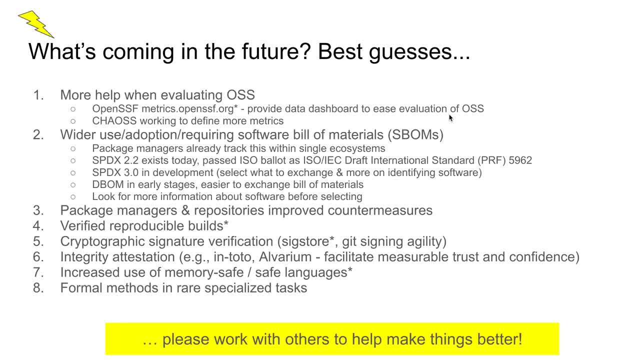 You can have better information Next up: wider use, adoption and requiring software build materials. A little earlier this year, the US White House released something called the Executive Order on Cybersecurity. It includes a number of things. It's including a number of requirements and statements about software build materials. 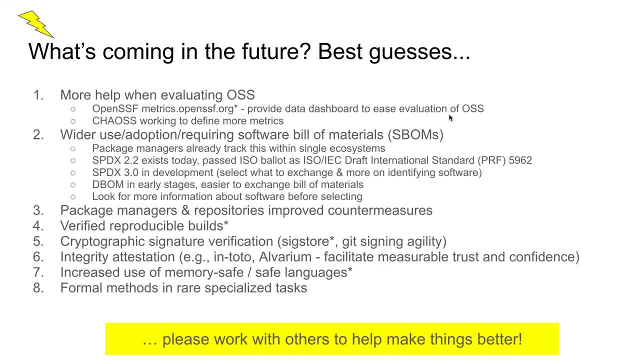 Today, generally when users get some software, they have no idea what's inside them. Okay, And it looks a whole lot like the world of medicine, looked like in the early 1900s, late 1800s, where you know people would hand you medicine and Lord only knows what was in there. 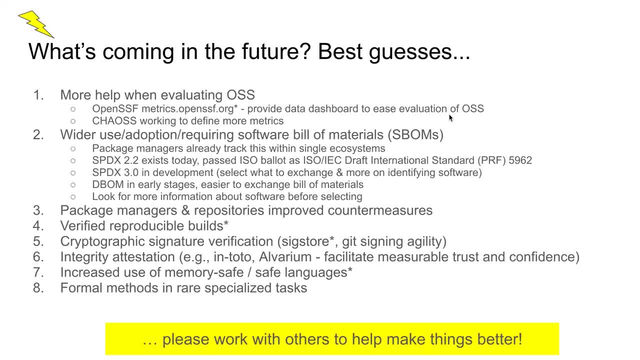 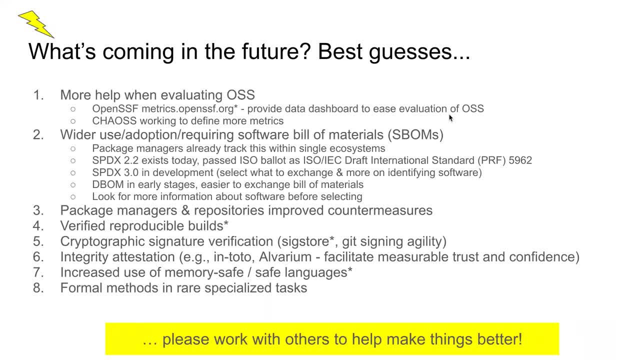 You know it might be some illicit drugs or things that you might not have otherwise wanted to put in. You know it might be some illicit drugs or things that you might not have otherwise wanted to put in, And yet for software, we have no idea what's inside there. 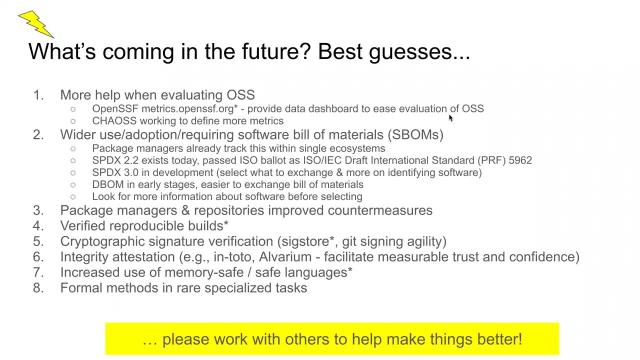 Packaging managers can already track within single ecosystems, the software within a system, But there are standards now in development or released that let you share software build materials, in other words, the ingredients of a larger piece of software. I'll note that SPDX exists today. 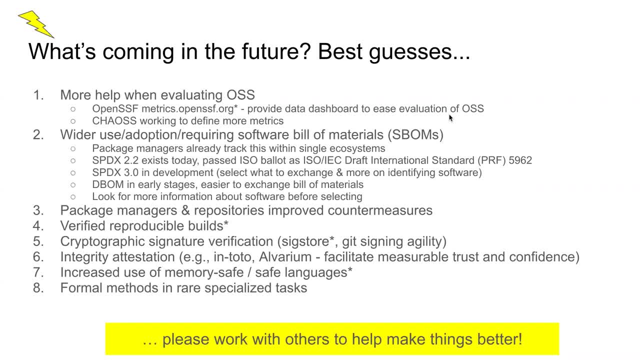 It's now at the PRF And there's some other work as well. So basically, there's already work ongoing to enable sharing the software build materials, And I expect to see more of that in the days ahead. I think package managers and repositories are going to improve their countermeasures. 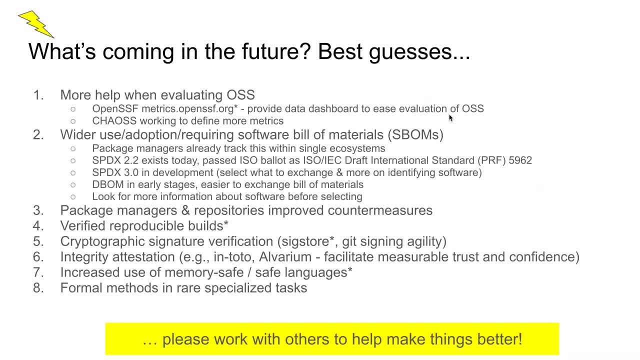 There's something called verified reproducible builds, which lets you verify that the bits that you're about to install really did come from the source code. There's something called verified reproducible builds, which lets you verify that the bits that you're about to install really did come from the source code. That was evaluated by developers. The lack of this was, for example, a problem for the recent SolarWinds debacle with Orion, where the code that was being installed and run was actually not generated strictly from the source code that was developed by the developers. 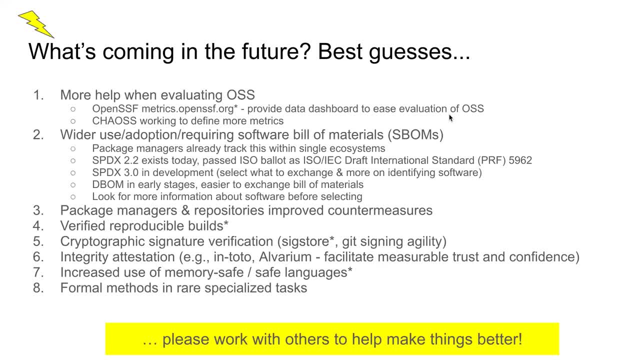 You know, the developers developed code and they reviewed it, but that's not what was used to be shipped to developers, because someone subverted the development process, The build process, actually Cryptographic signature verification. From a mathematical point of view, cryptographic signatures are solved. 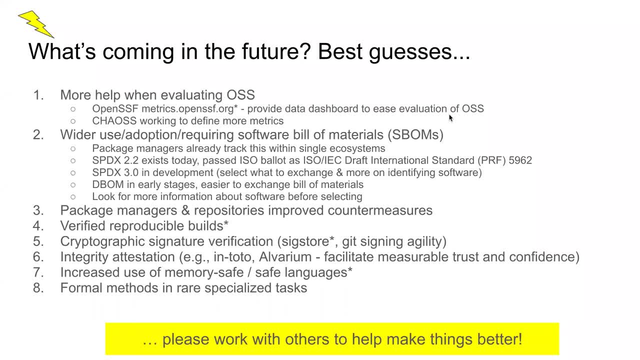 We know how to do it math-wise, But there's a lot more to the world than mathematics. Applying cryptographic signature verification in the real world has turned out to be a challenging problem, And so one Linux Foundation project is called SigStore, which is working hard to make cryptographic signatures. 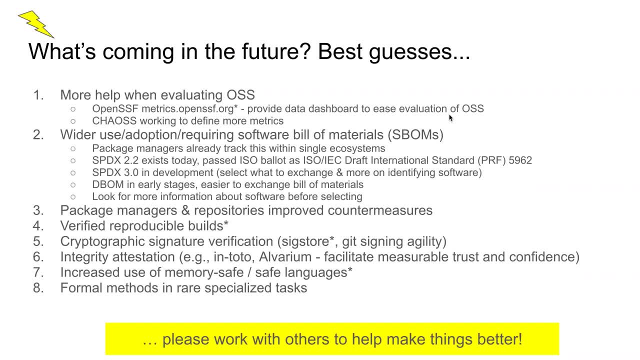 It makes signature verification much easier. also working on improving get-signing abilities. Integrity attestation: There are things like Intodo and Alvarium to help with attestation of integrity. Increased use of memory-safe and safe languages: If performance is not super important, there's a huge number of programming languages that are available that are also memory-safe. 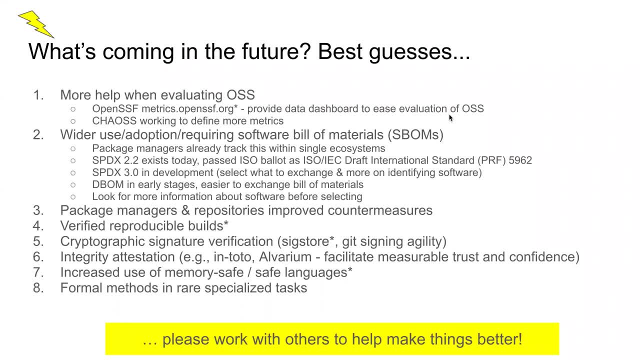 But when you really need strong, Very good performance. A lot of programs today are written in C and C++ which are not memory-safe, And this has led to 70% of the vulnerabilities today in a lot of systems are memory-safety problems. 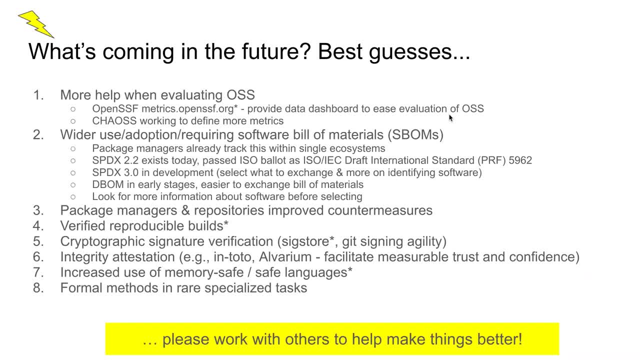 So increased use of languages that just prevent this whole cough, I think is very promising And is likely to continue in the future. I think that full methods are going to continue to be used in rare specialized tasks. I'd like to see a little more of that, but I don't think that's going to be common. 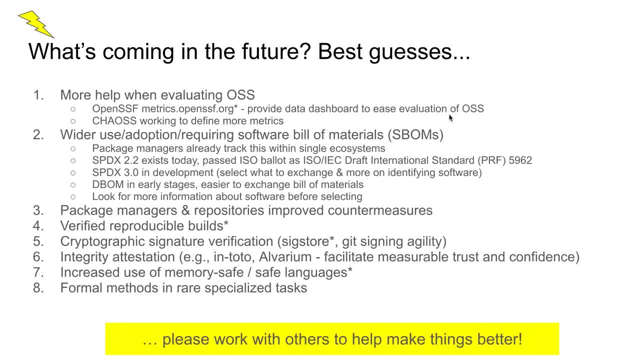 Happy to be proven. I don't want to be proved wrong in that, but I think we are going to see them in some specialized tasks Now. please work with others to make things better. Okay, Because the future is whatever we collectively work to make it. 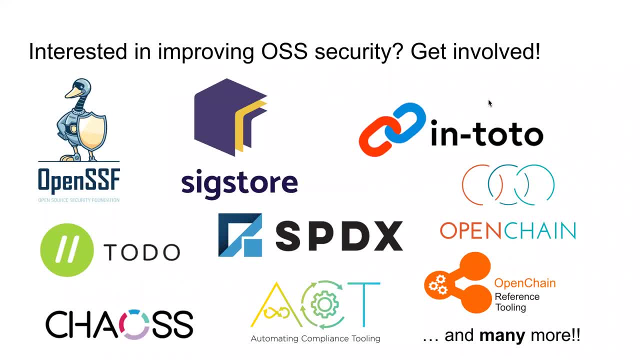 If you are interested in improving open source software, the open source software security, then the answer then is get involved. Okay, And here are just some of the organizations. I've mentioned, most of them now. Okay, There's, of course, the Open Source Security Foundation. 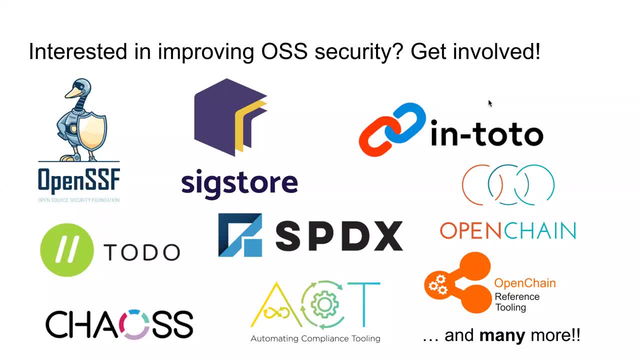 SIGSTOR in TOTO. There's many others. There's many others. frankly, I'm not putting them on this list here. The point here is: if you want to improve the security of open source software, get involved. And this is not to say that, oh my gosh, open source software security is a disaster. 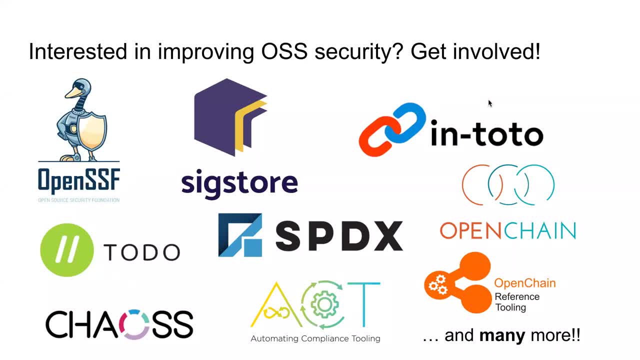 Not at all. You know there's a lot of really secure open source software. Open source software has some real potential advantages For security Because many people can review it and get it fixed. But those potentials are not always lived up to. 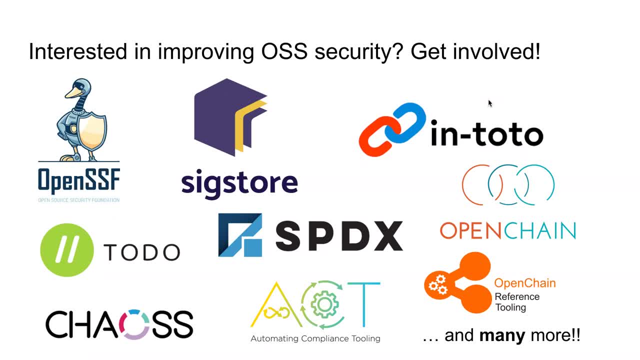 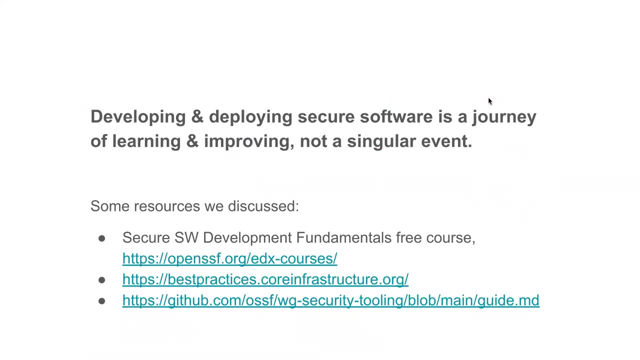 And, frankly, we don't want just good, We want really good, Because we're all dependent on this stuff. So we want to make things better and better over time, Which really leads to this bigger point here: Developing, deploying, secure software. 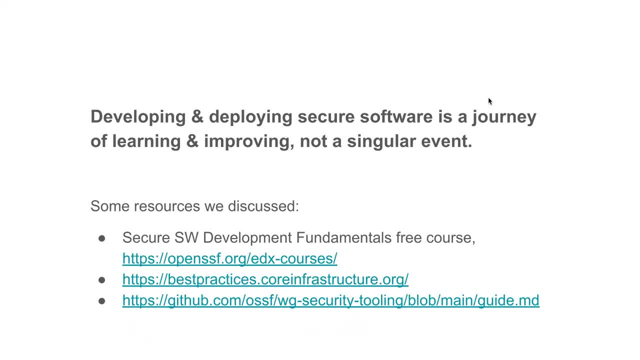 It's really a journey. It's a journey of learning. It's a journey of improving. It's not really a singular event. Because of the way the English language works, it's often easier to use. you know perfections and goals. 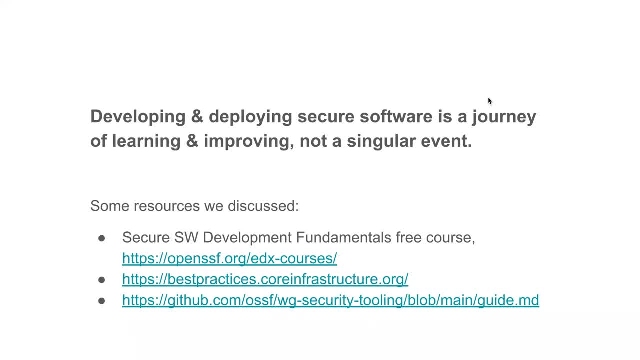 But the reality is that there's always going to be ways to improve security, even if it's not vulnerable. Hey, you know, we can change the software so that it's even less likely to get a vulnerability later. It's going to have stronger defenses. 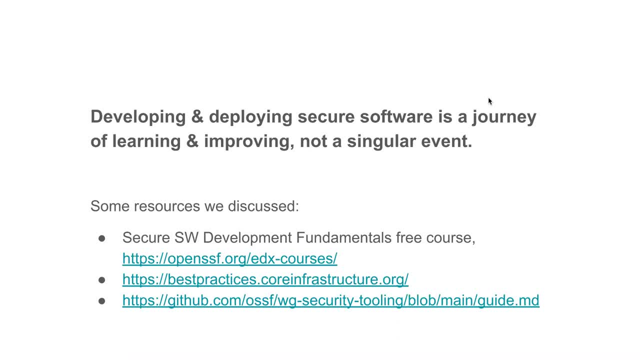 So here right below are just a few links to a few of the things that I've mentioned here. I already mentioned the free course. I don't have time to cover a whole course in this very short time, But I'm hoping I'm giving you a flavor of it. 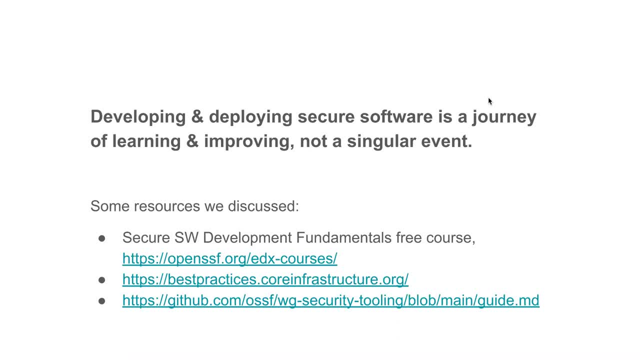 Because, in the end, I think that that's, in many ways, the most important thing: Understanding Some education, Some training. Once you know how to develop secure software, a lot of other things can become easier, And it's one of those things that will pay you dividends through the rest of your software development. 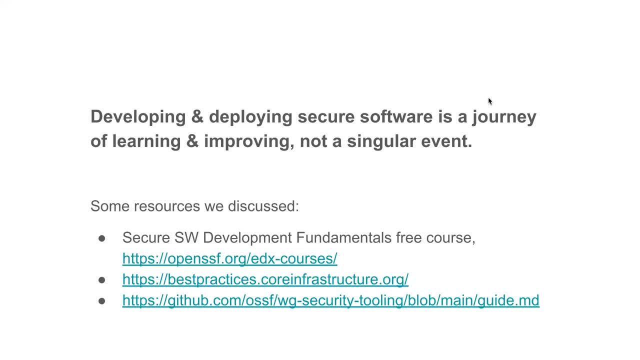 Of your software development career. The best practices core for structureorg is where the CI best practices badge project well lives, Or at least you know that's where you can get started to get a badge. Here's a little guide on how to use tools. 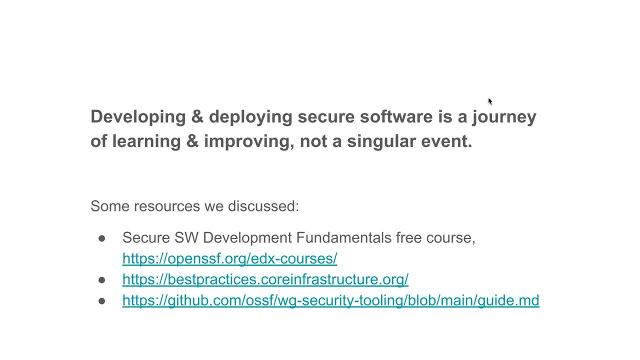 There's many other guides, But, you know, the key is get some tools into your process so that it can start into your CI process, So that you can start detecting vulnerabilities, Building on what you already learned from. you know: some course of some course. 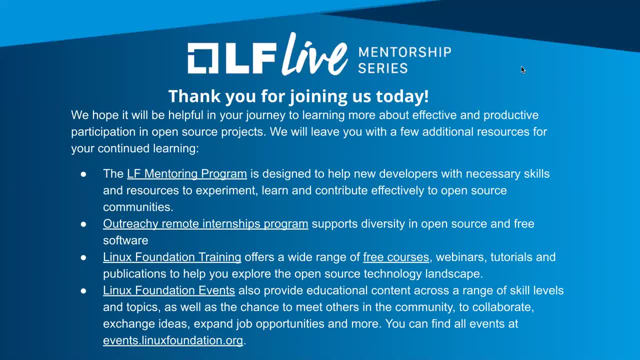 And you know any kind of course, All right. So I wanted to leave a lot of time for questions, So I'm I've tried to get through- I know a lot of material relatively quickly. I have lots of backup slides If you want to ask specific questions or go in a particular way. 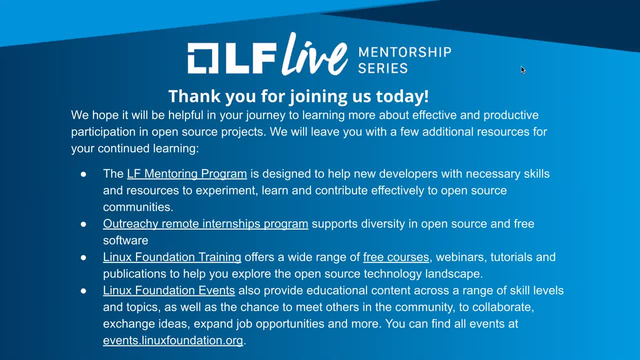 But I'm really interested in helping you today. I want people to leave here feeling that the important questions to them were answered, And I just want to point out that this is, of course, part of the LF live mentorship series. mentorship series, uh, and that's really kind of the goal of all of these um events. uh, for an lf live. 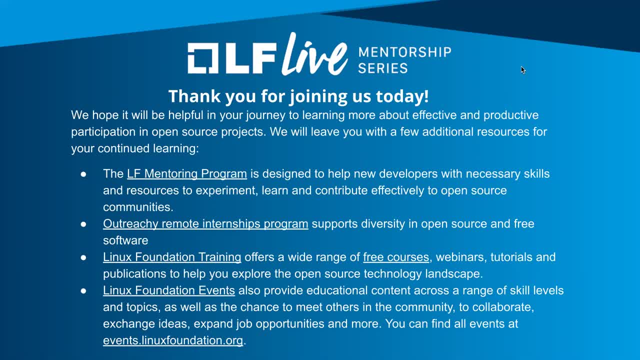 mentorship is basically we're trying to give you some information, but we also want to, you know, discuss and answer your questions to the best we can, um, so that you can go away and apply and you know and, uh, you know, be glad that you were part of the experience. all right with that, um. 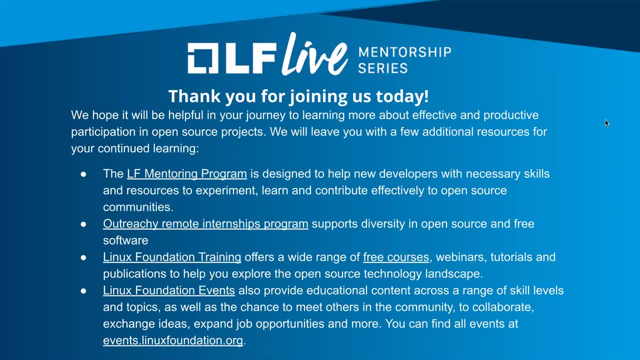 let's see here. uh, i'm gonna. i guess i'm going to start with looking at some of the questions up. that seems to have been built up as we went um, so let's see here. oh, yes, okay, so the c, the top 25, there's a link there, sure, um, you know, there's uh, if you just 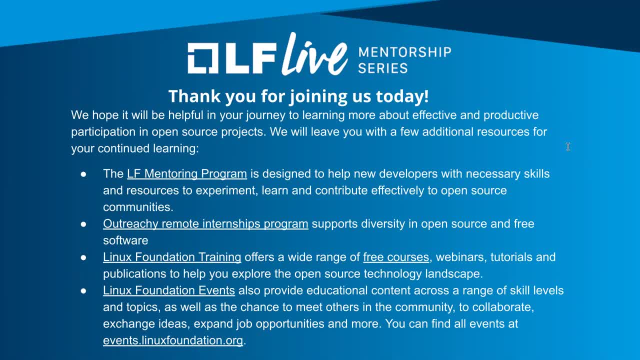 do in cwe top 25, you should be able to find it quite quickly. um, yeah, so, and in fact, if you take that, uh, the course that i've been mentioning earlier- which, by the way, i make no money if you go to, if you go to edx. 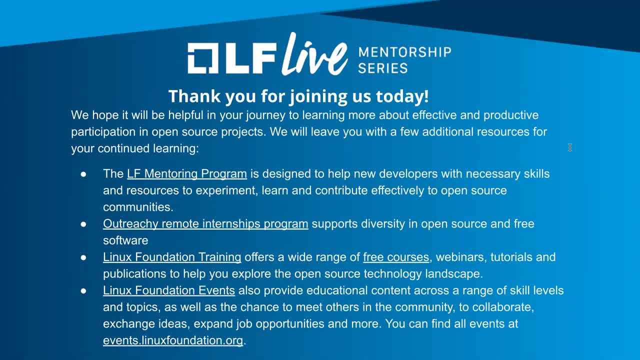 and you take the course: i make no money, you pay no money. um, i am very, very excited about this particular topic. i think it's very, very important and, um, one of the things that i made sure- because i actually uh wrote that course um- is that i made sure it covered um all those top things. so you 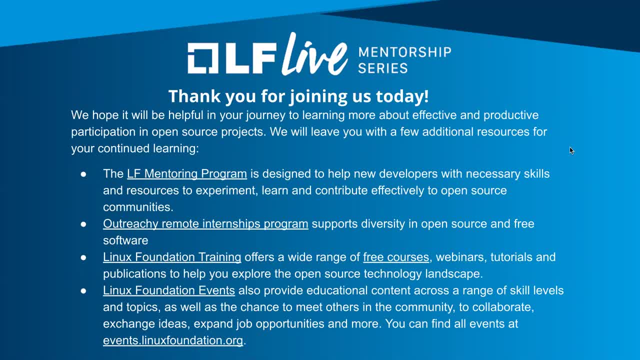 will actually walk through those various top items and see various options on how to counter eagle. what is it and how do you counter them? all right? how are we going to address the gap to map security from cve, cpe to s bomb, swid uh connection? 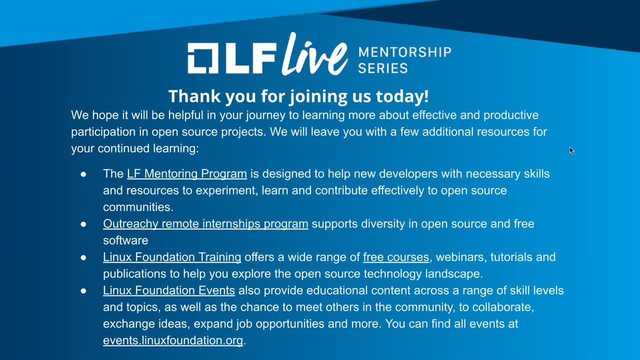 okay, uh, so, um, so, regarding cve, cpes and so on, um, i think that the okay. so, for those of you aren't familiar with this, um, there is a well-known method for identifying vulnerabilities, uh, software vulnerabilities. it doesn't- it doesn't, um, identify them all, but it covers many. it's probably the most most complete collection of any publicly. 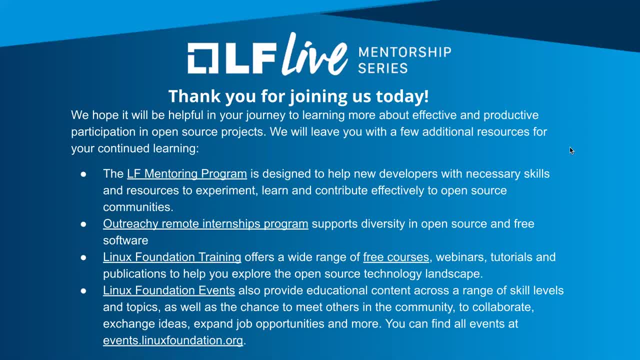 accessible list of vulnerabilities. um, and the idea is pretty straightforward: every vulnerability has a unique id it. they look like cve dash year it was reported, dash some other number to make it unique. um, the current problem today with cves is, although they report vulnerabilities, they don't record- uh, almost all the vulnerabilities, um, they don't record in their 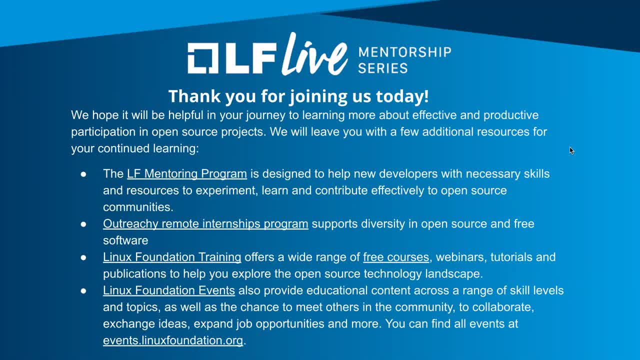 information any way to automatically link the vulnerability report to the software that is vulnerable? um, there's typically some textual description. um, and you know what, in a world where maybe you had 100 programs, that's fine, you can live with that. you don't need to worry about automation. um, i did a. you know, there's literally millions of open. 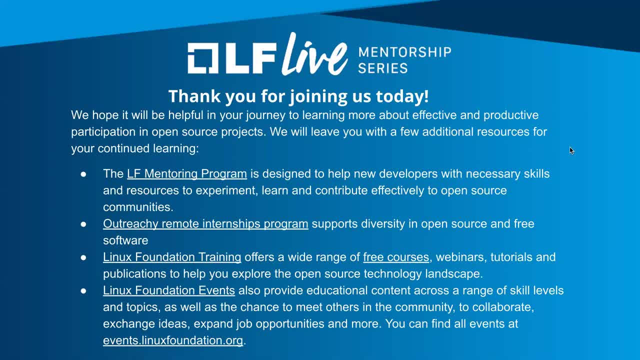 source software projects today. that is complete insanity to think you're going to be able to do that by hand today. there are a number of projects which which are different but share the same name. there are a number of projects which have multiple different names for the same thing. 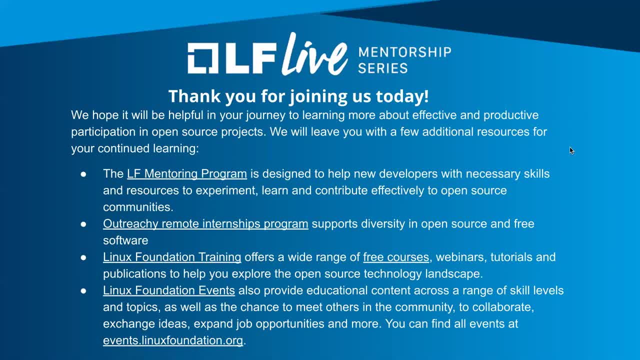 trying to handle that with a human is ridiculous. now the cve does attempt to do this with something called cpes, but they- but almost no projects- have cves today. they're not really supporting them. they keep saying they're going to use swids which don't actually work for this case. i don't. 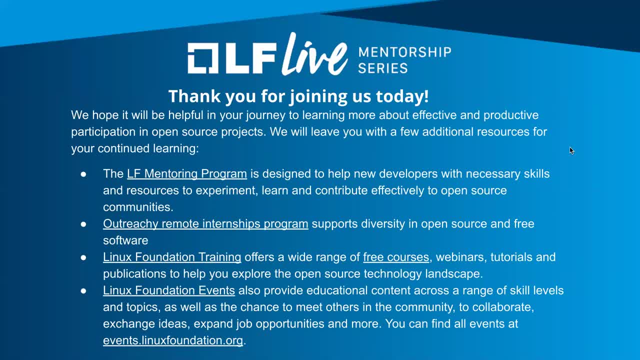 know why they keep saying that swids are going to work when it's known they're not going to work, because most of the software in there's open source and swids require unique hashes: uh for the x, for the, uh for the binaries. oh, by the way, you can recompile, that's a thing, so it just doesn't. 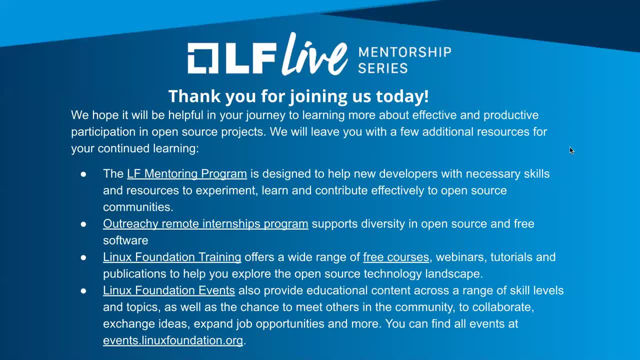 make any sense. um, so what are we doing to address? i think a number of people have repeatedly told the um cve folks, uh, that this is a critical thing to do. um, i think the reality is either the cve process is fixed to to address that, or that the community will abandon the cve process and switch. 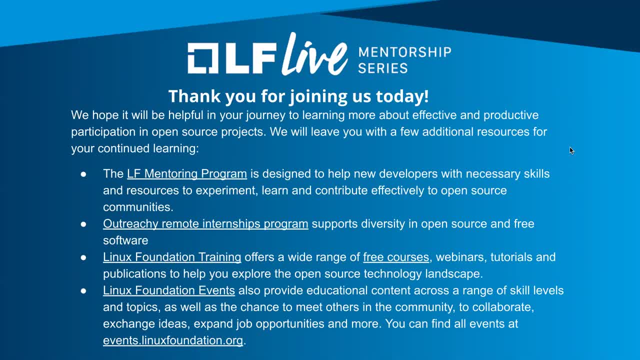 to something that actually resolves the problem. i'm kind of hoping that the cv- i mean it took a lot of effort for the cve folks to do what they did. i'm hoping that the cve folks will fix their process so that there can be an. 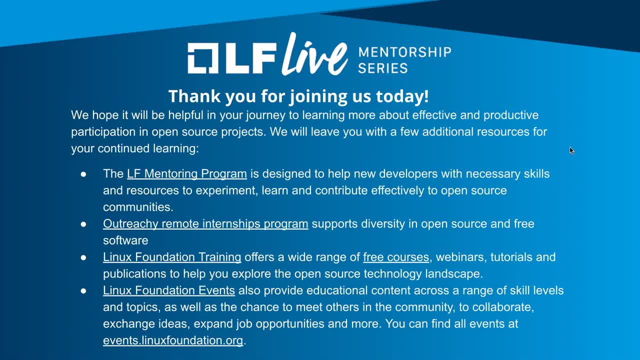 automatic connection, but in my mind there's really no point in reporting vulnerabilities without a way to connect it to the software that's vulnerable. it doesn't make any sense to me and it doesn't make any sense to a lot of other people too. um, i realize they do it with human. 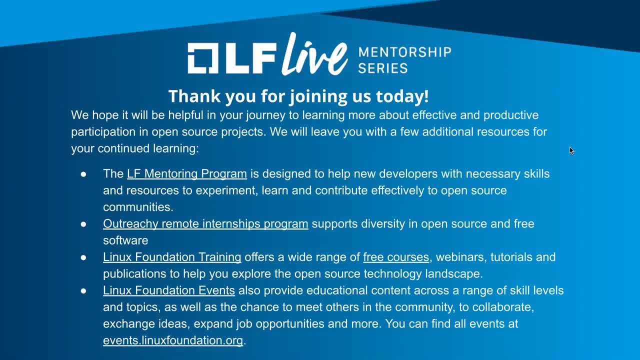 readable text that doesn't make. that also doesn't make sense in a world with millions and millions of software projects. so i'm hoping that they'll fix it. if not, i expect the community will come up with an alternative. um that actually resolves the problem. all right. 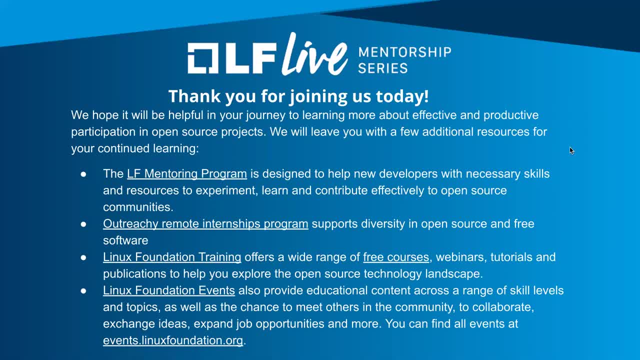 what do you suggest the learning strategy for the beginner? well, hey, i have an nx. i have pointed that nx course start there. um, it's not complicated, you click and learn. it's. it's a simple little reading materials, uh and uh and click on quizzes as you go along. it's not, it's not fancy, um, that's. 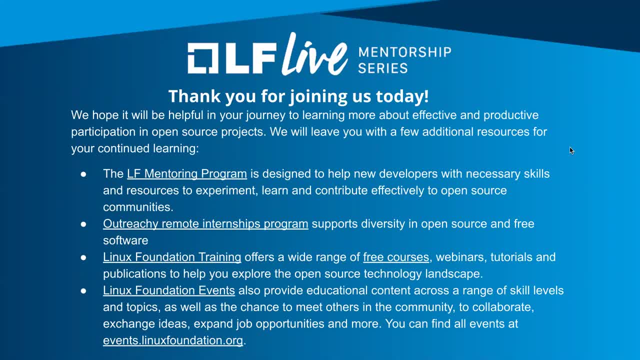 a good place to start. there's always something to learn. i've been doing this for a long time and there's always new things to learn. um, so start with you know simple courses like that, like that nx course, and then just be open to learning. okay, just keep you know, keep monitoring things. oh look, a new kind of vulnerability has been. 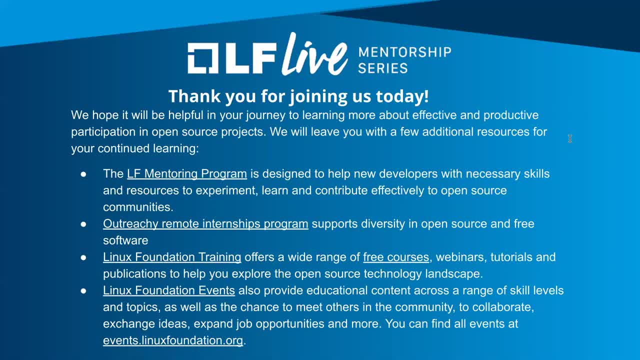 discovered. let me i'll read the article about that, okay, um, all right now let's see here. i think there's a. let me go. that was from the chat. let me go look at the uh, q and a. i gotta find where there we go- q and a. all right, uh, so i'm going to try to answer, open up the chat and i'm going to 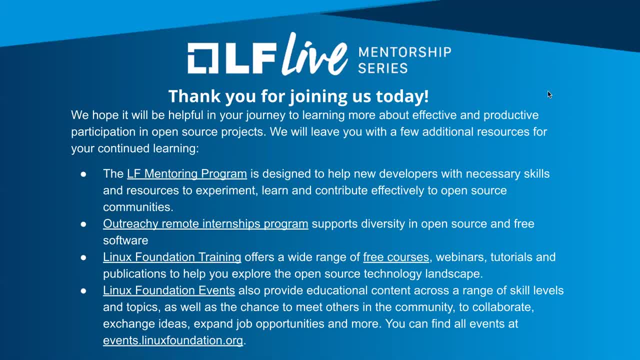 from the q and a sections. uh, what vetting occurs to prevent bad actors from getting involved in open source security and subverting these proposed improvements in some way? um the honest, the answer is actually the same is true for proprietary software. okay, which is you? make sure what you? 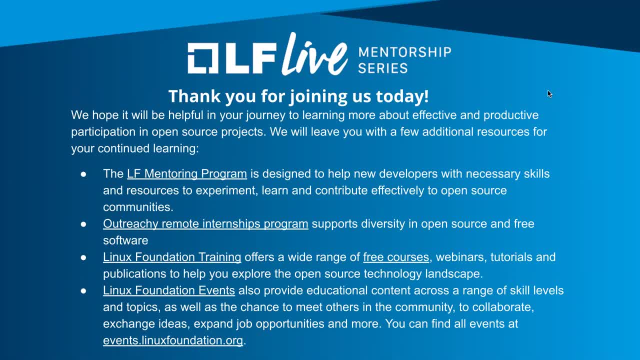 should be doing is having other people review that code, either before it's employed or afterwards, to look at the code to find those problems. and most the biggest risk is really open source software projects with single developers. in that case there often isn't a second person who can review it, other than maybe a reviewer a later. 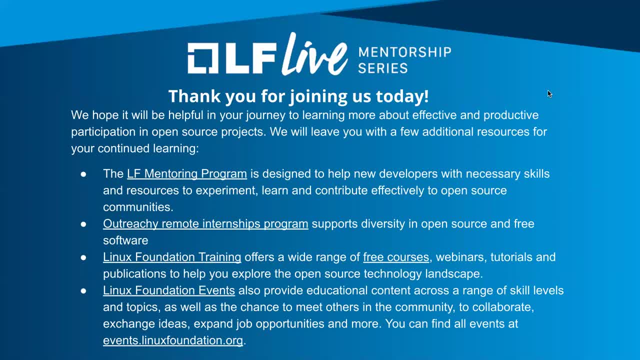 potential users who check, when the advantage of open source is that you can't. anybody, not just the developers, can look um. as the projects get larger, typically they start requiring more and more review by other people um, and so that makes it much more risky for an attacker to slip in and propose um uh, subverted, uh, improvements. i'll note there. 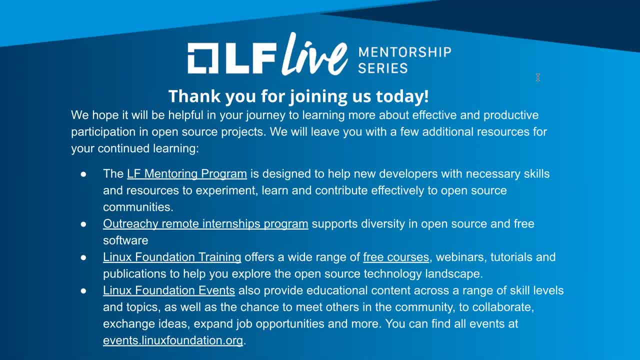 actually have been some efforts to insert malicious code that don't. that haven't worked um. somebody tried to subvert the uh, insert a malicious code, some malicious code, the linux kernel um almost 20 years ago- i think it was like 2003, i may not, the year may not be quite right, but 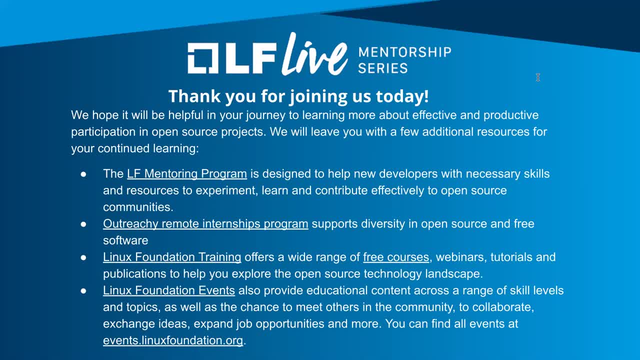 basically, they tried to insert code that looked right, but it used a single equal and instead of a double equal, a very- uh, subtle, hard to see flaw. if you weren't used to this sort of thing, um, that would quietly subvert, you know, enable someone to take over a linux-based system. 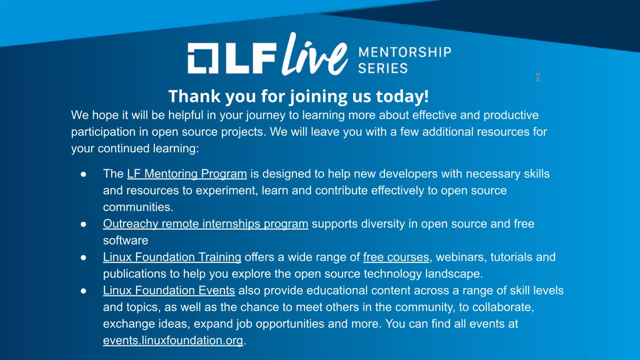 it was. that code was never included in a real linux kernel uh version. it was immediately detected by the kernel developers. uh, more recently some developed some um. researchers from university of minnesota tried to create some vulnerable code and tried to insert it, get it into the linux kernel um. the way they did it frankly was not appropriate. i'm not a fan of how. 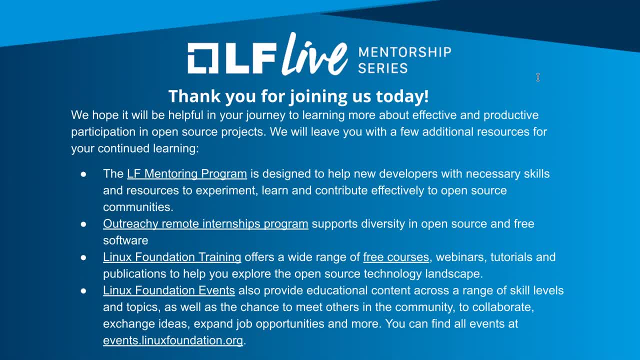 they did it, but you know what, since they did it, i will- we may as well learn from it what they did, and i'll note that, once again, their attempts to insert vulnerabilities were immediately rejected, uh, by the uh linux kernel developers. um, and so therefore, um, you know, all right. 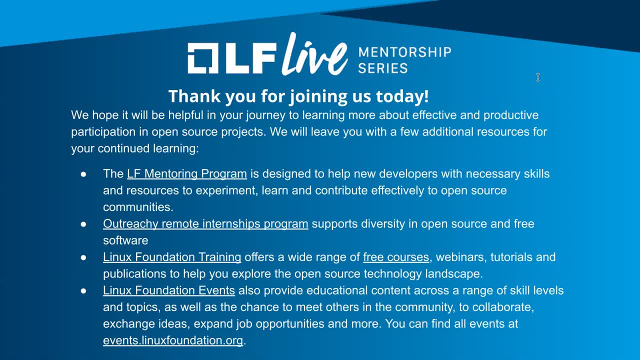 both those are linux kernel examples. let me add a third one. um, this is a very, very different one also. uh, years ago borland sold a? uh proprietary database program- uh, for years and it and they had some success in the medical community, but eventually it just wasn't. 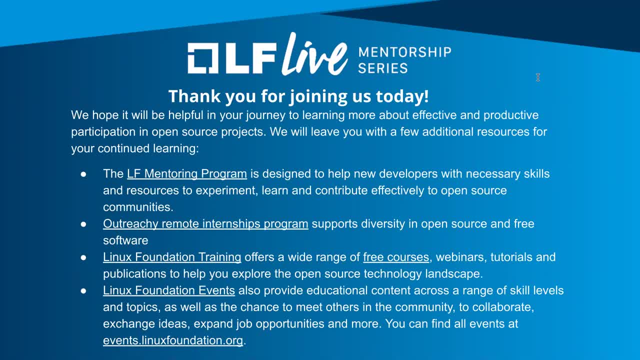 profitable, and so they decided, after many, many years of releasing as a proprietary program, they decided to sell as a proprietary program. they released it as an open source software program. um, within less than a year, um months, i don't remember exactly how long- um, someone found um, uh, a, a subversion that looked 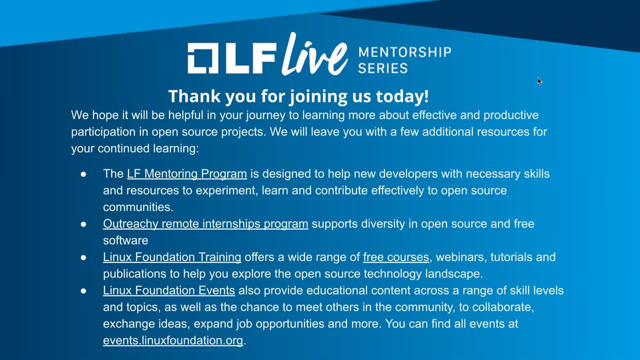 for all the world, like a maliciously subverted um uh backdoor. basically, if you entered your, the username of politically and the password correct, uh, you were suddenly the database administrator. this was not documented, in fact, was, of course, a very, very bad idea. now, maybe this wasn't a very, very bad idea, but it was a very, very bad idea. 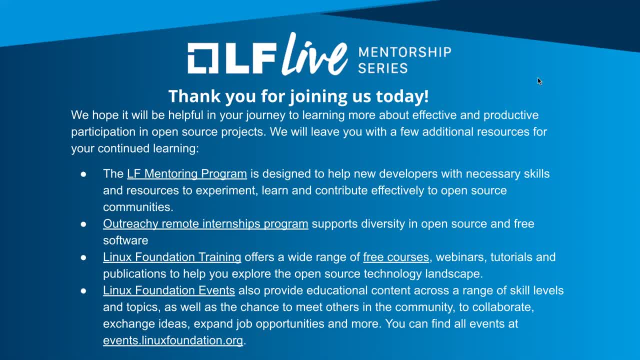 it wasn't an intentional, uh, malicious back door. it certainly looks like one, though, and whether or not it was, it shows that, hey, it was sold as proprietary software for many, many, many years. nobody noticed. this back door is released as open source software. people noticed, okay, uh. so while that's no guarantee, that does at least provide. 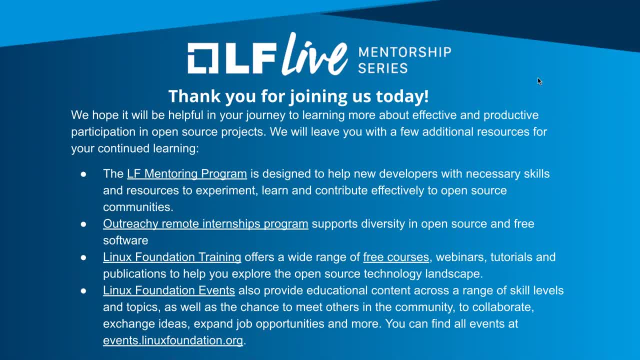 decent evidence that people really do look at code, open source software code, and they really do understand that. um, it's also a subject matter. um, you can look at code, open source software, online and you can look up your code and find the code on the web page and it's, it's, uh, it's. 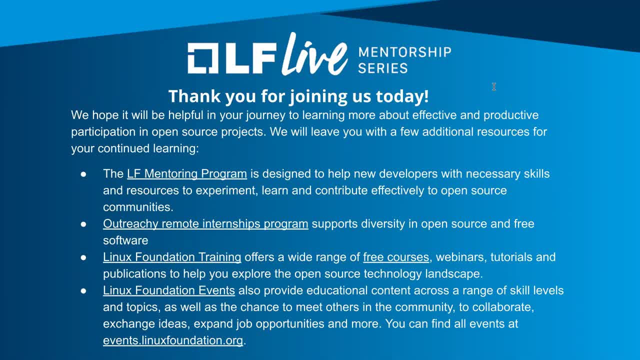 not a lot of data, and so, even if it's not like- uh, you know what i mean, though it's not very much of a um filter that can affect and counter problems, all right. next question: what language is the most vulnerable to attacks in developing open source software? oh, that one's actually harder to answer than you might think. um, let me, let me reverse the question a little bit, because i think, um, whoops, because i think that, um, i mean not in this particular question, or may not have had this line of thinking, but i have seen this line of thinking, but i have seen this line of thinking. so 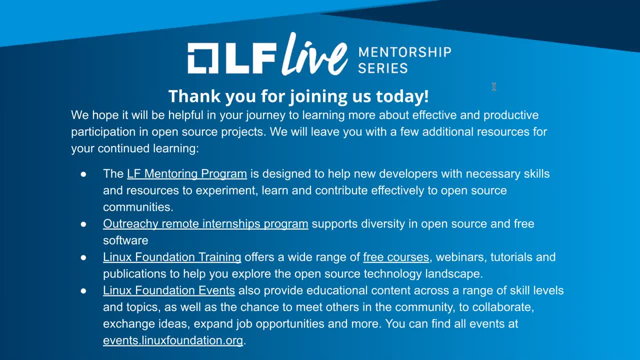 thinking where: hey, if I just chose language X, I will have no more vulnerabilities. And let me just cut that off right away. There is no programming language that ensures that there are no vulnerabilities possible of any kind. okay, It is always possible to make mistakes. 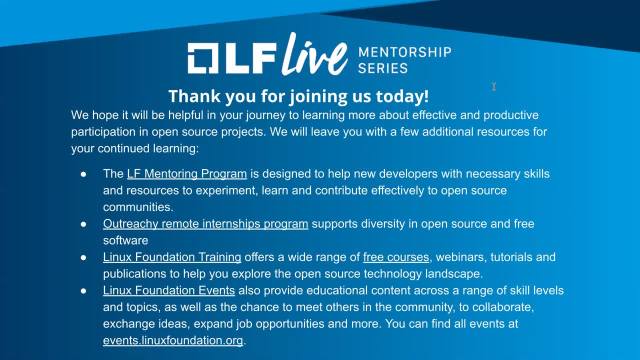 in any programming language and that result in what you didn't expect. okay. Now, that said, some languages do allow for a kind of foot gunning that is harder to do in any other language, I think, probably the poster child for this kind of thing, and I'm sure no one is shocked by this. 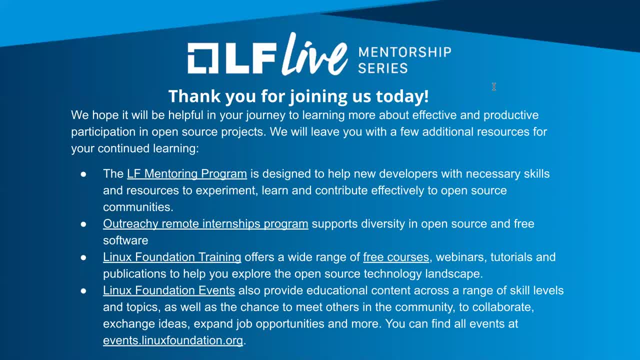 is the paraprogramming languages C and C++. They're not necessarily awful languages and they were designed for a particular circumstance and for a particular situation. The problem with C and C++ is that they assume that the programmer never, ever makes a mistake And the programmer is willing to take great pains. 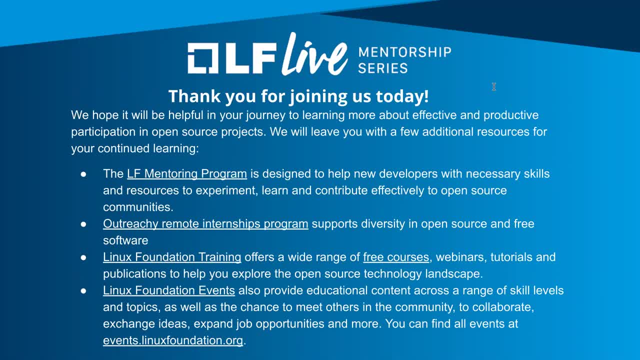 and care to check everything. So, hey, before you access an array, you're going to make sure that the array access is within bounds. If you read from a pointer or write to a pointer, that pointer is going to be where you wanted it to be, okay. It also assumes that the software 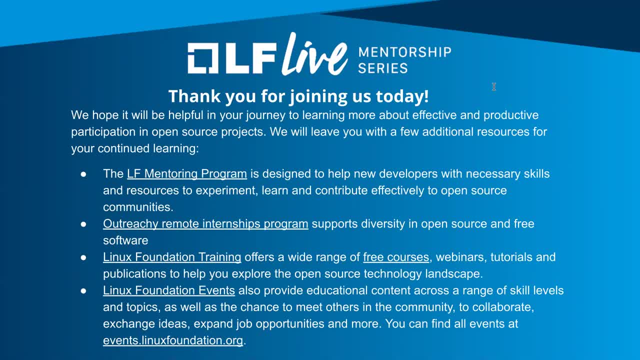 developer is going to be where you wanted it to be, okay. So that's the problem with C and C++. I think, of course, that's absolutely ordeonyo- The problems of vice versa. So I'm going to hear you wrap. 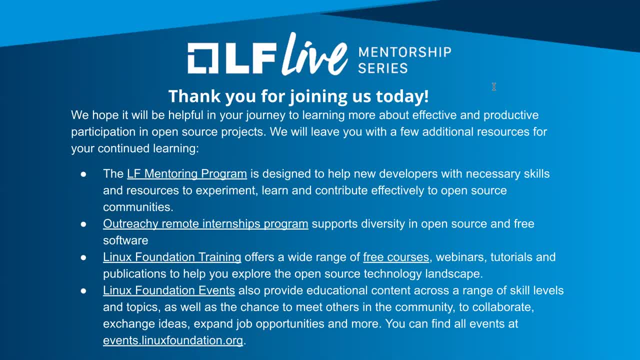 right around and make sure that we're looking at enterprise cartoon kind of type stuff, so that we're focusing on and thinking about ихind Pic, thinking about how we're going to address other Prayers, Which is we're going to get to atualize. what is a Python application? 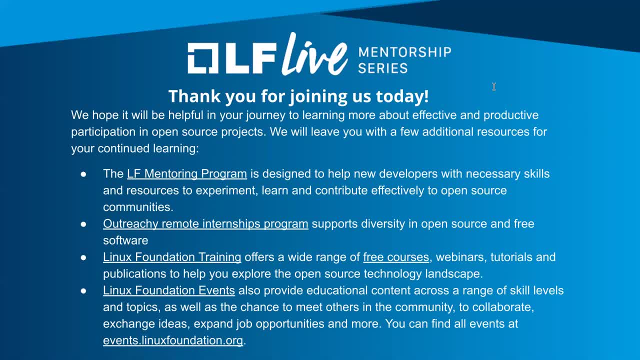 Sarah, what would you like to know about PC machine languages? Sure cool, Love it, Leroy. Very nice, Larry, in wrapping around, uh, but wait a minute, i thought computers did that. that's a machine thing you're using c. c has different rules and um, so i i think you know i mentioned earlier chrome 70. 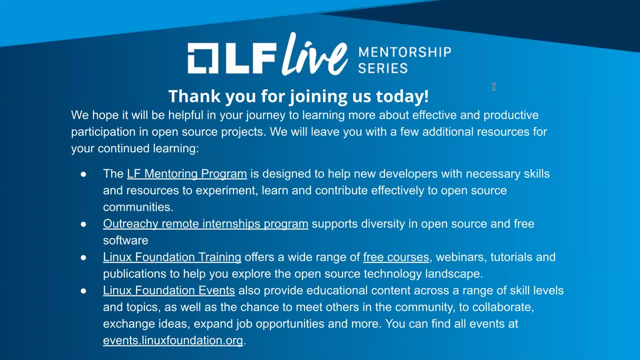 of its vulnerabilities. the last number of years, microsoft across its software 70 of their vulnerabilities are all due to memory safety issues. um and c and c plus plus are memory unsafe. always. all use of memory, uh, uh, uh. all use of scene c plus plus um always allows memory safety. 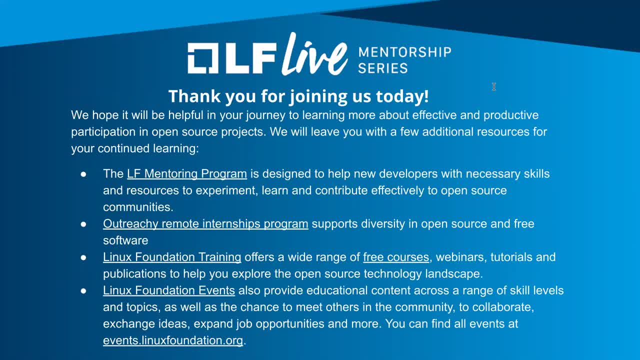 problems. there's no protections against memory safety issues built into the language. now it's true that some c plus plus classes, if you use them in certain ways, uh will protect against some memory safety problems, but in general but it's easy to escape out of and in fact it's easy. 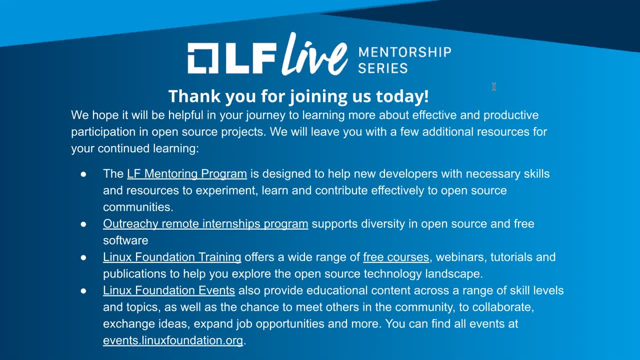 to escape out of them without realizing that you're escaping out of them. so, um, those are probably the most dangerous in terms of vulnerabilities, but, um many, many other languages. you can have vulnerabilities in any language. um, i mentioned earlier a push increasingly towards memory, safe languages, languages like rust, and so on. now, it's not that you can't have memory. 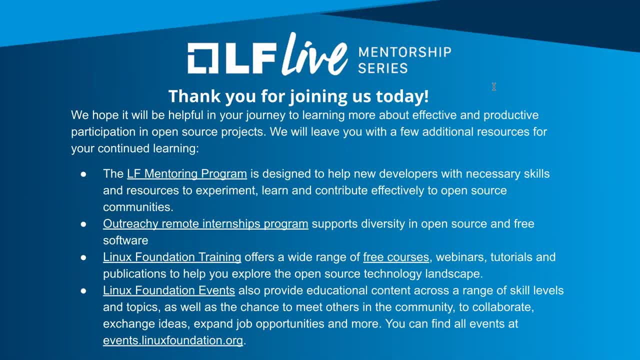 safety problems in languages like rust or ada or many other, or c sharp um. but the difference is that you have to specifically enable the unsafe behavior so there are safe normally and then you can disable the safeties and special cases when you need them. but as long as you limit the unsafe code to very small sets, you can check carefully. 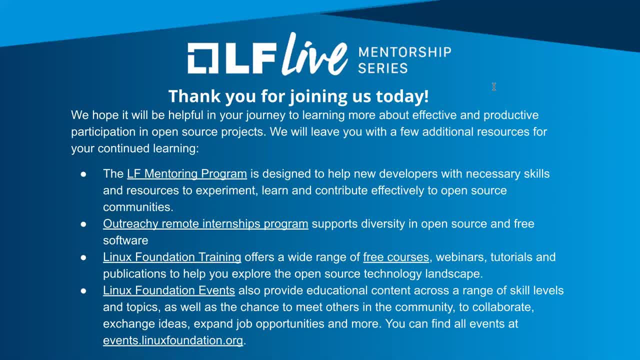 much, much less likely to have at least many classes of vulnerabilities? okay, um so. that said, can you have vulnerabilities in java? yes, absolutely. can you have many other language? absolutely okay, um so, but but there's, but, there's a trade-off and all too often it's. 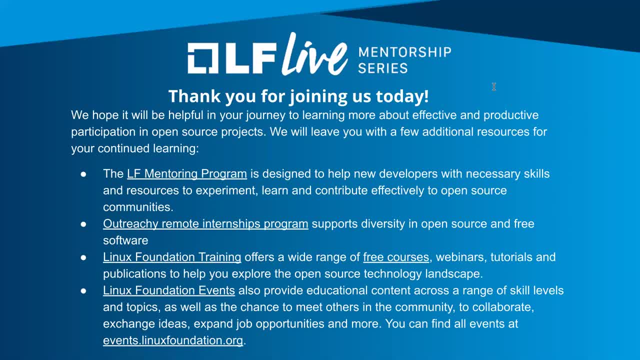 just too hard today for software developers to be perfect in every way, and that makes it harder to write secure software and scenes. a plus plus, not impossible, harder, right, um next, uh, let's see here what static code analysis tools do you recommend. what about dynamic code analysis tools? oh my, 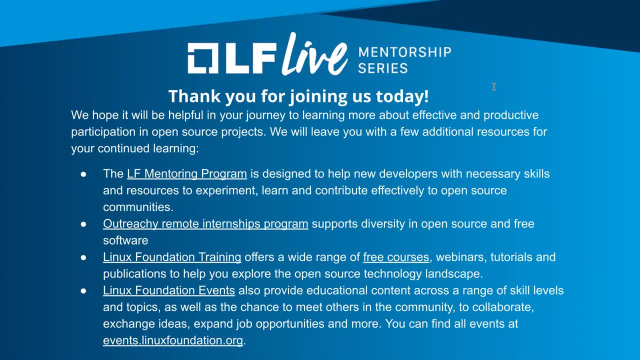 goodness, oh, okay. so first of all, i need to clarify that. um, you know, different tools are better for different circumstances. Okay, And so it's really not a matter of here's the one tool and off you go. Okay, Let me. so, that said, let me hit the dynamic analysis tools first. If you're doing a web, 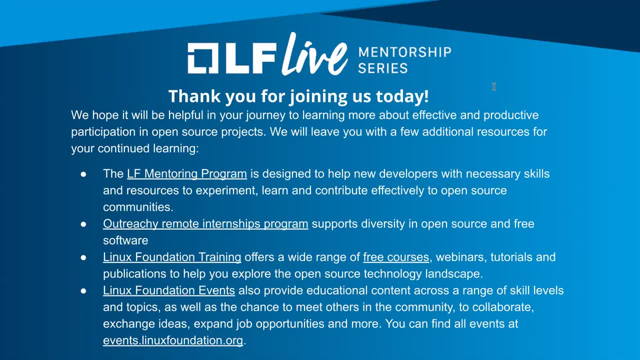 application scanner. there's a huge number of them and I'm not and it's hard to keep track, but I've used OWASP ZAP many times. I've been very happy with it. So there's one. Are there others? You bet There's a lot of good ones. If using fuzzers, there's tools like AFL++. 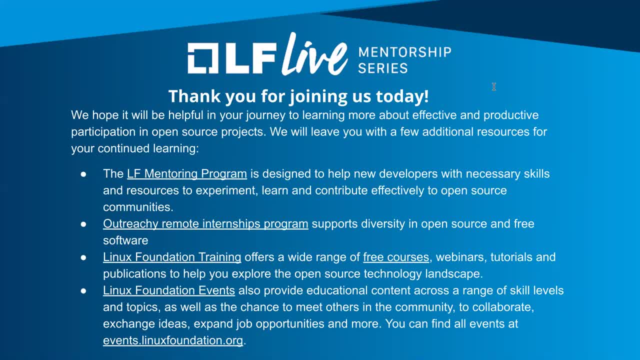 which is basically a fork- and a maintained fork- of American fuzzy lop. That's something called a coverage guided fuzzer. Coverage guided fuzzers are amazing. They have made it much easier to apply fuzzing without having to be really really. basically, they've lowered the barriers to entry. 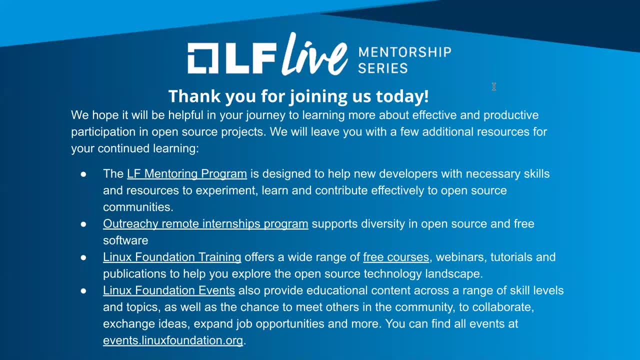 As far as static code analysis tools, that's way harder. Almost every language has at least one linter Use, at least one of those. As far as static analysis tools, that's really challenging And a lot of it depends on the languages that you're using. I know a lot of folks use Coverity. 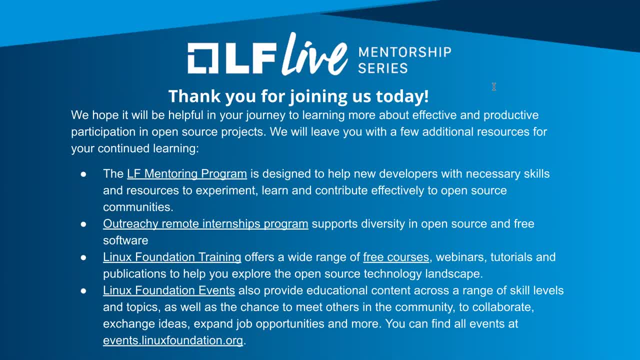 which is a proprietary tool, or Fortify. There's also just a boatload of other tools. Now, one complication that I should also note, that makes a little little bit challenging for me to recommend tools, is that some of the proprietary tools come with something called DeWitt clauses in their licenses. I am very much opposed to these things. 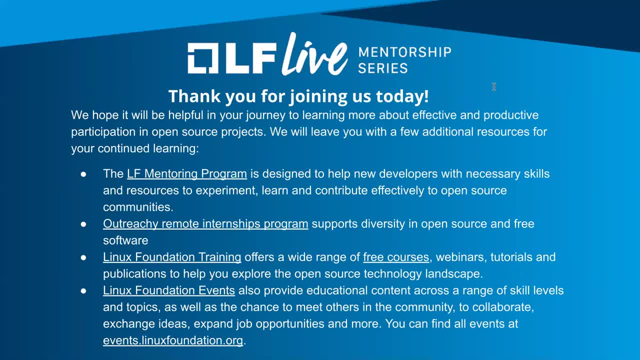 DeWitt clauses I think should be straight up illegal. But basically they say that if you're going to use the software, you can't publish results publicly unless we approve. And of course the toolmaker is not going to approve anything. that doesn't say the tool is wonderful. 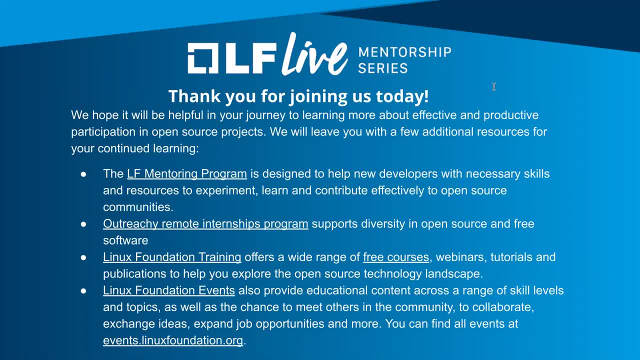 And so it's had an incredible chilling effect. I believe that these should be just straight up illegal. There's a lot of other free speech laws in the US that prohibit these kinds of things. Somehow this has flown under the radar. 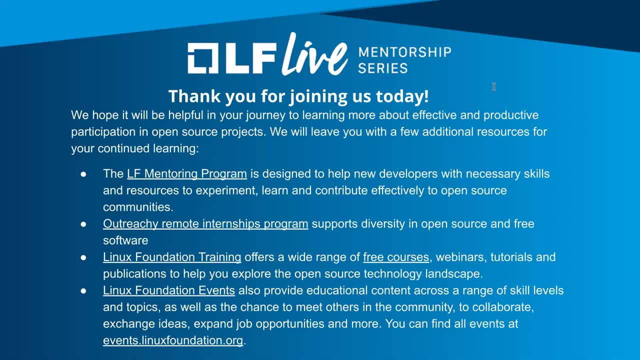 And once one supplier adds a DeWitt clause, other vendors are typically pressured to add clauses to their tools too, because otherwise people can talk bad about their tool but not their competitors. It's a bad situation, And it makes it harder to honestly give you recommendations, because 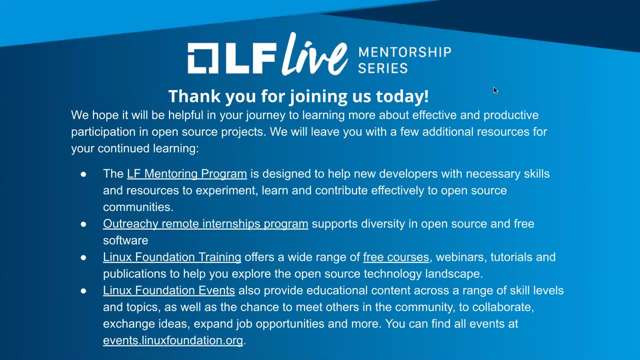 what I really need to do is go grab benchmarks that people have done that are published, And it's right now very, very hard to get that kind of data. So I've given you just some personal answers, But in the longer term, I'd like to see more and more tools and more evaluations public. 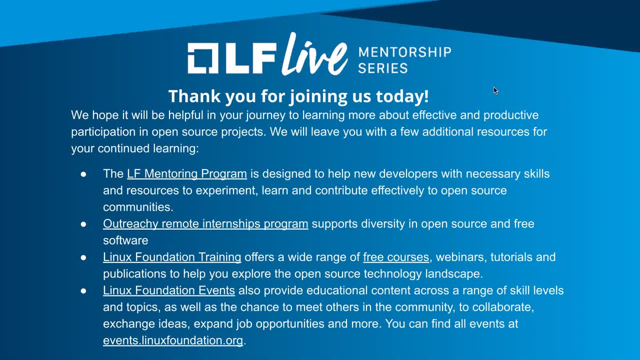 so that we can make a better evaluation. All right, how can you speak to how to best manage open source software dependency chain? today? If I evaluate widget X, how do I manage how to use gadget A, which uses gizmo B, and so on down to the bottom turtle? 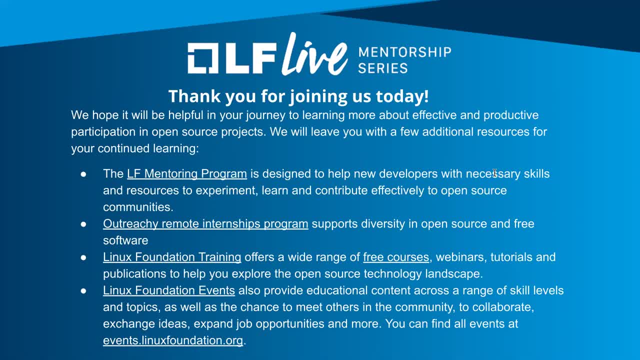 I know exactly what you're talking about. Yes, indeed, It's turtles all the way down. All right, It is something of a challenge. How can I best manage a dependency challenge today? Really, if you are developing software or receiving software, the number one thing you can do is look at the ingredients, what's going in, because you can compare those. 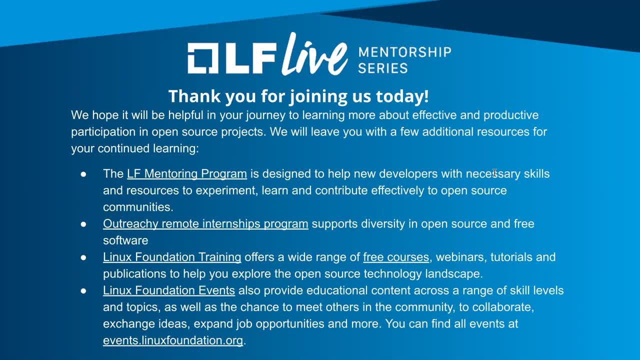 There are a number of tools that work to compare known vulnerabilities with the software and the version of the software that's actually in there. And you know what, If it's known to, If it's vulnerable, If it's vulnerable, complain and say, hey, wait a minute, you're depending on an old version, you need to update. 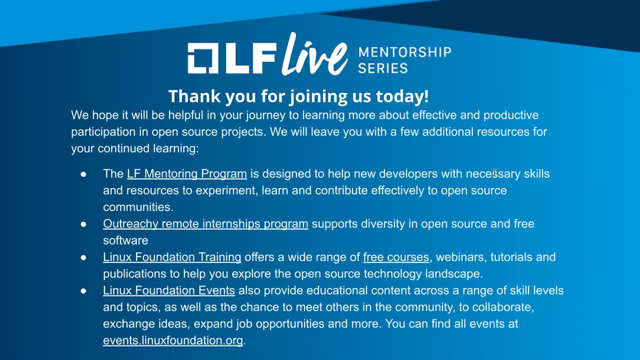 And I think right now, today, that's one of the key things- is going and complaining to your upstream. And you know what, If we weren't talking about software, if we were talking about physical devices with no software at all, that's actually how we would do it also. 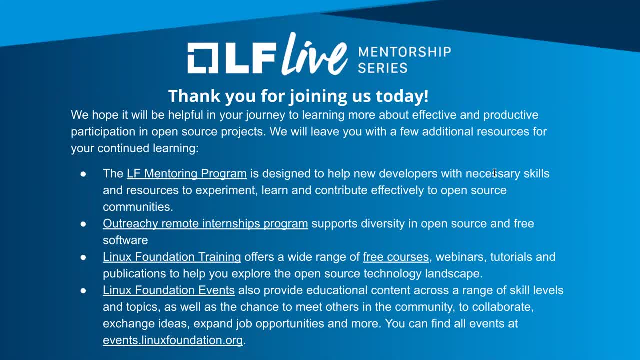 Okay, If I'm building a device made of other devices which in turn are made of other devices, You would look at your, At least at the major components, and probably look a little further to see if everything's okay. And if you saw a problem you would go and complain, you know, to your what's called the upstream. 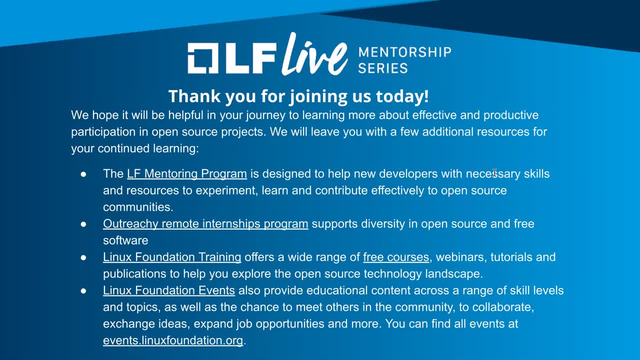 Think of things in terms of a river flowing down to you. You go to your upstream and say: wait a minute, the thing you're using in there has a problem. Go get that fixed, Get it updated or replace it. Do something. 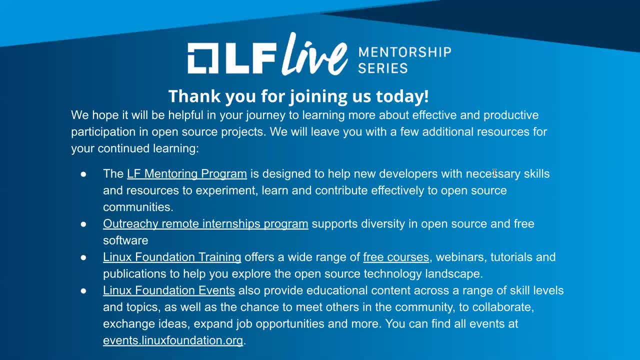 And really I think that's what's going to need. What we're going to need is more and more people, More and more people running tools, detecting problems, reporting back- say go fix, go fix, go fix- And getting people to start moving and updating. 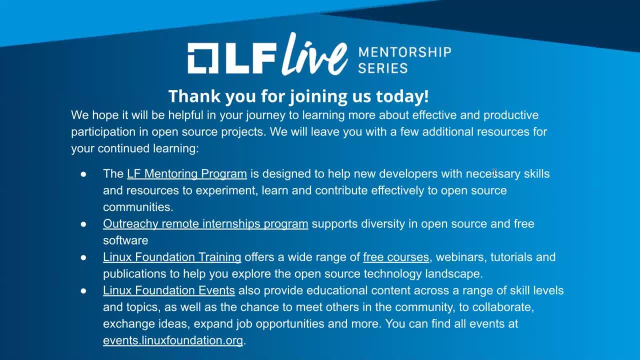 Because today the problem is often that a vulnerability is found, but somebody uses it, uses an old version, doesn't update, And then people who use it end up with this old, obsolete subcomponent. So it's not unsolvable, We just need to get people moving. 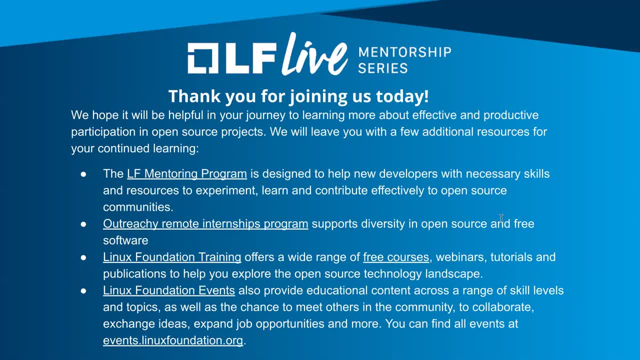 All right, Really great presentation. Thank you very much. What's the best way to do? responsible disclosure for open source software with a known vulnerability? All right, Let me see Just a quick side note, because you asked me a question. I'm actually not a fan of the phrase responsible disclosure. 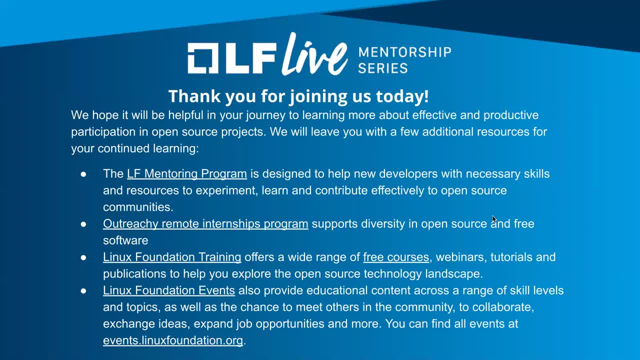 I prefer the phrase coordinated disclosure. The folks who originally coined the term responsible disclosure actually recommend using the term coordinated disclosure instead, Because it implies that doing anything other than that process is irresponsible, And I don't think that's quite true. Let's see here: 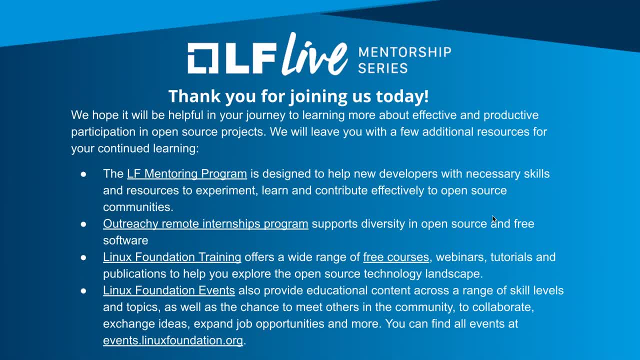 So, in any case, typically for coordinated disclosure, you report to the supplier, And I'm a fan of coordinated disclosure with a time limit, In other words, not just reporting but saying, hey wait, If you don't report to the world within some reasonable time and fix it. 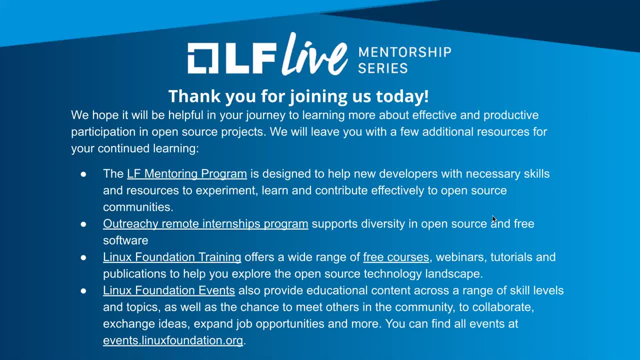 If you don't fix it within a reasonable time, I'm going to tell the world. Now, unfortunately, there's still a lot of- I'm not sure I should call them bad actors, but poorly behaved suppliers who instead will try to threaten you with lawsuits if you expose their problems to the fact that they have a vulnerability to the world. 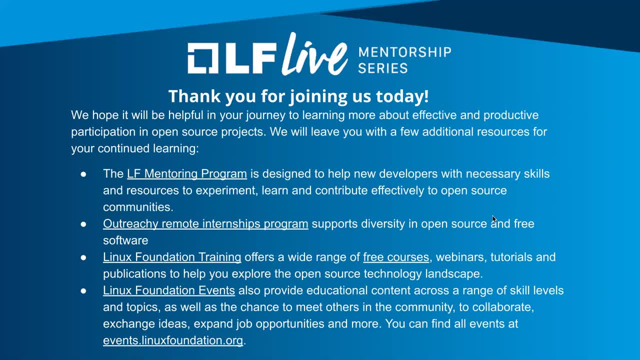 But you know what Too bad You wrote the software. You included a vulnerability in it. It's your job to fix it And you know, if you won't fix it, then I think the public has a right to know that the software that they were thinking about using is vulnerable and maybe they shouldn't be using it. 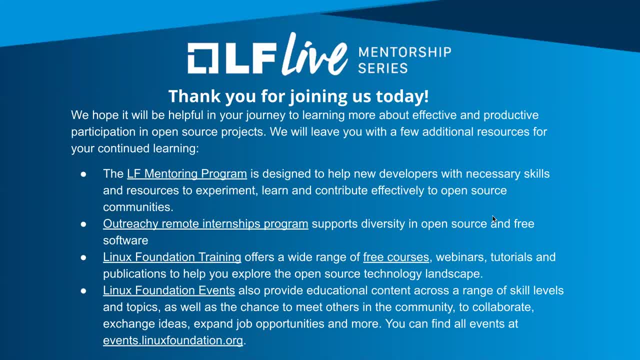 If you don't like that answer, then please go fix it. Ideally, start writing your software secure in the first place, To be secure in the first place. So what's the best way to do? disclosure To open source software. Well, the number one thing to do is actually not your problem, but the open source software project's problem. 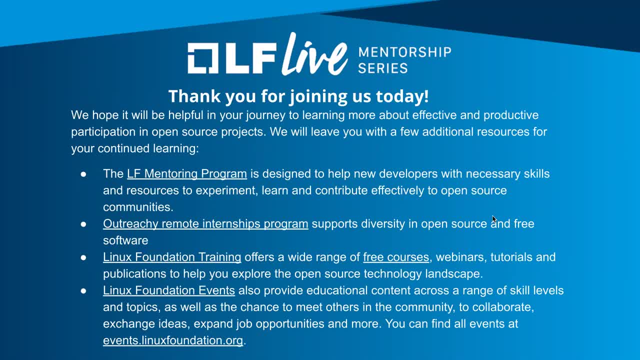 And that is the open source software project- should tell everybody how to report vulnerabilities to it. That is one of the CII best practices criteria. I'll also note that is one of the most commonly missed criteria, In other words, when a project doesn't get a passing badge immediately. 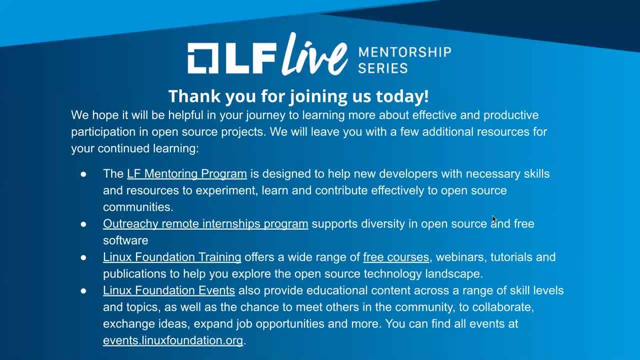 This is one of the most common reasons for it is: they haven't told anybody how to report vulnerabilities to the project, And you know there are reasons for it. I understand, But you still need to do it. So the best way is to go to the project page. 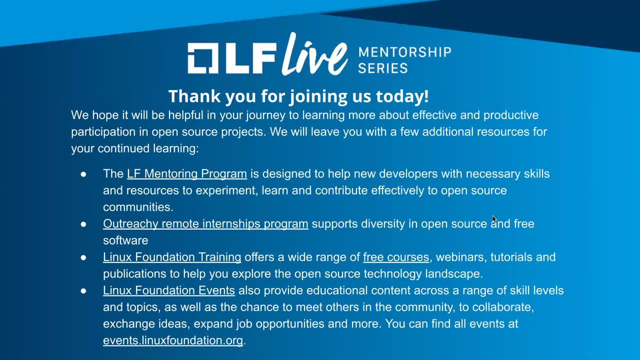 Notice that they have told you how to do it And then go report it. Okay, All right, That's a little bit of a cheat. What happens if I go to the project And, in fact, they haven't told me how to report it? 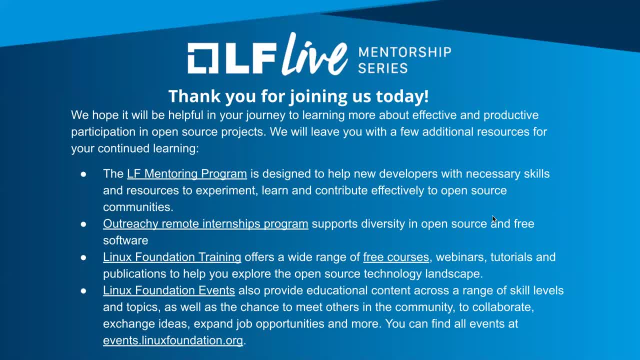 So what do you do then? Well, what you do is you go find a way to contact them. For example, if they're on GitHub, you can at least probably open an issue And say: hey, I think I may have found a vulnerability in your software. 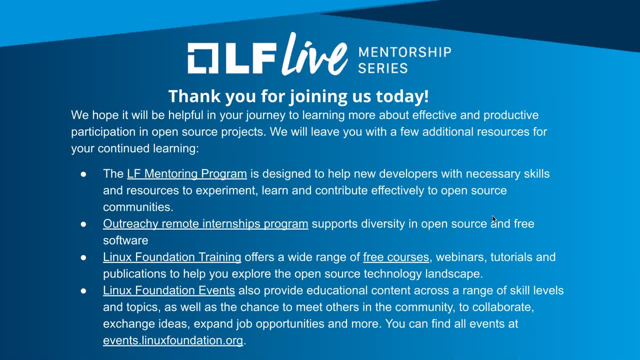 Please contact me, Give some contact info. Let's talk about this. In most cases, I recommend what's called a coordinated disclosure And in most cases, I recommend a coordinated disclosure And in most cases, I recommend a coordinated disclosure. In other words, don't reveal publicly immediately exactly what the vulnerability is. 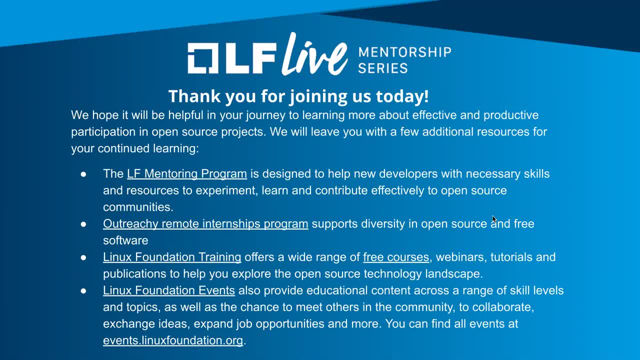 And the reason is that attackers will look for that information and will start exploiting customers immediately. Well, customers, People who are using that software right away, And you know that's not fair, because the users of that software had no reason to know there was a vulnerability. 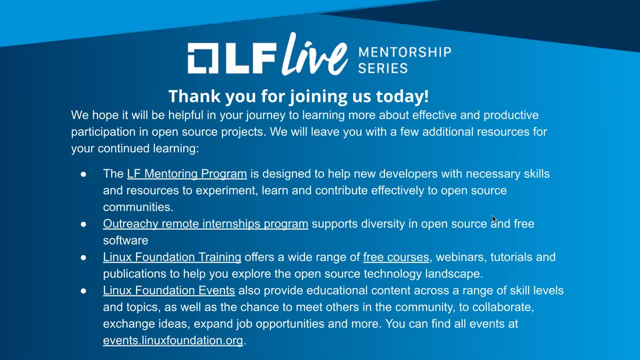 And it's going to typically take some time for the supplier of the software to create a proper update And fix it. So it's often best to try to do this quietly. Now. when is that not true? Well, sometimes that's not so true. 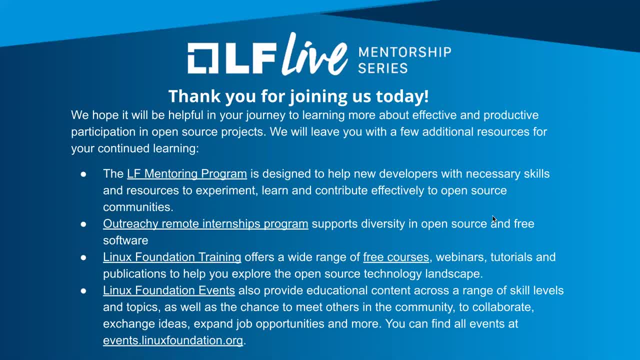 For example, if all the attackers already know about the vulnerability, it may be the only organization that doesn't know about the vulnerability is the project. Maybe the secrecy isn't so important. Maybe what's important now is getting it fixed well and quickly. 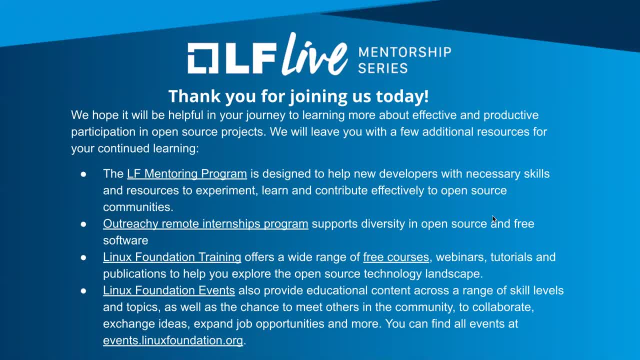 But really I think right now is: find a way You know, identify. Find a way. Ideally, use whatever process they have for reporting. If they don't have one, quietly ask them, Create one and coordinate so that you can report the vulnerability to them. 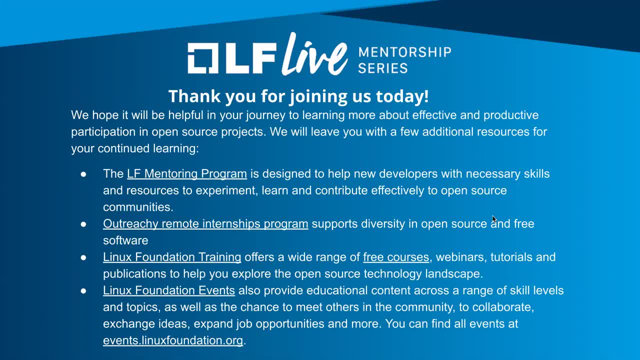 Give them a time limit. You can negotiate a time limit. There's various discussions on what a time limit should be. A lot of suppliers think the time limit should be really long. A lot of people who are potentially vulnerable, who are possibly impacted by these vulnerabilities, want them very short. 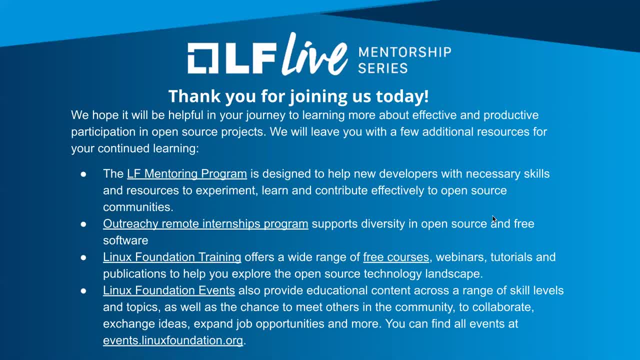 But you know, a lot of these things can be fixed in a week or two weeks. 45 days on the outset and the outside, You know, some will even give up to 90 days. But you know, basically, you know, try to create a timeline because otherwise it's easy just to let these things go on and on. 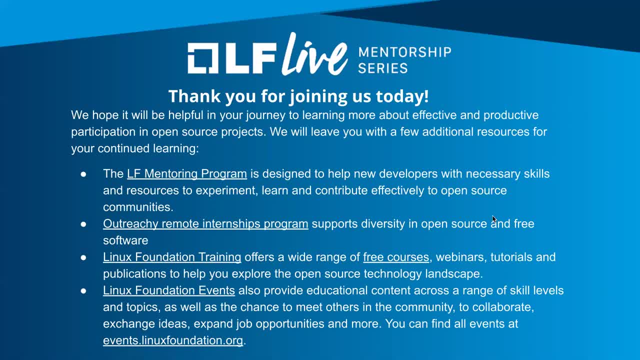 And the problem with that is, of course, with that no deadline and just going on and on, eventually attackers are going to start exploiting it. Attackers may find it independently. Heck, they may have already found it independently and are already exploiting it. 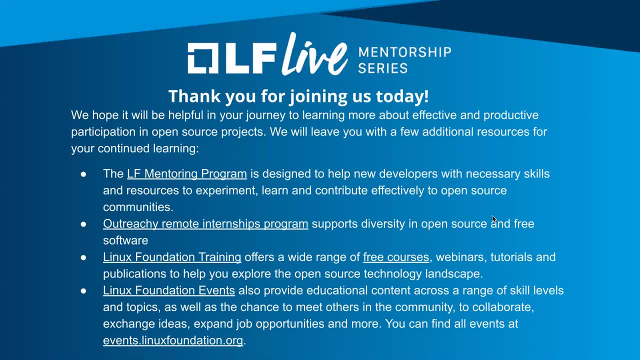 So once a vulnerability is found, it needs to get priority. Well, if it's an important vulnerability, it needs to get priority. attention get fixed Now. if it's a low level of importance- in other words, things like this almost normally never matters. 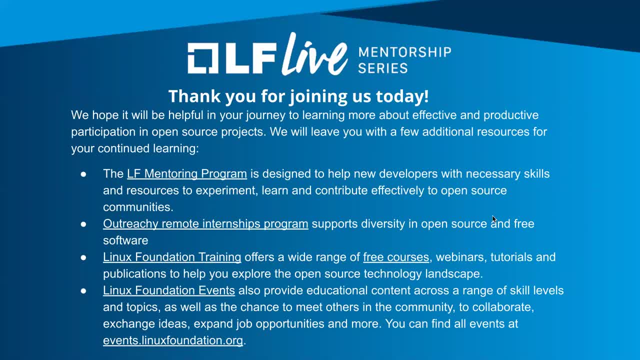 But in this really quirky, weird edge case, edge use that most people wouldn't be doing, it could be exploited. You know, maybe, in terms of You know, it could be shut down. you know not, you know, not revealing any data, just you know, maybe it's a denial of service and an incredibly weird edge case. 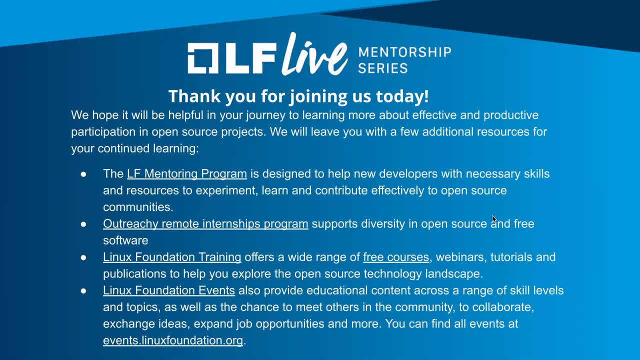 Maybe that's not so important And maybe you can give more time for that, But for super important vulnerabilities, you want to get them worked out quickly, OK, so I'm hoping that answers that question. I'll note that the OpenSSF actually has another group, the Vulnerability Disclosures Working Group, where they're discussing things like that. 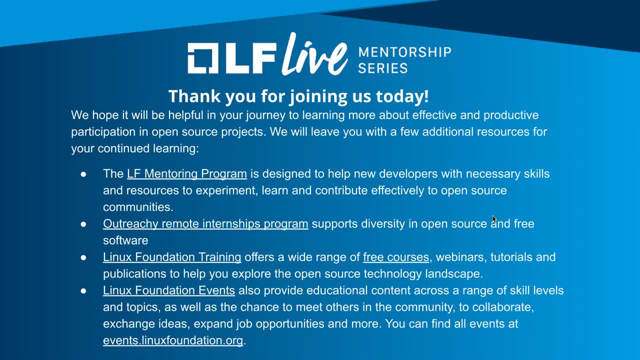 And there's also other groups like that First and so on- that have some information about how to report vulnerabilities and vulnerability process processes in general. OK, let me go to the next question. I have a project with a lot of depend about. updates have stacked up. 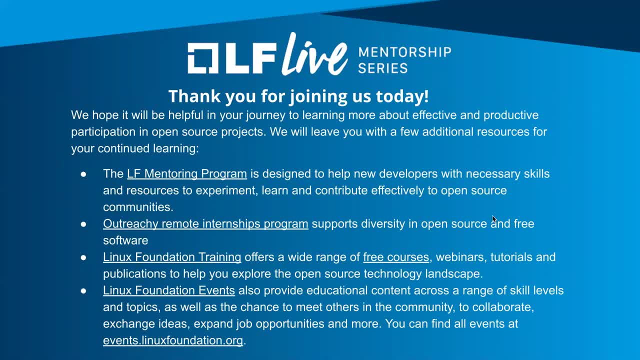 Some of the updates are breaking to the existing code. Oh, how do you recommend updating the code? Oh, my goodness. Well, I suppose I could just say carefully and leave it at that. But that's not really fair, All right. 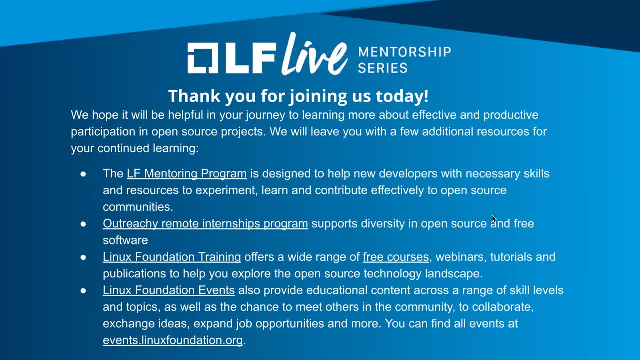 Well, first of all, You have my sympathy because I've lived that that joy many, many a time, So actually. So let me quickly go on a hobby horse. I mentioned this in my presentation earlier. If you are developing software for use by others, you should be ashamed if your API changes in ways where you're making it hard for your users to update. 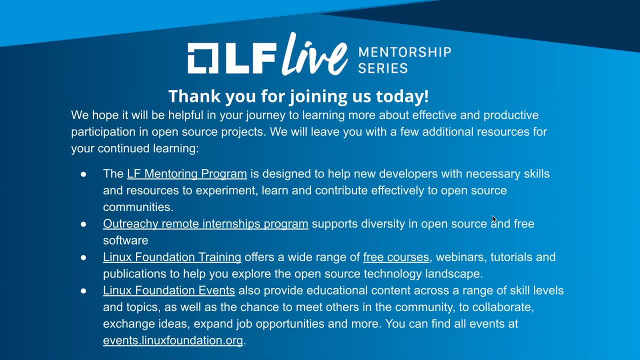 Oh, my goodness, I misspelled the old interface. Great, Add the new, correctly spelled. Keep the old one around. Why does it matter to you that it's not, But my API has five interfaces instead of four. How about that? 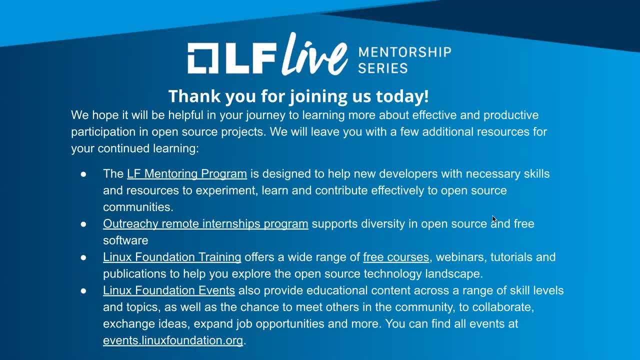 Why don't you think about the users for a change? OK, for the user's point of view, anything that is a breaking change is a big deal, because, oh, they just have to rename something or they just have to restructure some code. 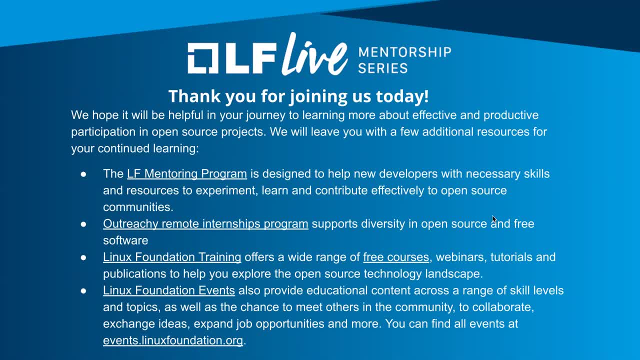 Most people have Other things to do with their lives than dealing with your API nonsense. OK. so please, please, please, try to make it so that software you develop for others isn't just break, isn't breaking, or at least not breaking often. 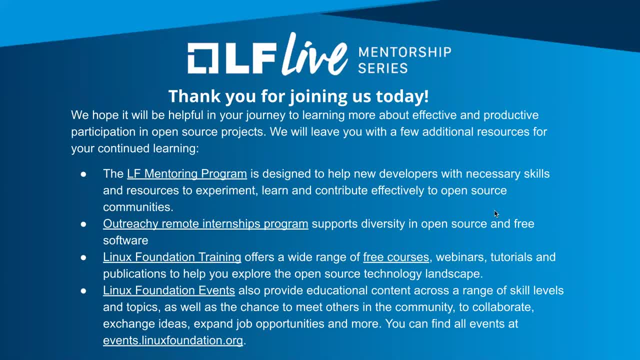 OK, try to avoid it. Give people lots of time to update. Sure, There are cases where you really just have to do a breaking change. OK, give the morning. Make it as easy as possible to update. I know the Python three folks thought, oh hey, the Python two to three is easy. 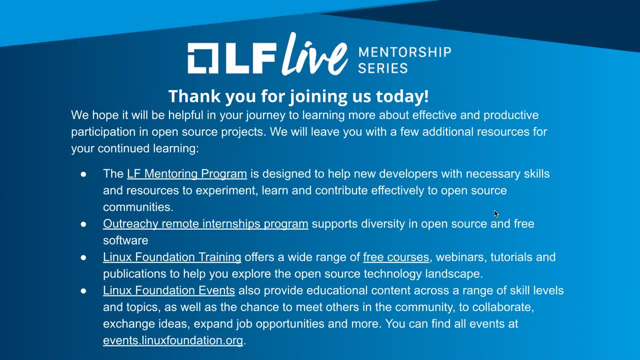 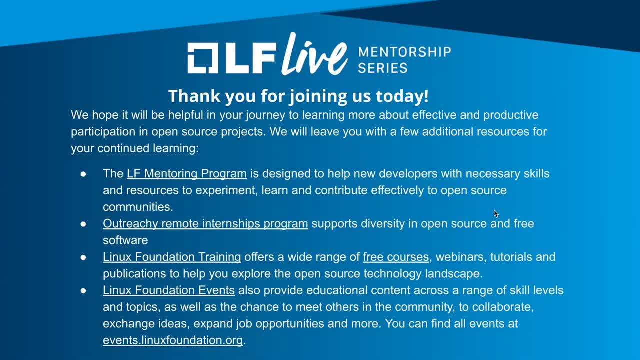 OK, be good to them, not malicious to them. All right, So, but you're not. You're, unfortunately, the other circumstance: Some of the updates broke your code. This is a problem. How do you recommend updating the code? I think in general, slowly, incrementally, you know, slowly, incrementally, one at a time, if you can. 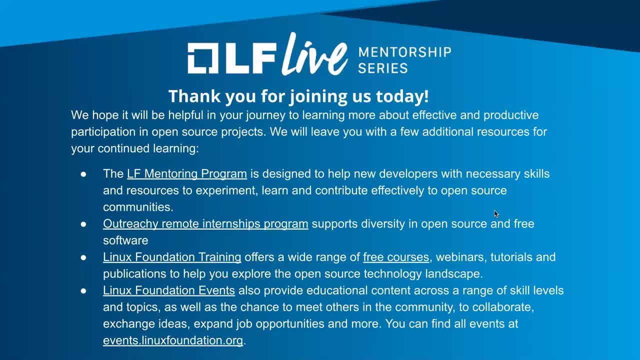 Sometimes that doesn't really work because you've got to upgrade things as a unit. But in many, many cases, what you want to do is upgrade very slowly And after every upgrade you run, You're, you're carefully, you're very thorough. automated test suite. 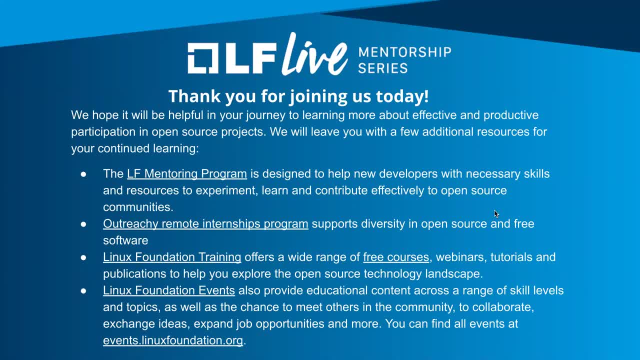 Oh wait, you say I don't have a good automated test suite. Well, there's your problem. Go get yourself an automated test suite. OK, It's not rocket science. There's lots of test frameworks out there And just you know, pick a testing work, write a bunch of tests. 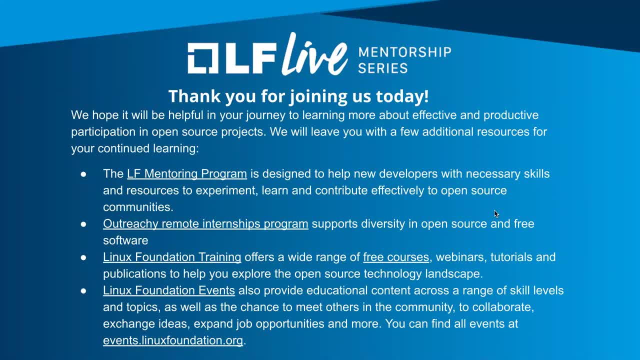 And you know, and once you have so on automated test suite. Now, every time you can update, you rerun your test suite. Is it good? Is it Good, Is it not good? You run an update. Oh man, everything broke. 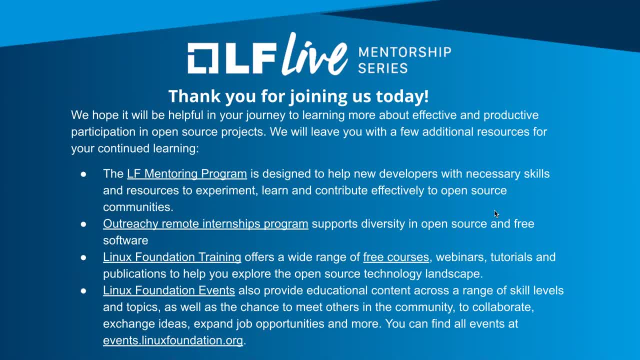 Okay, or maybe it doesn't even compile, All right. well, at least you know what to fix. But you want to try to make each of those changes as small as you can and then use your automated test suites to help make sure that, yeah, it doesn't complain immediately when I update, but does it really work and do what it's supposed to do? 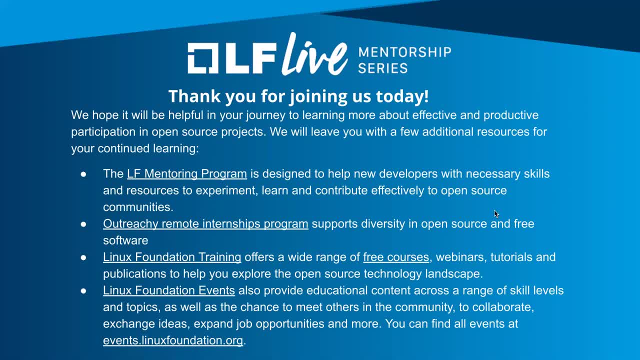 Okay, an automated test suite lets you do little tiny increments, update over and over and over again, And package managers also help you because they make it easy for you to say: see that, update it to this version. Do it just one at a time. 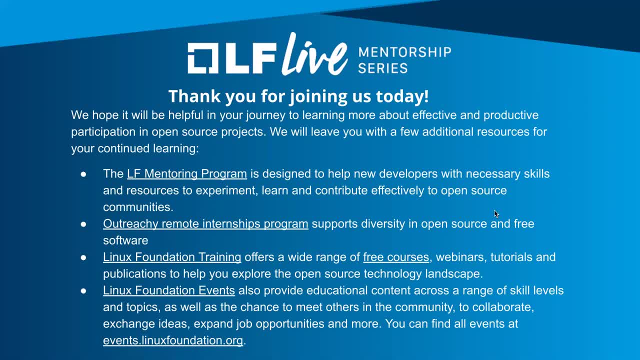 And typically you don't want to update. you want to update incrementally, not just in terms of small number of packages update, but small version increments. If you're using version 1 and version 20 is out now, it's likely you might want to update that version to 2 to 3 to 4, or maybe 1 to 5 to 8 to 12.. 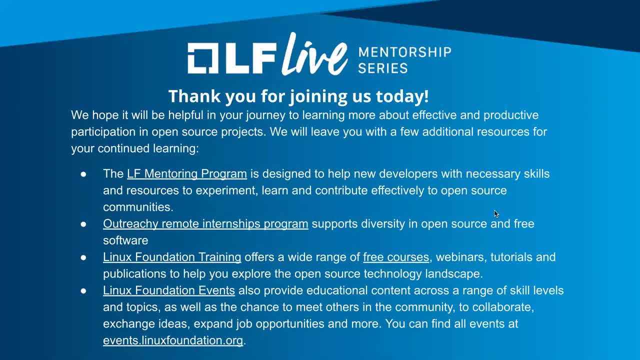 You know something like that. Okay, instead of just trying to do a big jump 1 to 20.. Okay, oftentimes projects will do things like, for example, they'll have backwards compatibility layers and things that warn you: hey, wait a minute, you need to change it to this way. 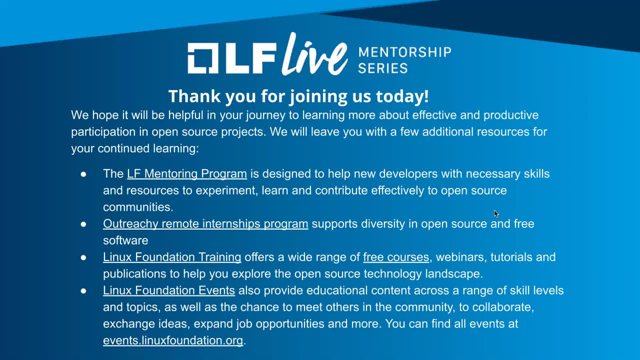 So if you have to change something, if you change more slowly, if you change the version numbers in a more incremental way, you're more likely to get help in improving, changing the software to be ready for the current And again automated test suites. 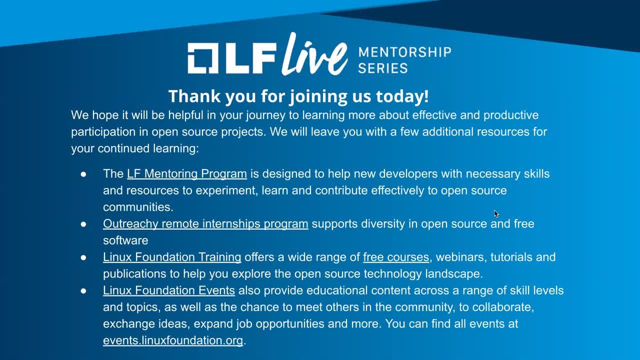 The great thing about an automated test suite is, once you have one those instead of saying, man, I got to change it all at once because I don't want to rerun my tests every time. Rerun your tests every time. 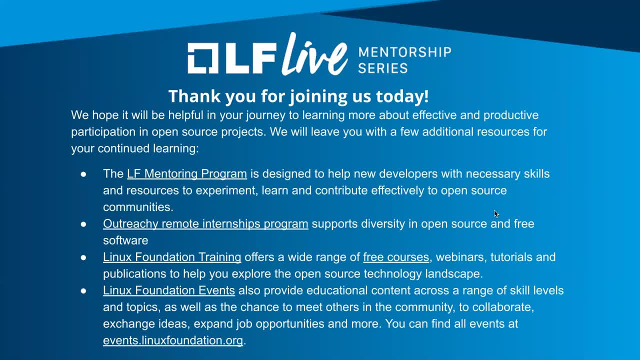 It's automated, Okay, And then you greatly, greatly reduce your risks of problems down the road And, frankly, you know- I guess this is probably obvious anyway, but I'll just say it- You know you may need to prioritize. 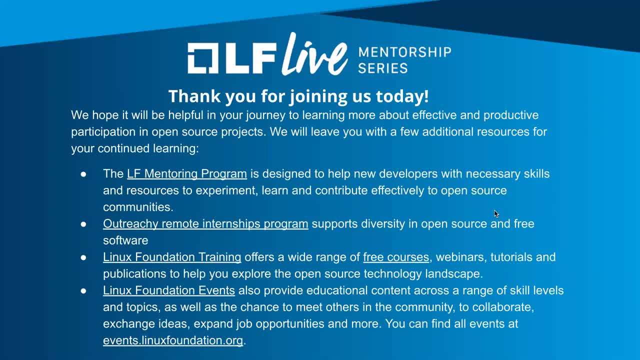 If you've got a lot of updates that have stacked up, some are probably more important than others or easier than others- Figure out what you want to prioritize and prioritize those. Okay, All right. So I think that's enough for that, All right. 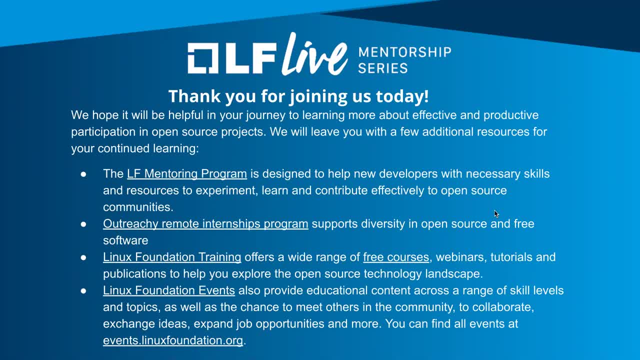 I'm trying to understand how open source software making money. Can you help me understand? This wasn't really frankly, we could have a whole presentation on just that. In fact, the people have. I've done whole long presentations on just that. 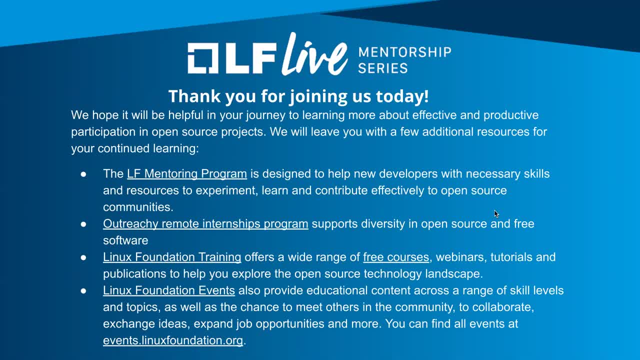 So I'm not going to be able to answer your question, to give it full justice. But let me attempt to do a quick answer. Hopefully it will at least give you a hand, And then by all means seek out longer presentations that really focus on that. 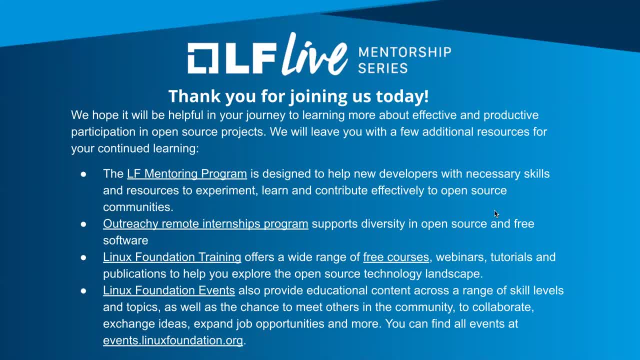 All right. So there's actually a lot of ways that people make money, And in a lot of cases, people are developing open source Software for reasons other than making money in the way that you're thinking about it anyway. So let me start by answering the question that's directly asked. 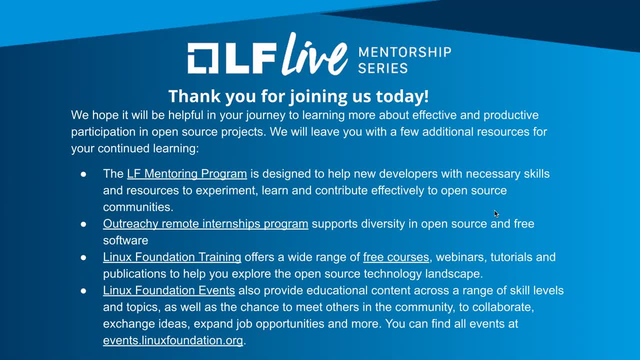 Okay, How do people make money Open source software? Well, first of all, a lot of open source software projects sell support or companies sell support to it. So, hey, you can use the software for free. And a lot of companies talk about in terms of funnels. 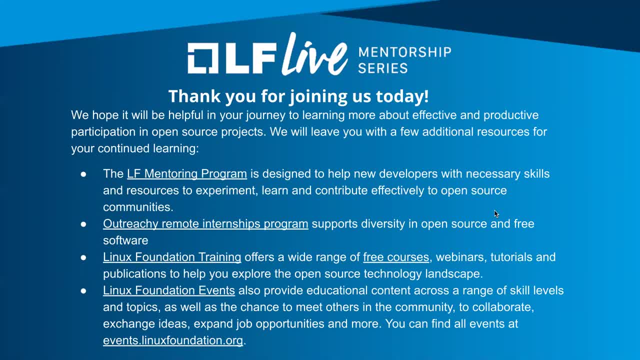 You can't sell services if nobody uses your products. So your first step Step is: how the heck do you get customers in the door? I'm going to give them the product for free or a low price And, once they're using the software, are comfortable with it. 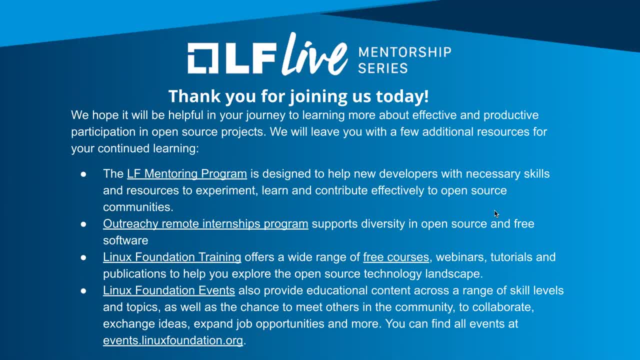 Oh, wait a minute. They want to use it, do it more with it, sell, support Some companies they have like the core is open source And then there are various additions that are proprietary, closed source, that you can use, But they charge. they charge extra for those. 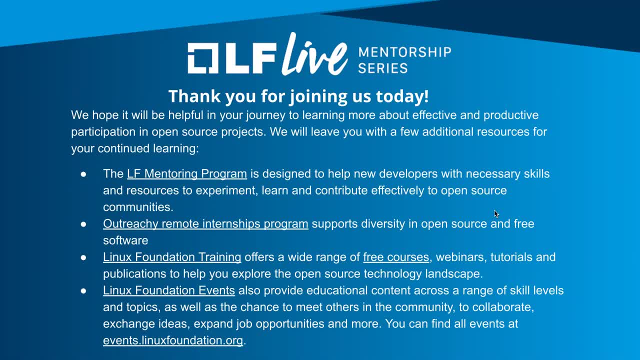 Um, Another thing to be fair is that, although open source software is often no cost, there's no requirement for that. That's not. you'll notice that my definition. that wasn't part of the definition. Okay, So people have and continue to sell open source software. 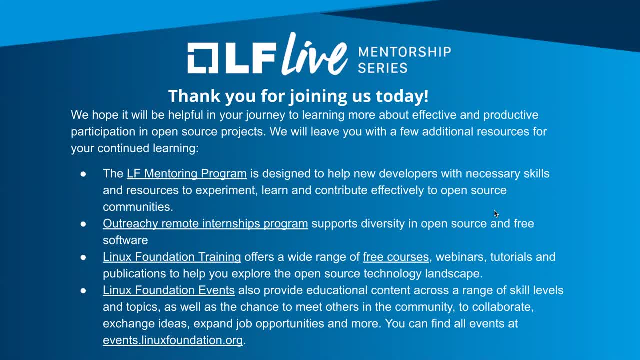 Um, now, that assumes that you're trying to make money just like typical proprietary or closer software vendors, But in fact, a lot of folks. this is not the primary reason for a lot of organizations, Um, Open, participating in open source software is a money thing, but it's not about making money. 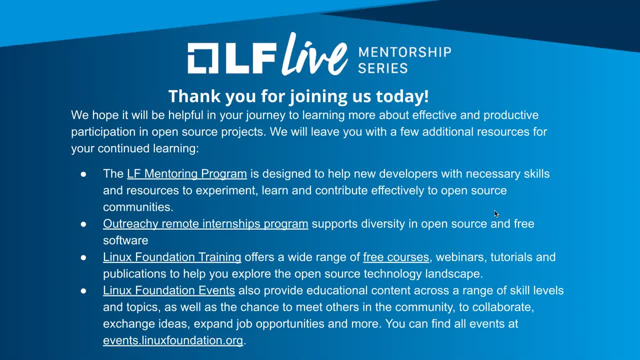 It's cost avoidance. You know, if you- hopefully you're familiar with- how profit is calculated: right Income versus minus outgo, right, Um. so you know, revenue minus expenses, Um. so basically, if you, if you can reduce what you spend, you end up with more profit. in many, many uh organizations use and support open source. 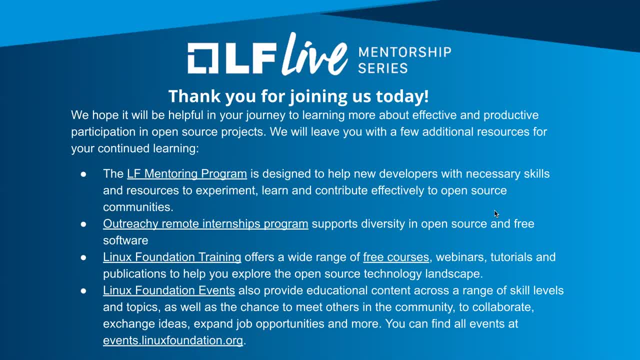 Um, so you know, if you can reduce what you spend, you end up with more profit. in many, many, many uh organizations use and support open source software because it's much cheaper than trying to develop the software themselves. Um, historically, if you look back, um you know, starting from the late sixties, early seventies, there were a number of suppliers who were selling various versions of Unix. 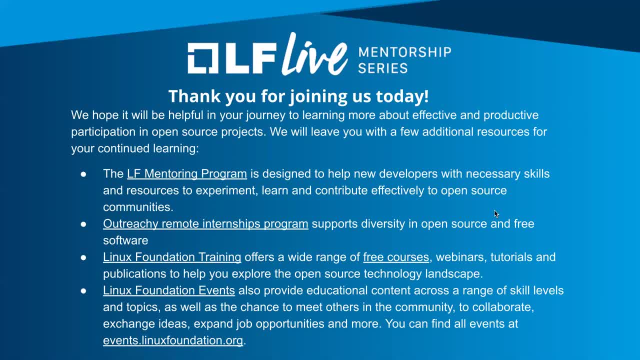 Um, and each of them, you know, would take some software modify, try to sell, And the reality was that it turns out to be really, really costly to do that. But if you, You can take a vast amount of open source software, um, and either use it and use it directly, or use it to sell something else, or use it simply to support your infrastructure. 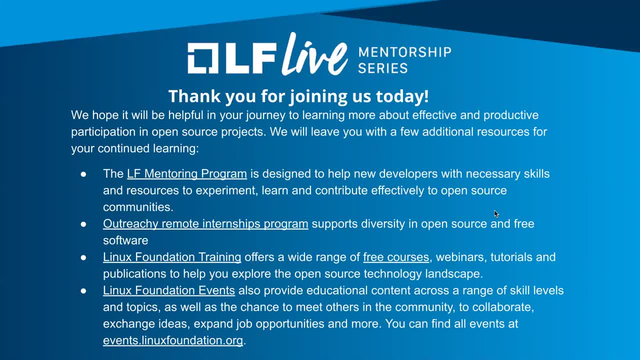 It's a lot cheaper than trying to build it all in house, Even if you have the capabilities. um, there's a um, you know, you, you, there's a lost opportunity If you use your resources to do that. when, wait a minute, here's some open source software. it's either does what we need or almost does what we need. 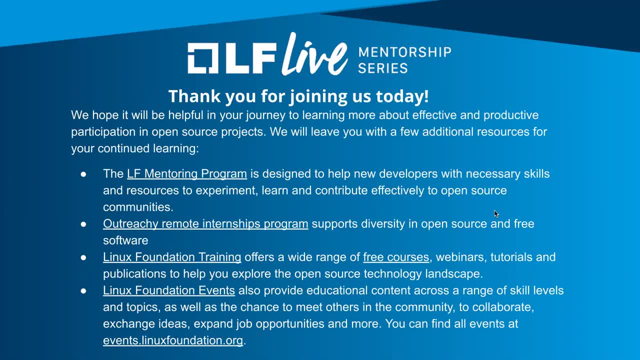 And we can make some small Improvements and make it better, And now we can use it for our purposes. Now, once a organization makes an improvement to open source software, they have a decision to make: Should they keep that improvement in house or should they try to release it back? 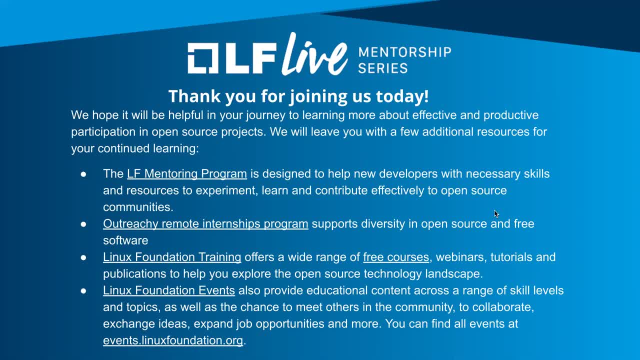 Well you would. you might think that, oh, keeping it in house is the obvious solution, but actually no. 90% of the costs of software are actually in the sustainment and the maintenance process, not in the original development. So for most folks it's a lot cheaper to get that improvement back into the main open source software project, because that means then they don't have to keep figuring out how to maintain it. 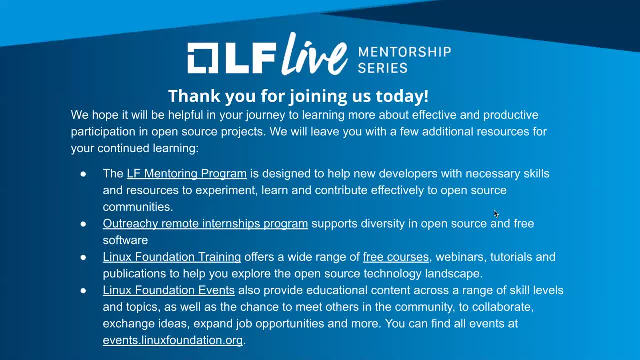 Uh, they don't have to keep trying to figure out how to make that work with other improvements that are being made to that software over time, And so, as a pure economic model, it is much cheaper for me reducing my expenses. Okay To take open source software, improve it, get those improvements. 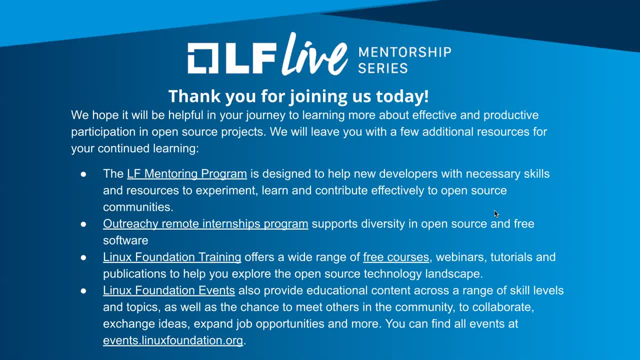 Back to the project, And now I have something that is far less expensive than, and possibly more functional than, what I might've done myself. Uh, and so for many, many folks, it's not making money, It's a cost avoidance. 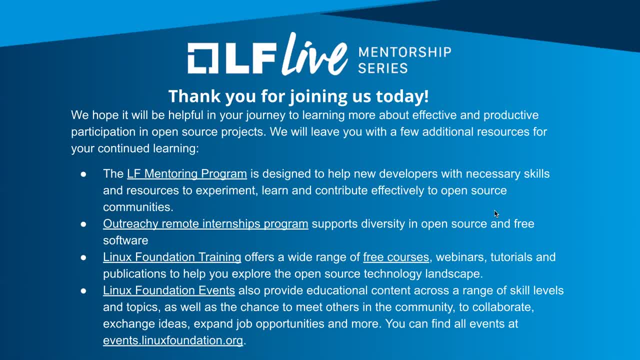 And I should honestly note a third, which is there are a lot of people who just like to write software. It's fun. And in a world where everybody seems to think that the only thing that's important in the world is making money, We sometimes forget that you know what humans are: humans and humans are awesome and humans like being creative and doing things like creating software. 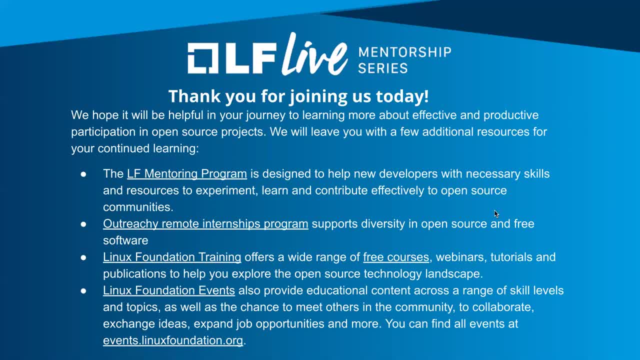 Um, and we should be grateful to those folks and celebrate these folks because they make some of the most interesting and useful software in the world. So those are three different and we can delve in further, but hopefully that at least gives you an answer to that question. 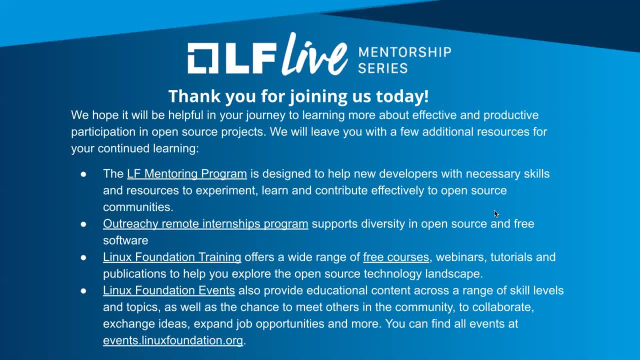 All right. Many companies prefer to use or reuse open source software. Don't want to share anyway, Isn't it In this case? how's the open source software? how the? I'm not sure in this case, how the open source software fundamental is a cheap. I don't okay. 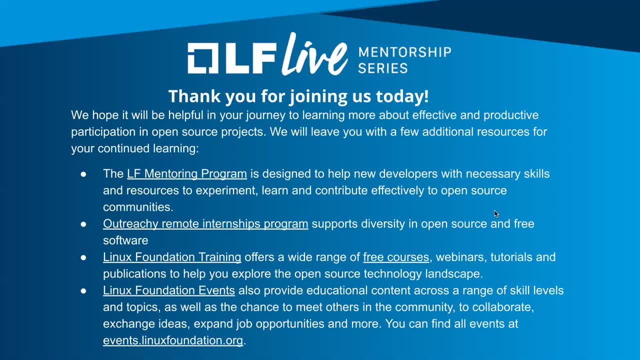 I don't exactly understand that question, So I'll answer what I think you meant and we'll I'll hope I got it All right. Um, you know what this is, something called the free rider problem. Um, but the great thing from the open source software world is that you know what. if somebody wants to reuse, take some open source software and use it and contribute nothing back. 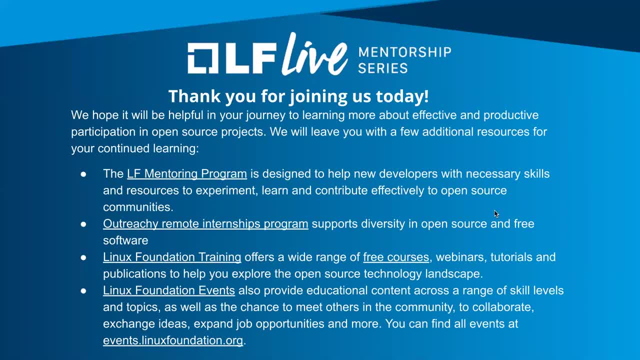 It also costs the open source software project nothing And it turns out that a relatively small percentage- it depends on the software, but typically maybe a percent, 1%, maybe two or three of the of the people who use the software turn around and contribute. 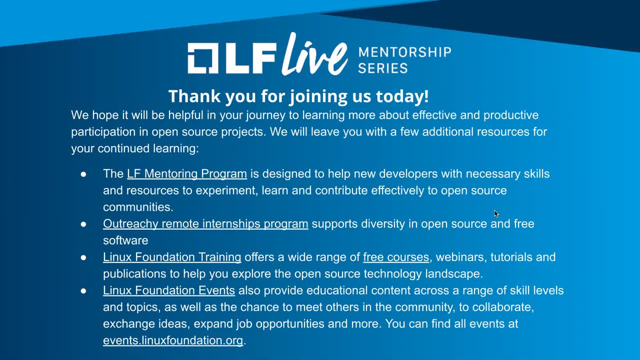 That's okay As long as you have a massive number of users. So if you only have a hundred users and only 1% Are provide any support back, You only got one person who's giving any help. That's a problem. If you have millions of people using that software, this is not a problem. 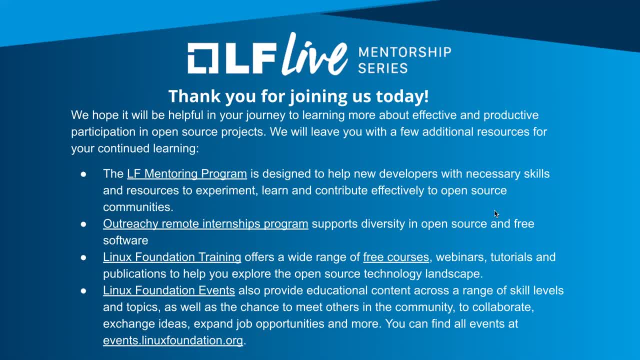 Okay, The, uh, the Linux kernel is available for anybody to use. Not everybody supports back. They literally have thousands of developers and they have an incredible uh release cadence. Uh, same for Kubernetes. Um so um, although it can be a problem as long as you've got a vast number of users. 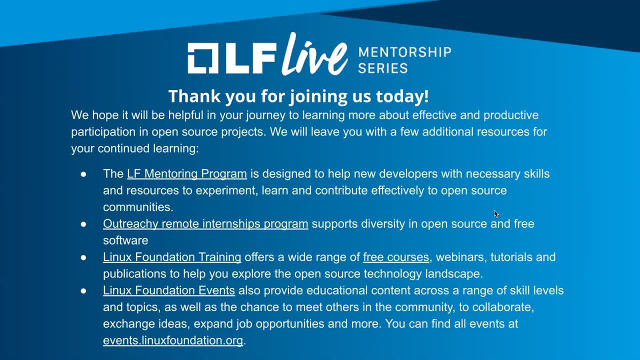 Okay. So the fact that many users don't contribute back is okay, As long as some are willing to work with and contribute back, and, uh, large numbers help a lot there. Um, should we take open source software and do changes for our needs without disclosing to the public? 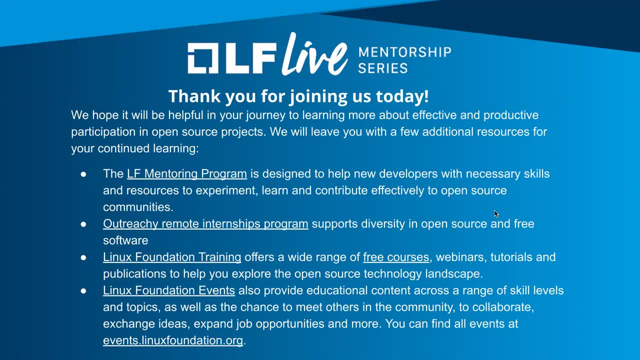 Ah, I kind of covered that earlier. Um, you can do that with any code. Um, believe it or not, you can even do that with GPL code. that is perfectly legal. whether or not it's wise to do that is a different question. 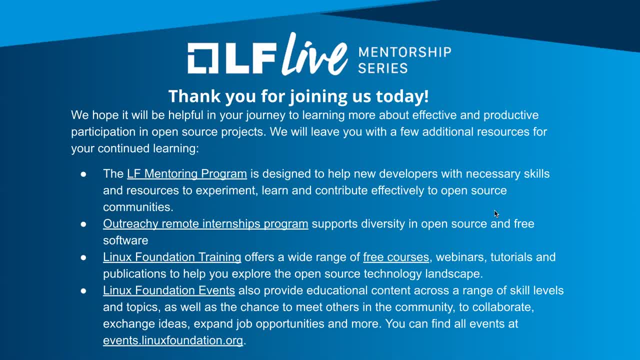 If you are, Needs are So weird and peculiar and no one else is ever likely to do anything like that. Uh, maybe that's fine, Um, but Um, while it's legal to do that, that doesn't make it wise. 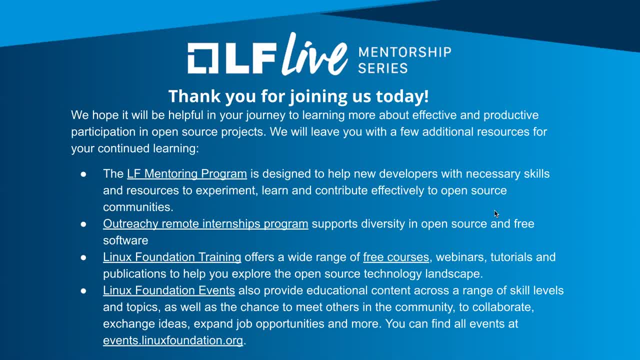 So let's talk about why you would do that. First of all, if you're an academic, you might say: well, I changed the code, but nobody would want to use my ratty code. It's not really intended for production use. 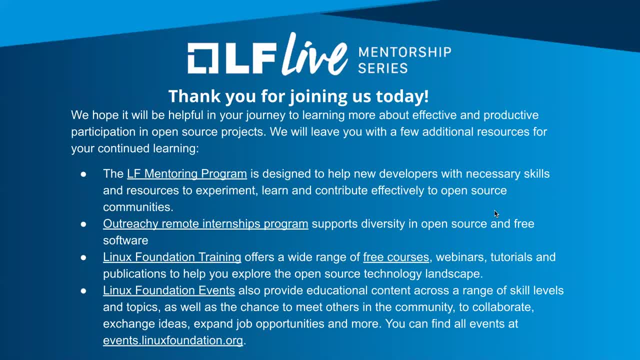 Yes, But you still should release it. Why? Because we have a real problem in science, something called the reproducibility crisis. There's an incredible amount of claims that are claimed to be science, But in fact, when people attempt to reproduce the results, we find out that in fact, they're not true. 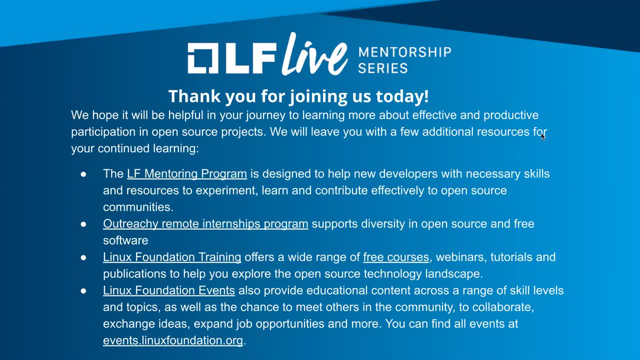 Okay, And that's a big problem in science today- Some areas of science much more than others. Um, so if you're an academic and you want to make a claim and your claim is somehow based on software, You should. You should be releasing that software, not because you think that the rest of the world is going to just use that as production code, but so that you can answer exactly how you got the results. 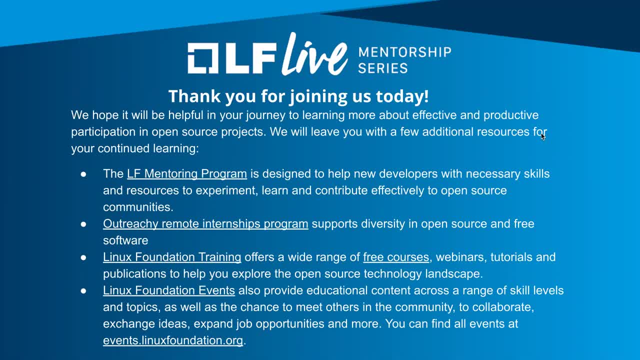 What was your analysis? Um, modern academic papers just don't have the space to record the details that are necessary. Um, and there have been some serious problems. Um, I, there was actually a problem in 2001 where there's a major algorithmic breakthrough. 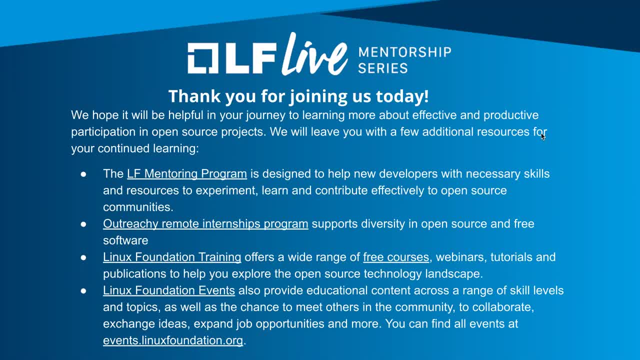 Uh, and something called the sat, uh, the satisfiability problem. Um, but for quite some time, although there was a paper that described this algorithmic breakthrough, no one else could reproduce the results. Finally, the code was made public. 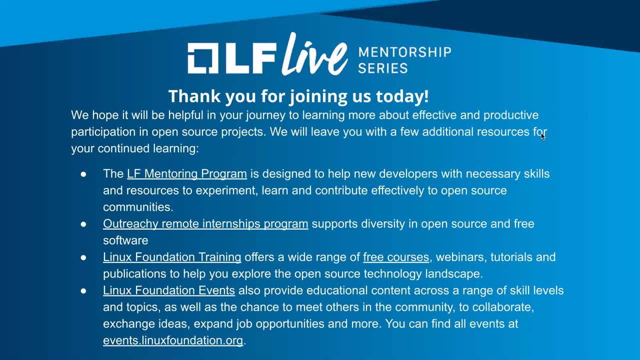 And in fact, in this particular case it turns out that the it was true, but the paper had failed to make some important details clear, And really it's almost inevitable. You just can't make a paper say everything by releasing the code. 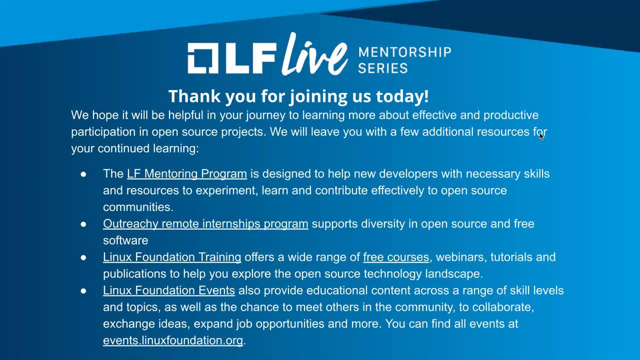 They release it. Now, what happens if it's production code and you're using in yours, in your environment? Well, you can, but if you do that, every time that project makes an update, you're not going to have to figure out how to merge your improvements with theirs. 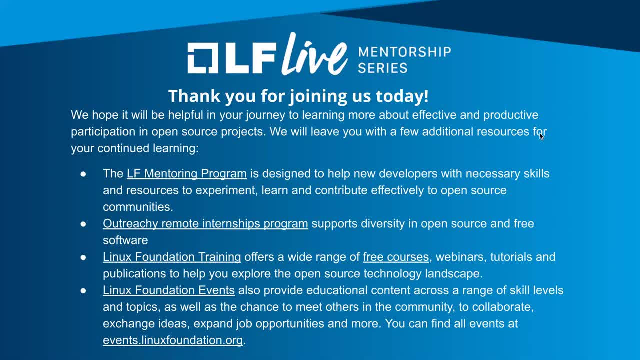 And they didn't make their changes to work with yours because they don't know what yours are. very, very quickly You end up paying an incredible amount of time and effort and money trying to take that code and merge it with the other changes. 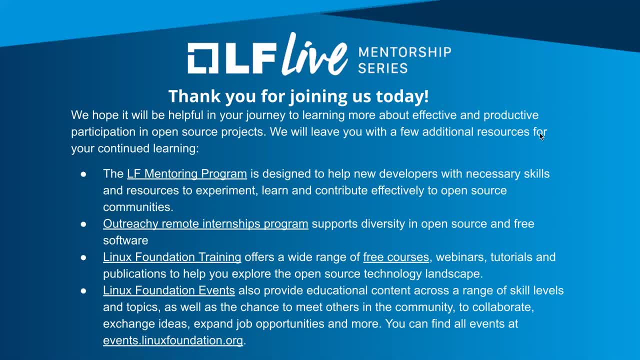 That were made, And the more active that other open source software project is, the harder and more expensive it is um in general, this is a real problem, Whereas if you bring it back you can avoid that 90%. you know that that well- that huge cost of sustainment. 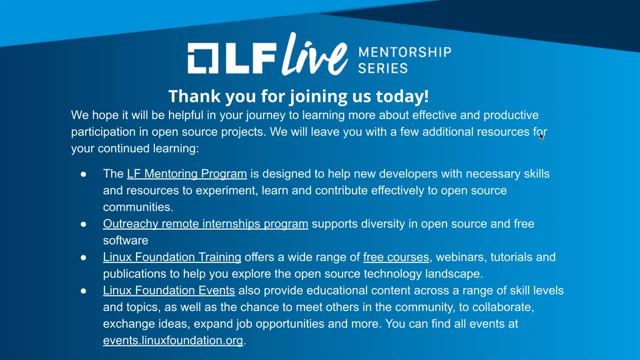 Um, and, of course, once companies start doing that, once individuals start doing that, um, the project starts moving faster. and that becomes even more important for other people to contribute back, to make sure that they're, So that their improvements get in. 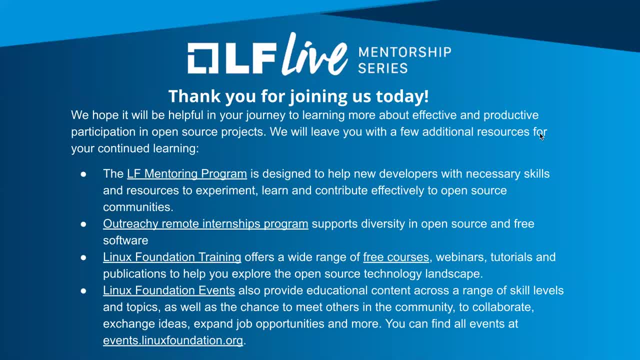 Um, so while it's legal, that doesn't make it wise, and you should be trying to make decisions that are wise, not just legal. Okay, Alrighty, Uh, let's see. here I'm going to go back to the uh, um, uh, to the chat. 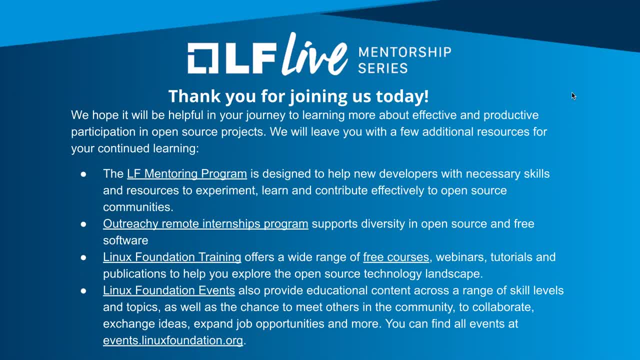 Uh, let's see here. Um, wow, There are a lot of questions here, so let me attempt. I have limited time, but let me try to get to. Um, David, uh, there is one question. really, I think there are a couple of questions. 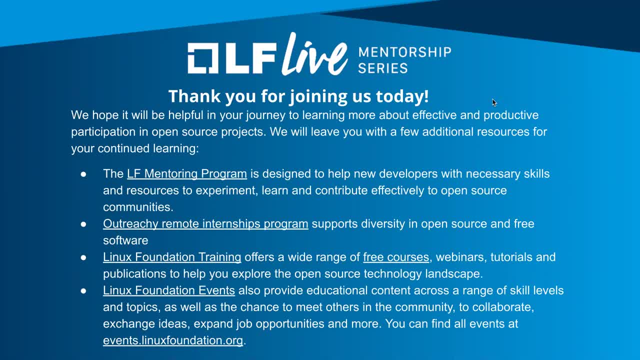 Uh, the rest of them are, uh, thanking you for the presentation. Uh, if I can orient you, there is one question from gosh. Um, okay, CVE, Jason's 5.0 schema. Well, I don't know who the we is. 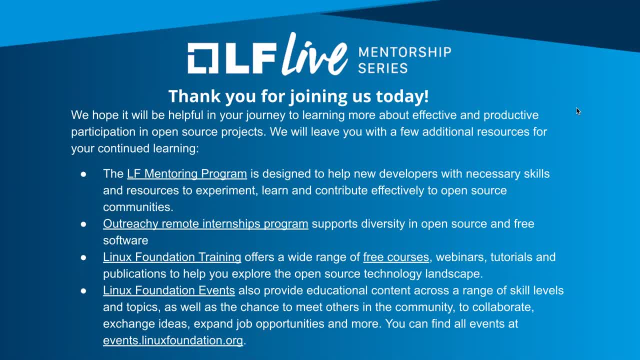 Um, I mean okay, but I mean the CV process does a project, Yeah, The process Community, whatever, Um, you know th there is, of course, uh, Jason 5.0, but we need more than that. 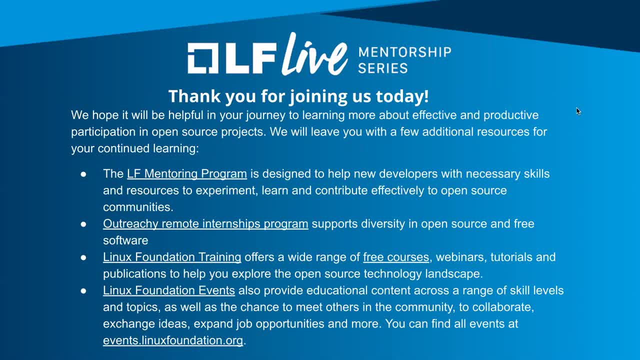 We need to do a better job of com of connecting the CVE reports to uh the software that's vulnerable, so that that can be determined completely automatically in almost all cases. Um, so I mean, yes, there's there's uh various improvements as they update their Jason, but in my mind that's the more. 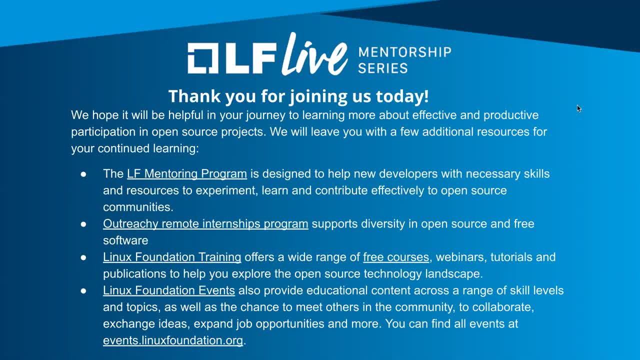 More important question: Um, so, yeah, see, assumes the developers can tell us Richie. well, and to be fair, the problems that they had at the time were quite different. Um, you know, they were trying to make very limited equipment do a whole lot. 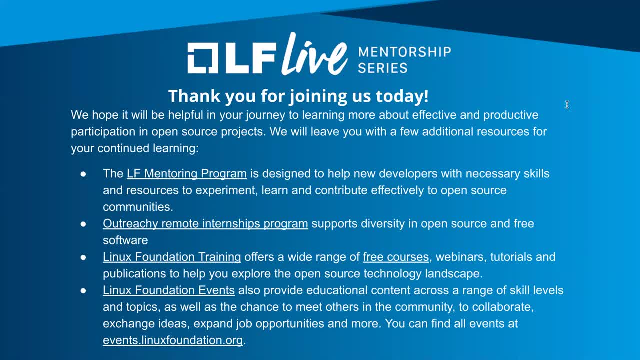 Um, you know, modern phones are thousands of times faster, thousands, probably millions of times faster. you know, thousands of times faster, a thousand times more memory, than the equipment that they were working with initially. So, Um, you know, different circumstances, uh, different problems. 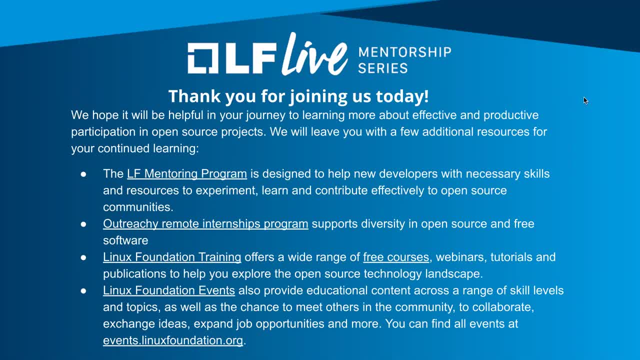 Um, let's see here. Yes, the slides will become available. Um, okay, No matter the language, we do see plenty more vulnerabilities in the application stack, where the lower stack, all the system that might have blast radius. Um, I think that's kind of oversimplifying, but there's some truth to it. 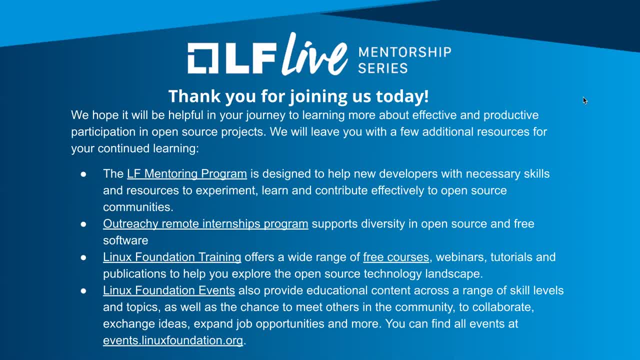 I think the re- I would characterize it slightly differently, Although Maybe it's a subtle distinction- Um, the system tier because that's used by so many different, completely different applications. um gets a lot of focus from a lot of different folks. 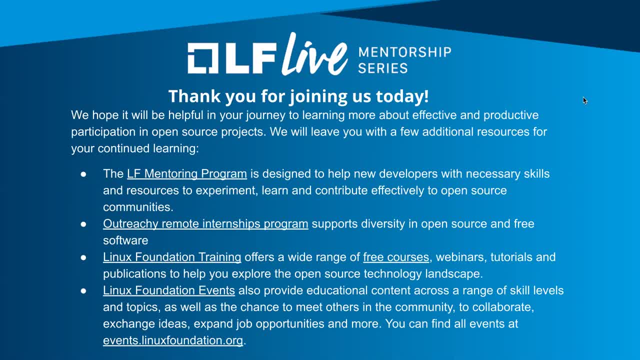 And so, um uh, a number of vulnerabilities get squished out from a number of the system tier components, simple because there's more people using them than any one specific application stack, Um, and of course, a lot of the application stack stuff moves. 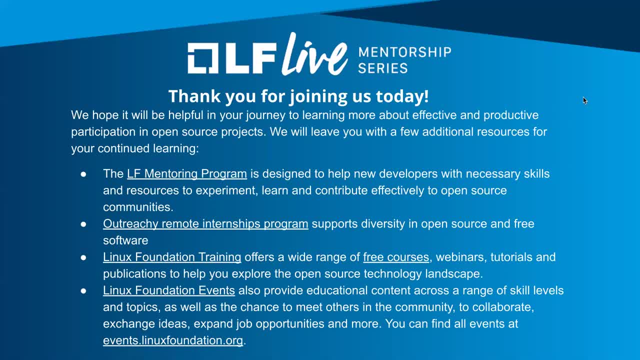 Uh is uh faster moving and changing, And when you make a lot of changes in a hurry, you're more likely to make mistakes. I mean, that's true for software, It's just for anything else, Uh. but I think the reality is that we need to worry about security at all layers. 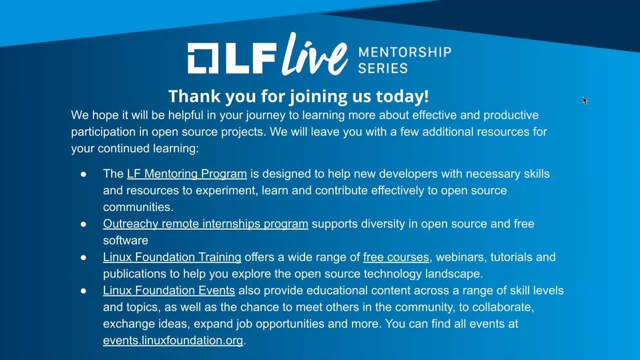 Okay, And there are basic, fundamental principles that apply no matter what you need to know. I mean, it's true that, for example, I mentioned memory safety. for many, many languages, you know their solution is: use a language that provides memory safety. 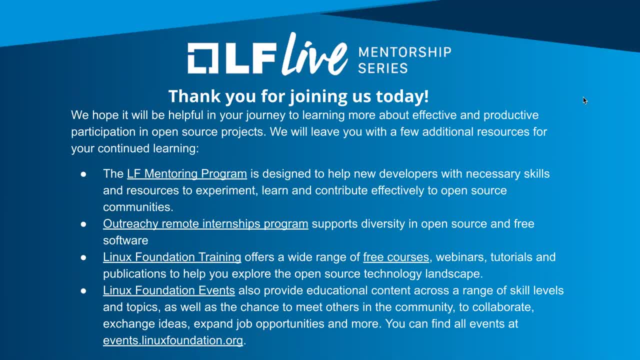 You're done. Uh, for some folks, though, you usually use a memory, a language. that's usually memory safe, but you can disable them, limit when you disable them And when you do. now you got to apply that knowledge that's specific to memory safety issues, because in the unsafe parts it's um. you have to apply that. 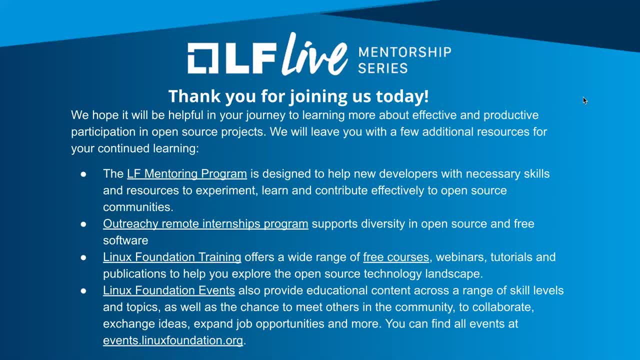 Of course, if you're programming in CNC plus, plus, uh, there is no safety, It's always unsafe And therefore, um, you have to write with extra care to make sure you don't have any of those problems. But you know, a vast amount of the stuff is just 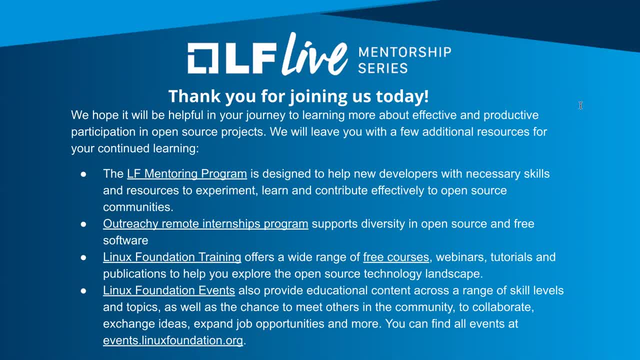 That's would be great, But you know, I mean you've got to be able to think about where the bad stuff of the knowledge is and, uh, what's going to work on where the bad stuff, uh, is going to work on. 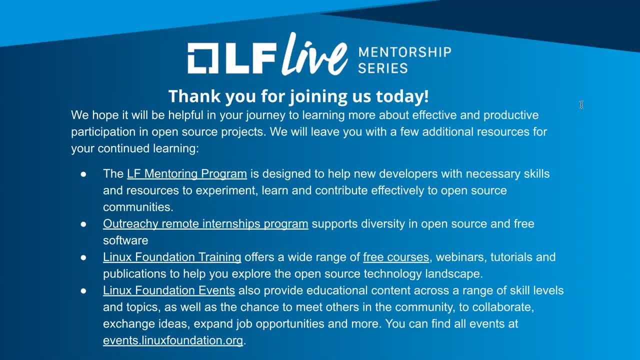 Uh, the people who write the code. that are the people who write the code. all the rest don't depend on you. know, like any other infrastructure, I'm always, I am, grateful to those many unsung heroes who make our roads. 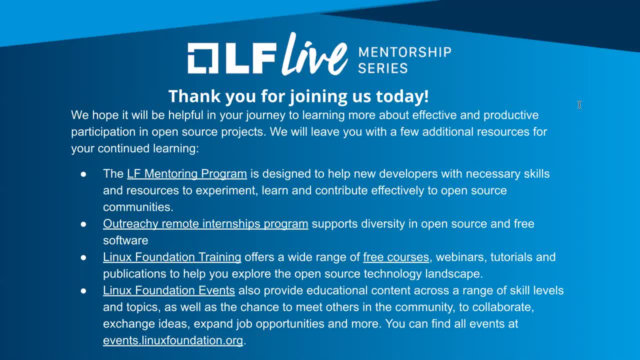 Uh, you know, build the bu, build our buildings and, oh yes, Write the software that we all depend on. So I'm grateful to all of them, including, Uh, you know, Including many, many of you who develop the software that the rest of us depend on. But please, please, there's some- I've tried to kind of give that surface. take a course- I pointed to a free one. you know, learn a little bit. 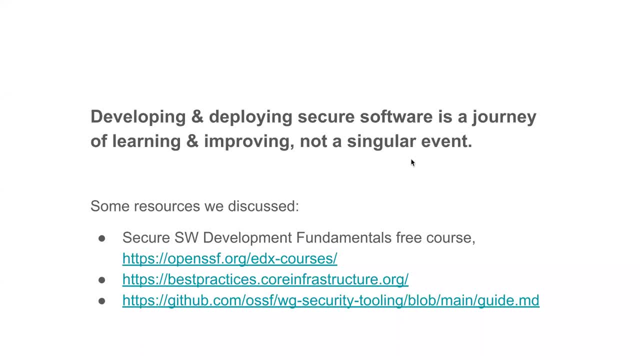 You know if you're doing, if you're managing or involved in open source projects. try to get badges, get some tools into your CI pipeline. While it doesn't guarantee those things- don't guarantee everything- they really make a tremendous difference. 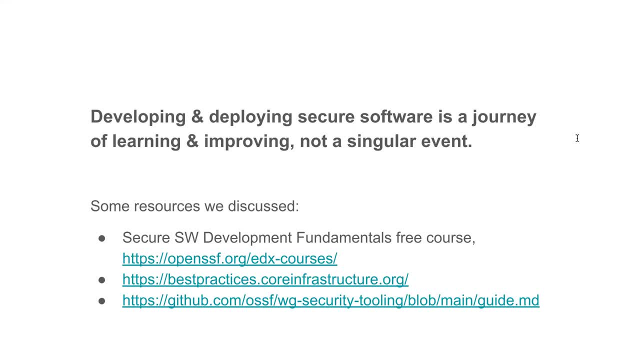 All right, Wow, I'm out of. am I out of questions? I can't believe that Surely people have some more questions for me, Because I do want to answer questions is kind of the point of this. Yeah, Yeah, you probably have time for maybe one or two more more questions. 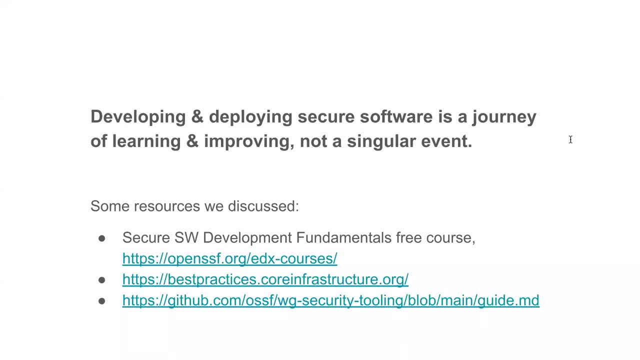 One or two more questions, All right. So somebody quickly type in a question, So we will. I can't believe I managed to get through them all. There were some interesting. there were a number of interesting questions here. Okay, I had. when I was creating this presentation I had originally thought about diving in, for example, 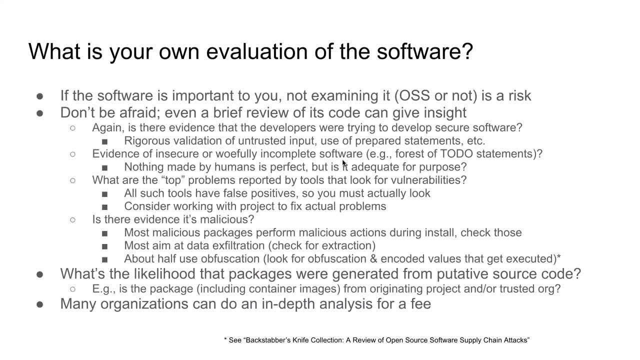 I had. when I was creating this presentation, I had originally thought about diving in, for example I had. when I was creating this presentation, I had initially thought about diving in, for example, into the many different common kinds of vulnerabilities. 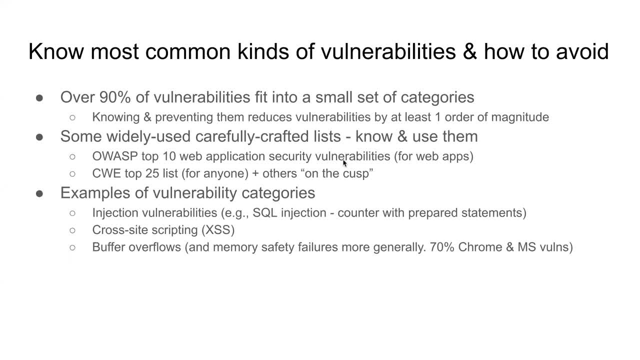 You know I mentioned right here, But I decided not to. There is always a danger, first of all, that thinking that if you know the most common kinds, you know all there is to know about security, and that's not true. 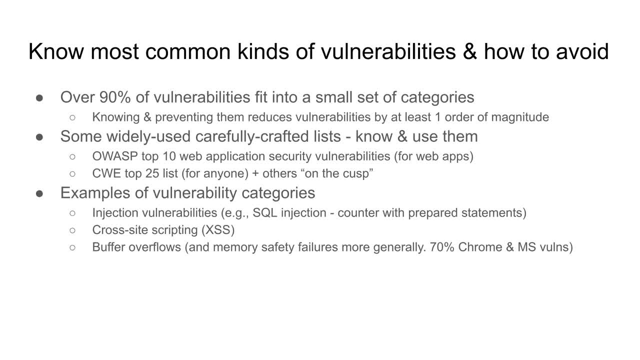 But in 45 minutes I just wouldn't have had time to get in enough. It's not that I need a lot of time, It's just 45 minutes isn't quite enough. And so you know, what I really want you to do instead is point you to these top lists, point you to courses like the one I just mentioned, that kind of walk through. what are the top ones? how do you counter them? but you know, counter them in terms of things, like you know, write code this way instead of that way, or use this kind of approach instead of that kind of approach. 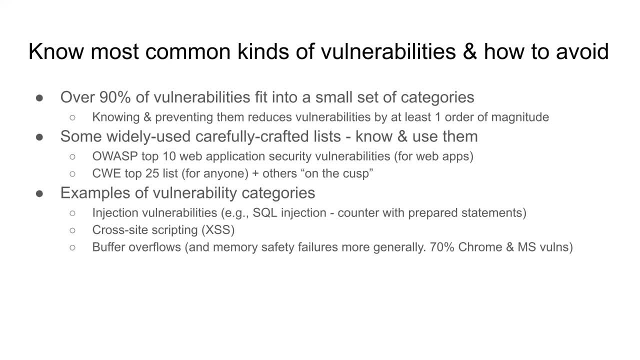 None of them are terribly complex mentally, particularly if you're just worried on what am I trying to avoid and how do I fix it. I mean, you don't need to know the details of memory management to know how to avoid buffer overflows. 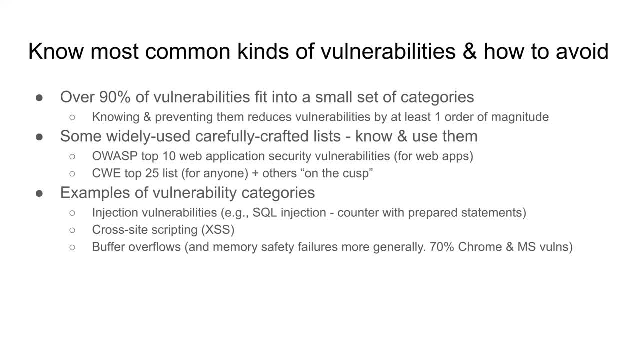 You know, don't try to read and write out of the buffers, usually arrays that you're supposed to be using. Check, make sure that you're within them. It's not complicated, at least mentally. It can be complicated to do because you have to keep doing it over and over again. 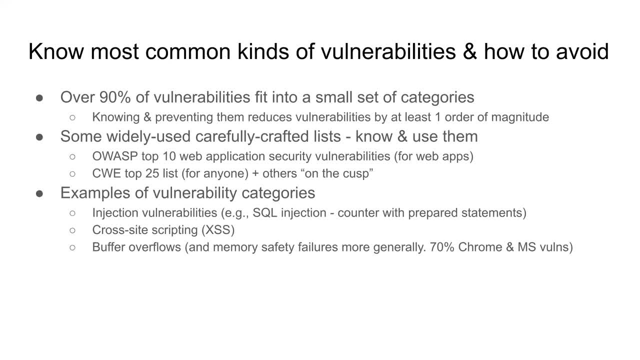 But if you're using C or C++ or any other unsafe concert, that's what you're paying for. You know you are getting all the control, But now you have to take responsibility for the awesome level of control you receive. If that's not, if you're not comfortable with that, if that's not what you wanted, maybe these were not the right design decisions for what you have planned. 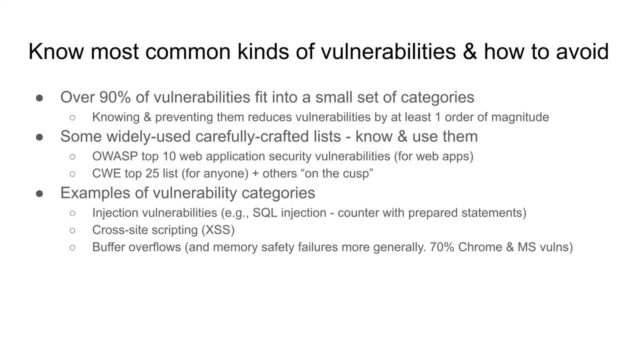 If you see what tools or guidelines exist to assist GBD, et cetera. Well, in fact, I've already gone through a number of those. There are a number of guidelines. I talked through the course. There's a number. 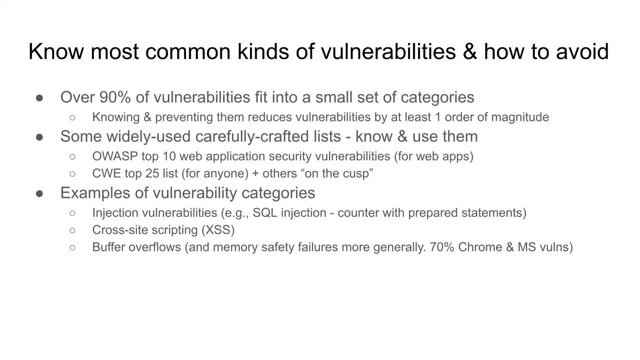 It lists a number. There's a number of common vulnerabilities When I talk. in the course itself, it mentions specific things. So you know, don't for C, don't use strcpy if you don't have to. Using strcpy or s and printf or some other function like that which provides automated protection, is going to basically replace the dangerous ones with the less dangerous ones. 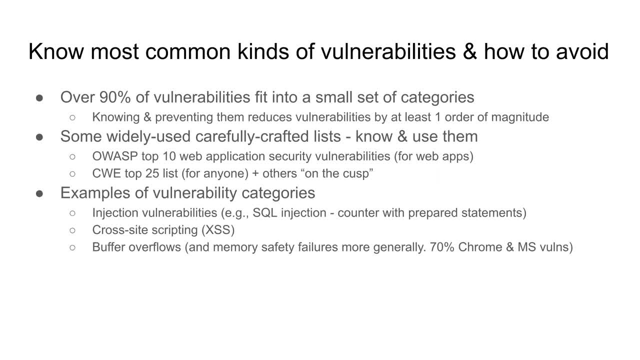 And the course goes through the you know, instead of this function, do this or, you know, consider using this instead. But GDB is not really going to be so much of your friend here. GDB can help you find if you have a particular input. that you know is a problem, but the challenge is finding the inputs. 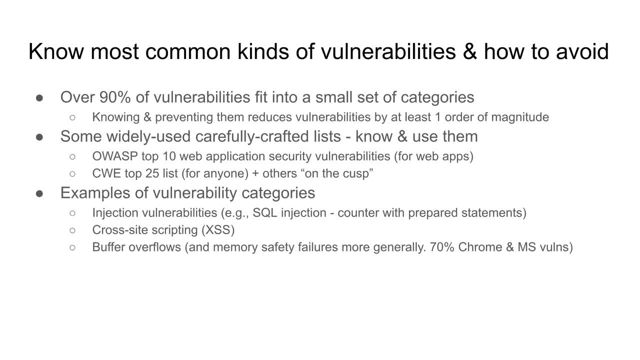 Fuzzers can sometimes help you find inputs that will cause trouble. In which case, once if you use a fuzzer and it finds a vulnerability, then yeah, you could use GDB to help you find those, But it's much better to know ahead of time where the common problems. you know what kinds of function calls. 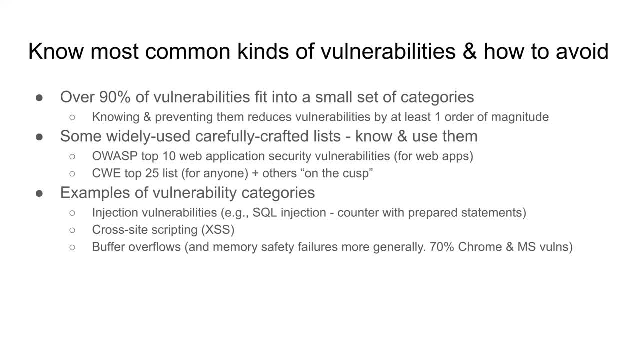 What approaches should I use instead? And then using tools to detect problems and fixing those remaining problems is really the way to go if you're using C- And I use C a lot myself, So it's not like you can't write secure software in C. 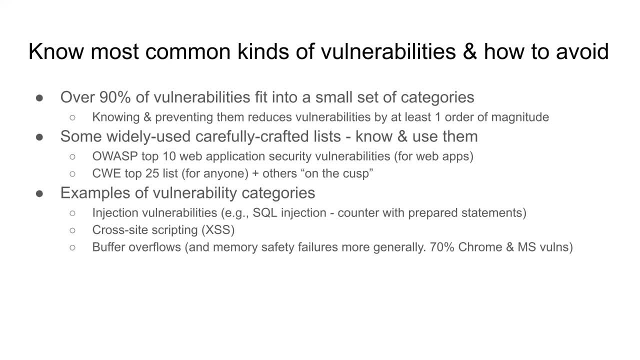 You just got to be stinking careful. If you're writing in C, also go read the standards. If you have not read the standard, in particular the appendix on undefined behavior, you got to do it. There's a lot of things that are undefined. 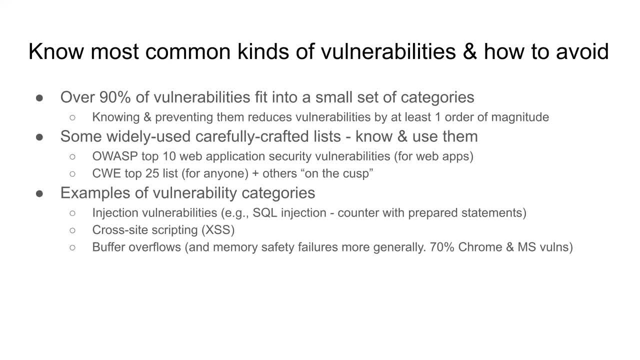 That a lot of people who write in C have no idea and they're just basically foot guns waiting for you. So hopefully that answers that question. David, GCC seem to be including some of the CWU detection lately with their FNLizer option that I'm finding useful to run through. 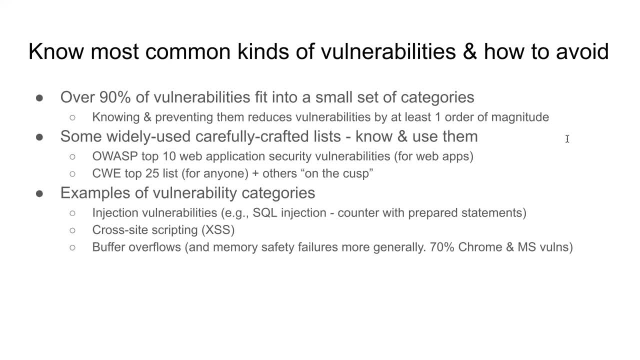 Right now, as far as I'm concerned, it's just GCC, and CLANG also has some tool, you know, using GCC and CLANG to detect some vulnerabilities. Right, It's a tool. It's just like your other tools. Turn on as many as you can. 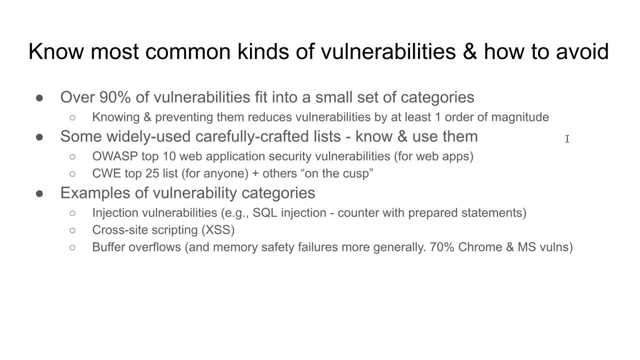 By all means turn on the mechanisms in GCC to detect vulnerabilities. On the other hand, don't expect that GCC or CLANG or any other tool will find all the vulnerabilities. You want to learn how to avoid them in the first place, and then you want to use tools to help you find the ones that got through. 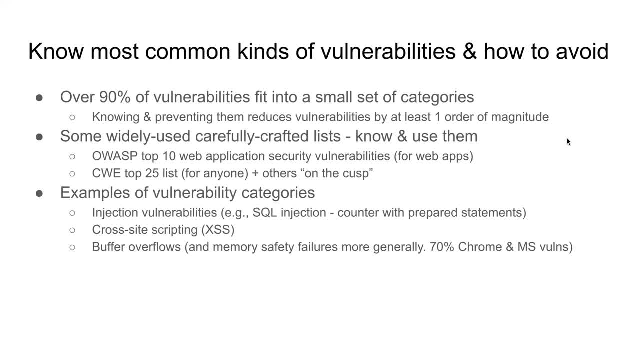 Right, Absolutely. Thank you Very good. Very good, I'm done. Yes, you did it. We are right at time everyone. Big thank you to David and to Shua for their time today and thank you all for participating and asking questions. 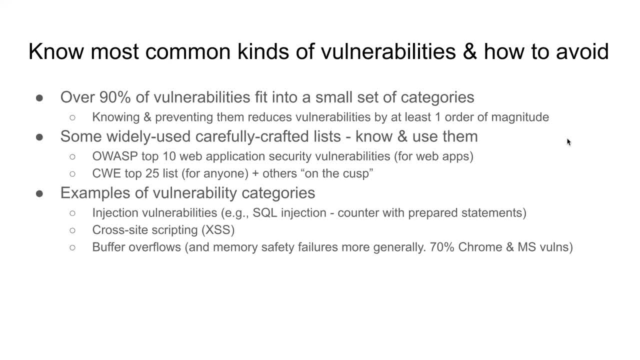 As a reminder, this recording will be on the Lenox Foundation YouTube page later today and a copy of the presentation slides will be added to the Lenox Foundation website. We hope you all join us for some future mentorship sessions, and that's a wrap. 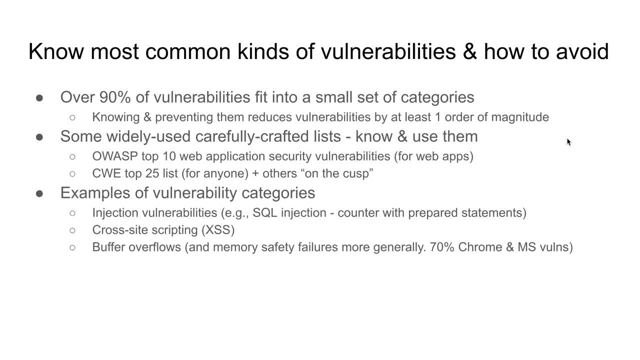 Have a wonderful day everybody. Thank you so much, everyone.